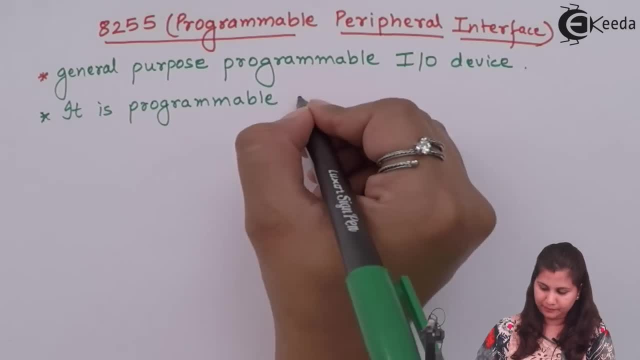 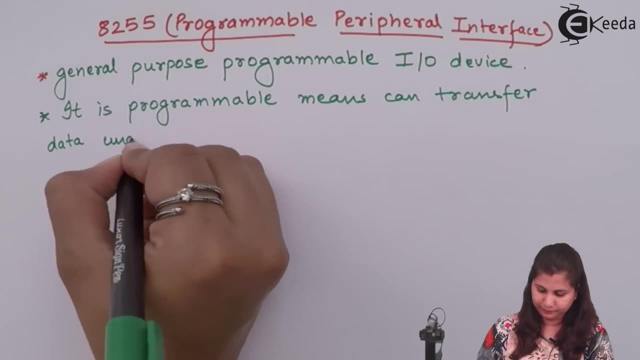 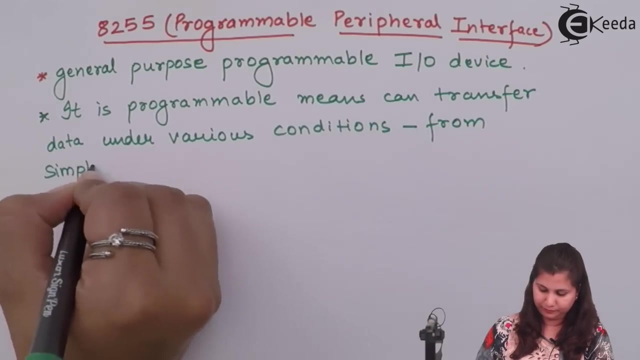 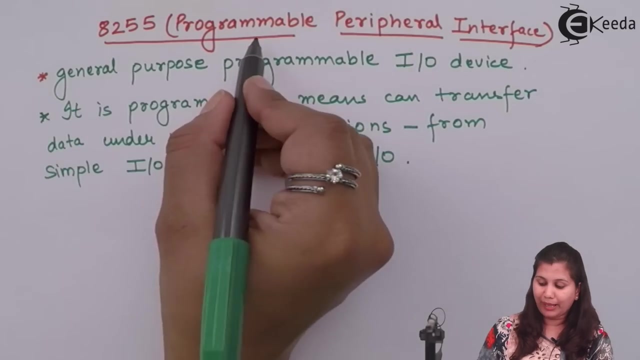 Go ahead and try out this 8255 and peripheral interface, This 05308, and the IC number is 8255, but that is aициаровize interface and the Department is capable of all these functions. So it is said to be programmable. peripheral interface. Now you can see it is 3D processing and an image processing. So let's go ahead and analyze the 8255, it is a general purpose programmable interface which can be programmed. So this 8255 and the IC number is a general purpose programmable input output device and the other devices. 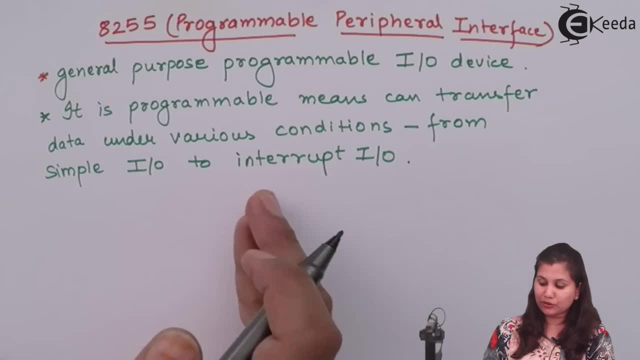 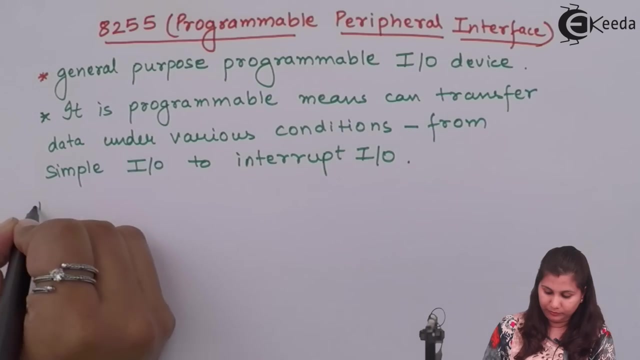 that it can transfer the data under various types of conditions, like from simple input output device to the interrupt input output device. It means it is acting as an communication path between the processors, microprocessors, so that they can have interaction with each other. Okay, Now this 8255 microprocessor. it is very flexible, it is versatile and it's 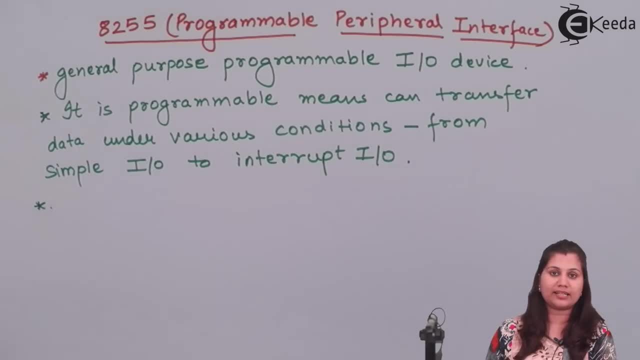 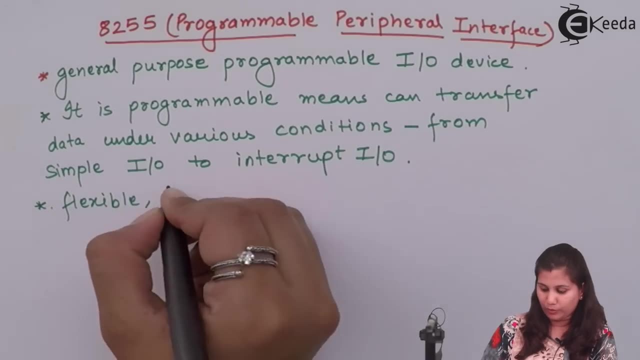 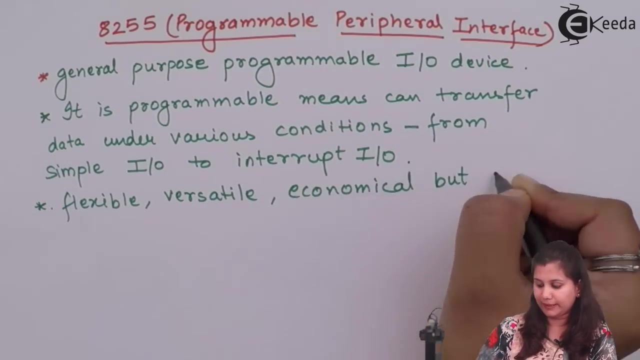 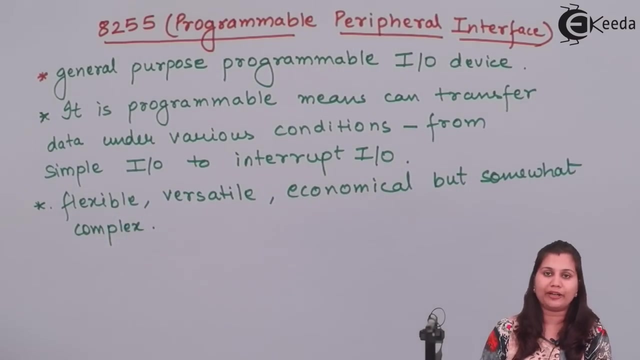 very economical but its circuitry is somewhat complex. So we can say that 8255, it is flexible, versatile, economical but somewhat complex. So these were little bit features of the 8255 microprocessor, this 8255 programmable peripheral interface. Now let's see that. what are the features of this? 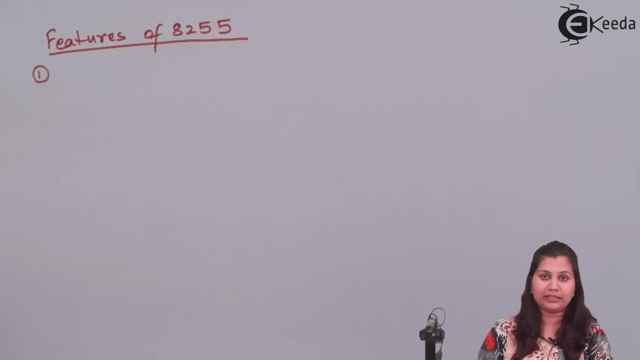 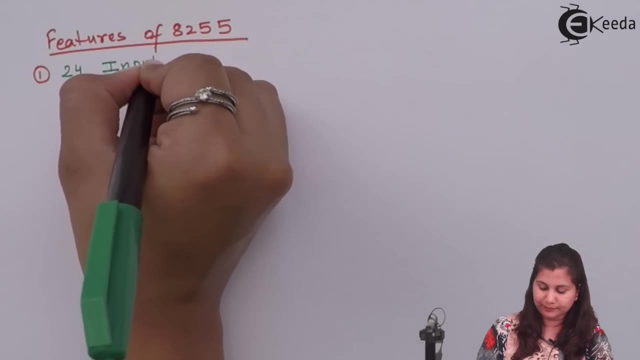 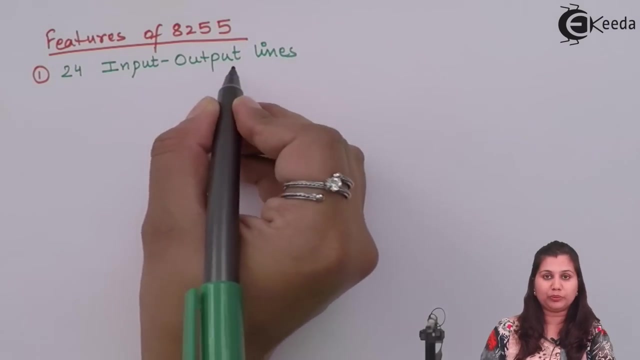 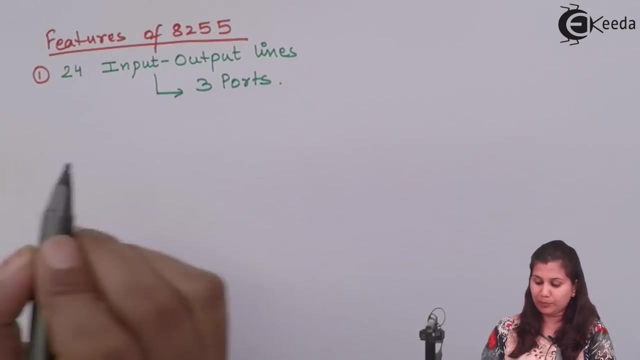 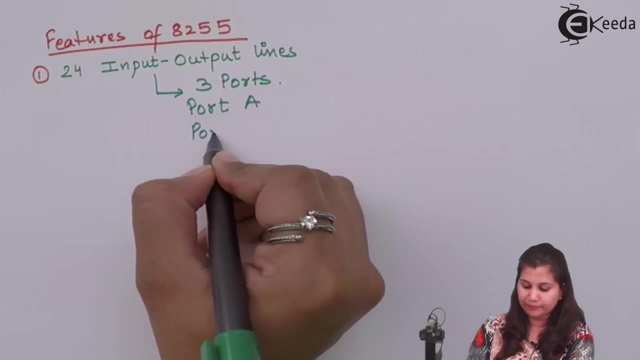 This 8255 programmable peripheral interface PPIA. it has 20 4 input output lines. and these 24 input output lines, they are divided into 3 ports. Okay, These ports are input output ports and they are named as port A, port B and port C. 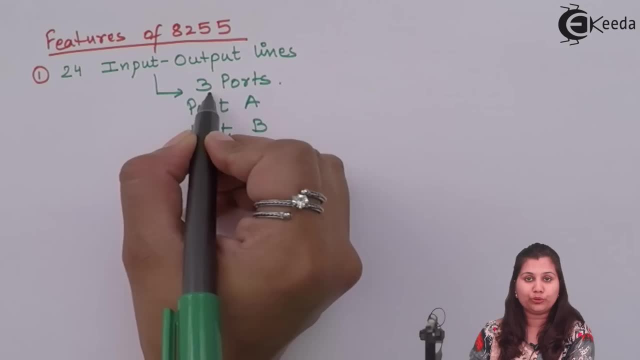 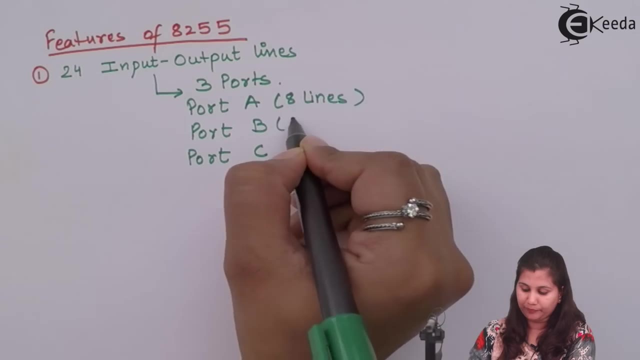 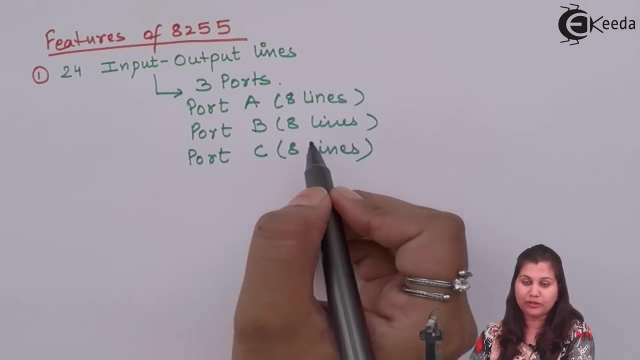 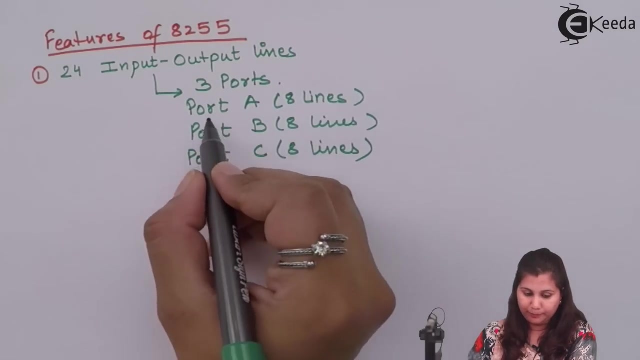 So 24 input output lines divided into 3 input output ports. So each port will have eight lines And these lines can be used as either input lines or the output lines. okay, Now the port A and port B. they have one 8 bit output and one 8 bit input and one output. okay. 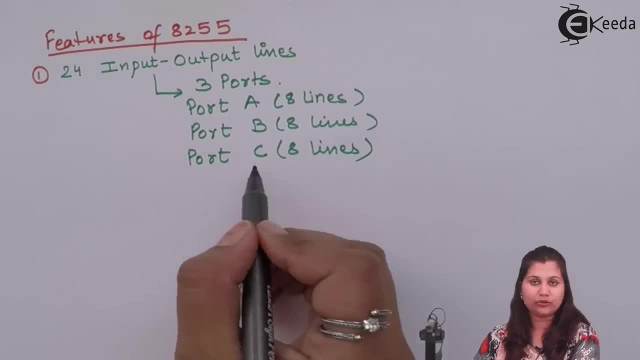 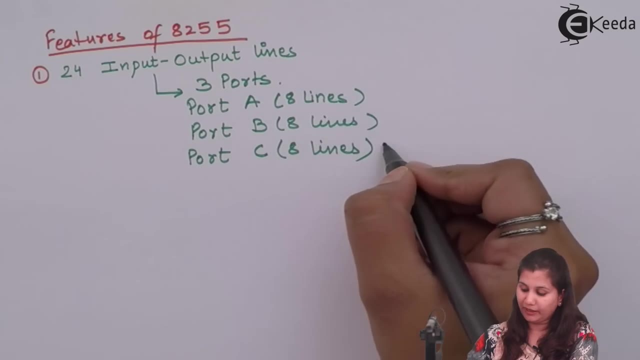 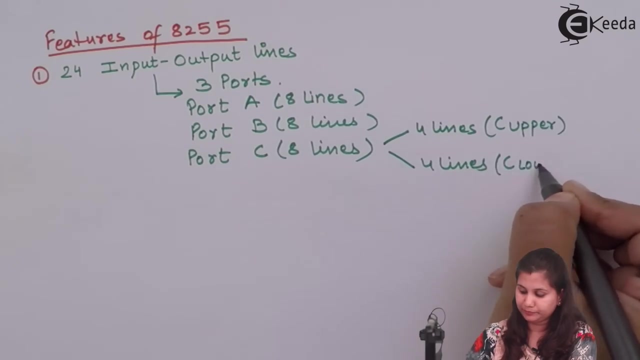 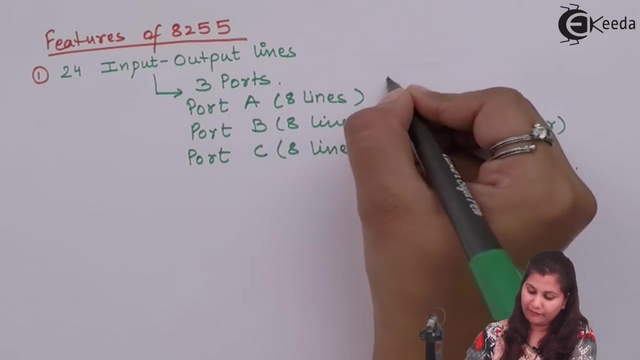 input buffer associated with it, whereas port C don't have any buffer associated with it. also, the eight lines of this port C, they can be divided into four lines, so four lines. they are known as the C upper and C lower. so if we denote the eight, eighth lines of all these four ports, then for port A we will have A. 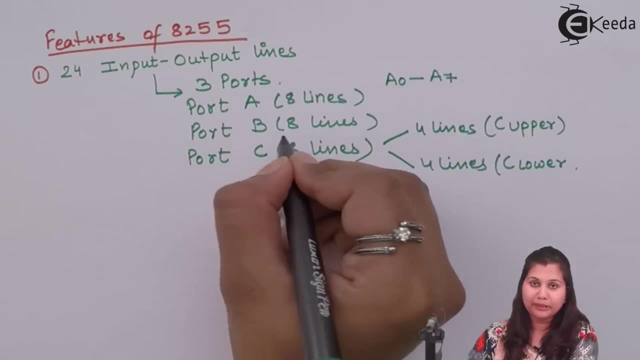 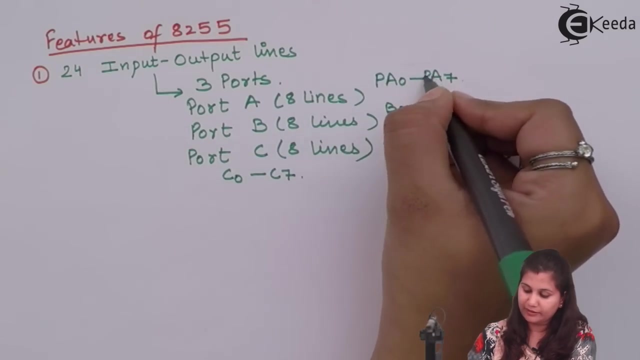 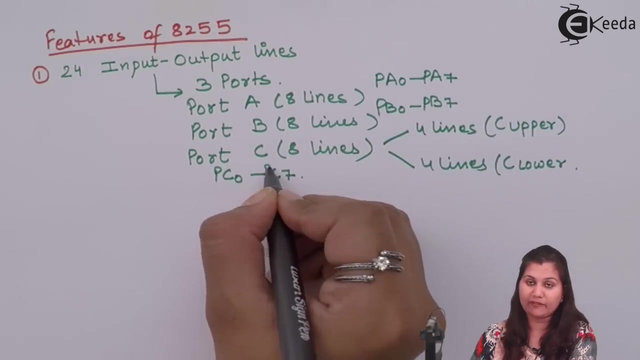 not to A 7. for port B, we will have B, not to be B7, and for port C, we will have C, not 2 C 7. okay, now, this is these are the ports, so it's suffix. we we are writing here as P A, not P A seven. then B B, not P B 7, and P C, not your PC, Mehran'. 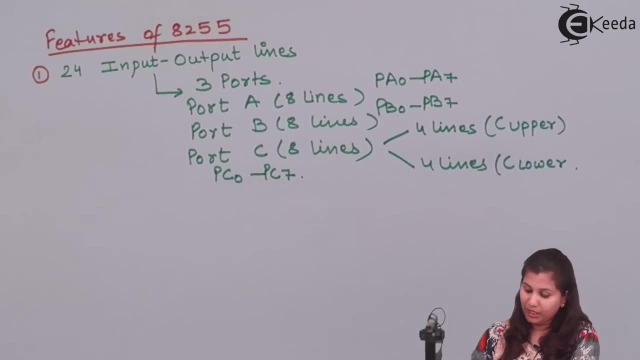 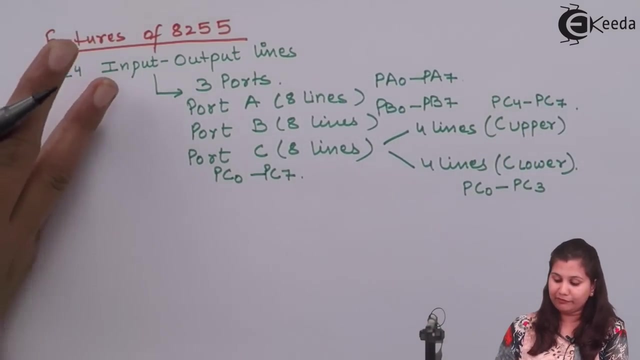 two things denote that these are the ports. okay now, pc, not pc7. they are, uh, these eight lines. they are further divided into four, four lines, so c upper and c lower. we will have pc naught to pc3 and pc4 to pc7. so we have the 8255. we have 24 input output lines, which are divided into three ports. 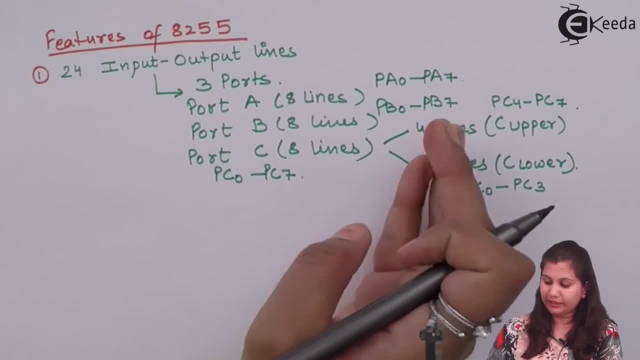 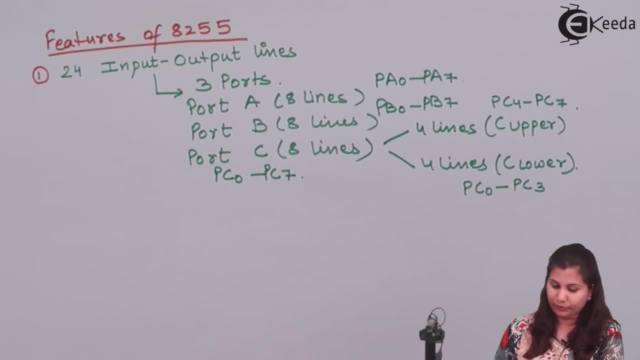 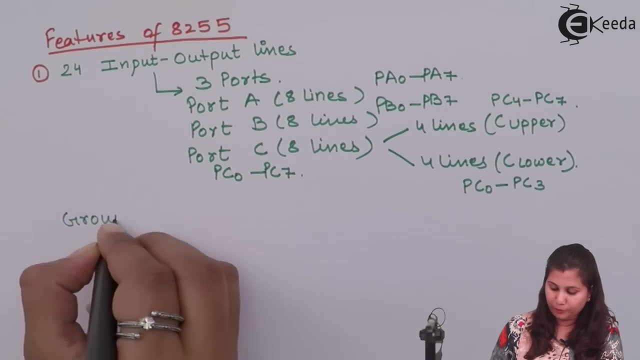 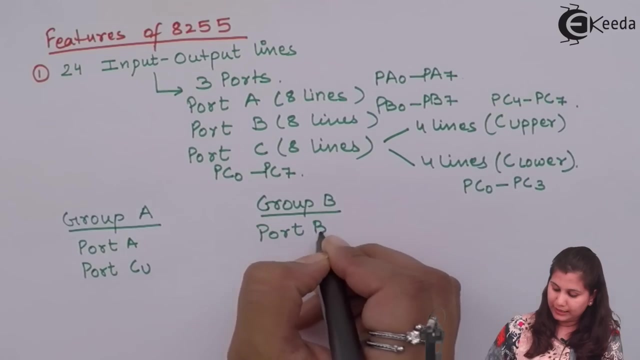 port a, b and c and port c is further divided into two, four ports, uh, four lines, ports which are c upper and c lower. okay, now these ports, they are grouped into two: group a and group b. group a has port a and c upper, and group b has port b and port c lower. okay, so port a, it has eight lines, then it has four lines. 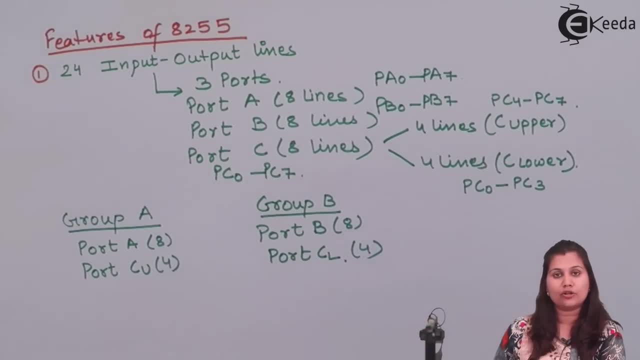 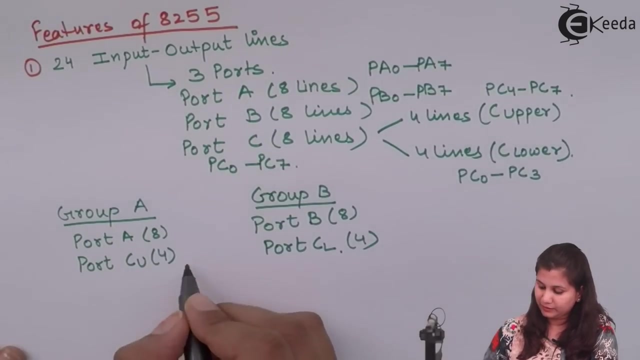 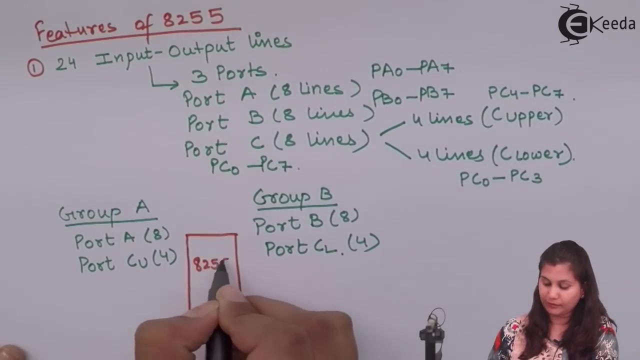 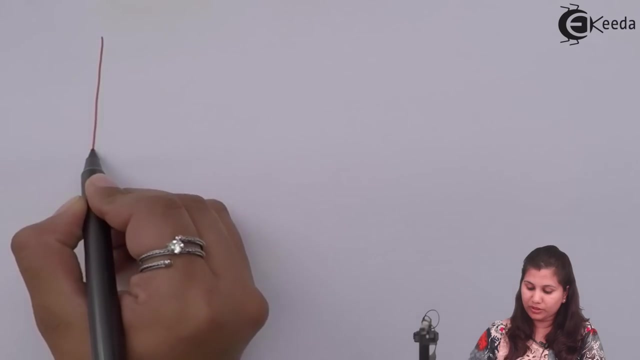 it also has eight lines and these are the four lines, so 12, 12 lines are available in each of the groups, group a and group b. if we draw the diagram here for it, then it will be like we have the 8255, let's draw it here. so if we draw the diagram for it, the ports how we can. 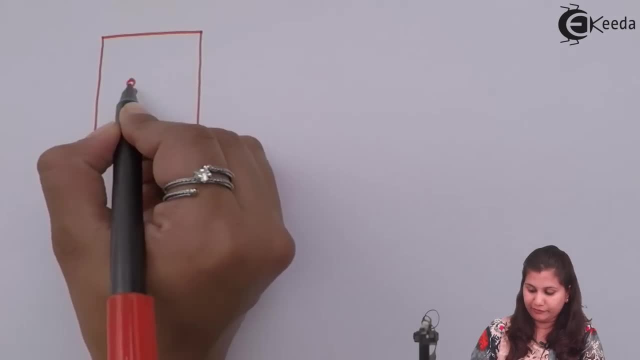 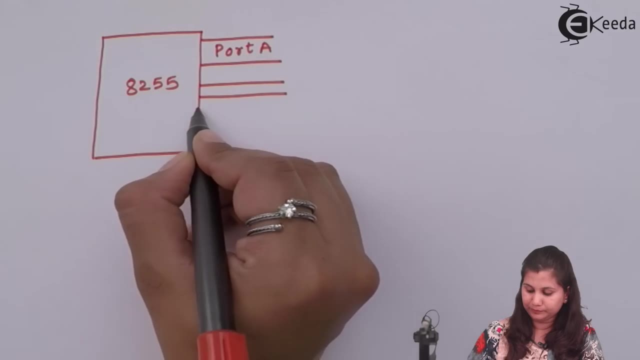 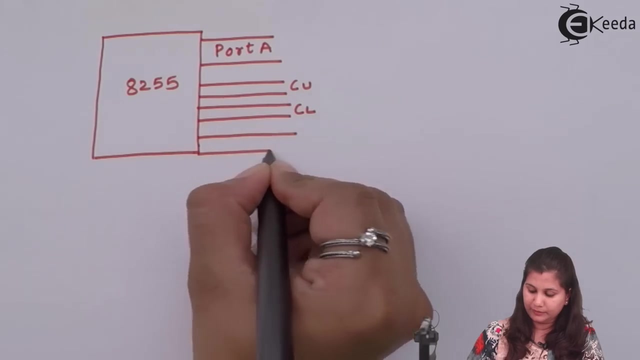 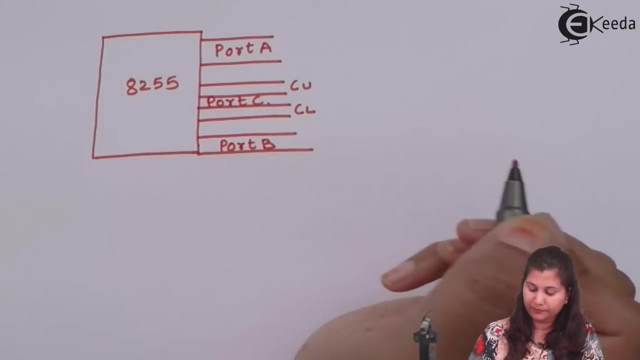 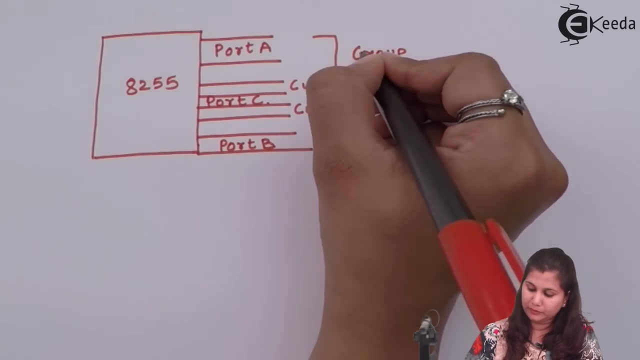 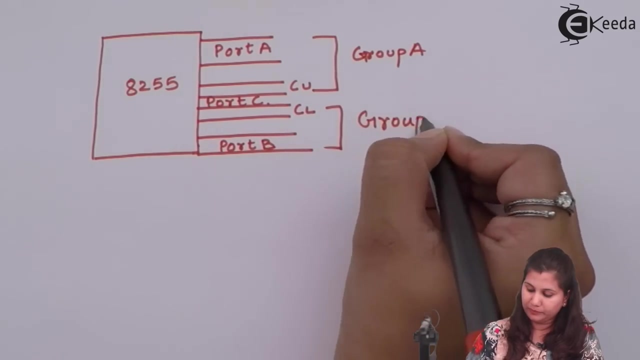 describe it. we will have 8255. port a, this is c upper, c lower, and then port b, this is port c. okay, so port a and c upper, they are forming the group group a, and c lower, and port b, they are forming the group b. okay, now these uh ports, they can be. 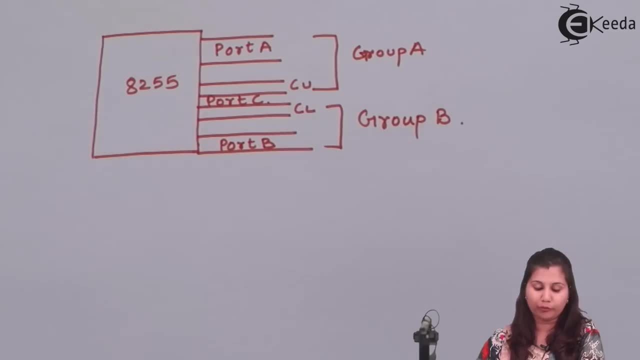 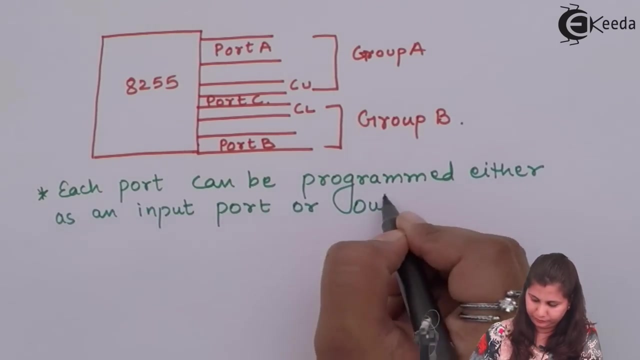 programmed either as an input port or either as a output port. so they can be programmed either as an input port or as an output port, and this description that how we are using the ports, whether as an input or output port. it is decided by the modes of the. 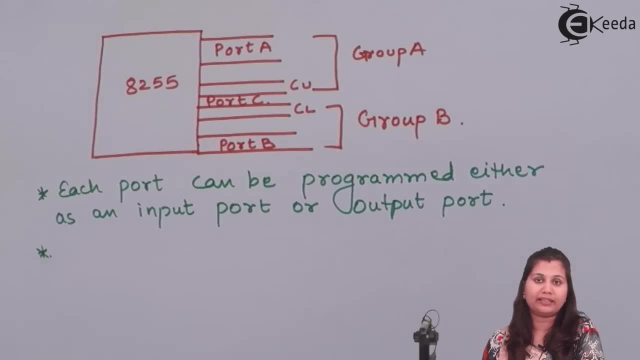 8255. there are different types of modes, so those modes define that which port will be used as an input port and which port will be used as an output port. so so groups, so the two groups of the ports, group a and b, it can be programmed in different modes. 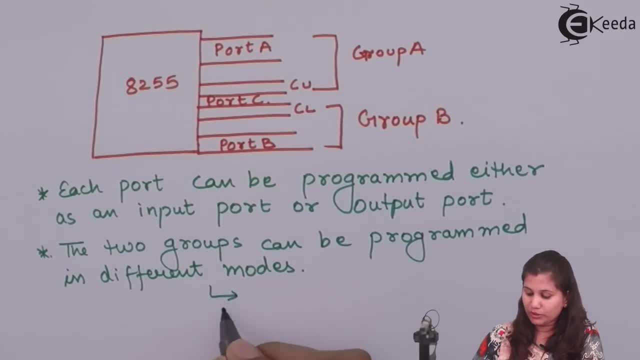 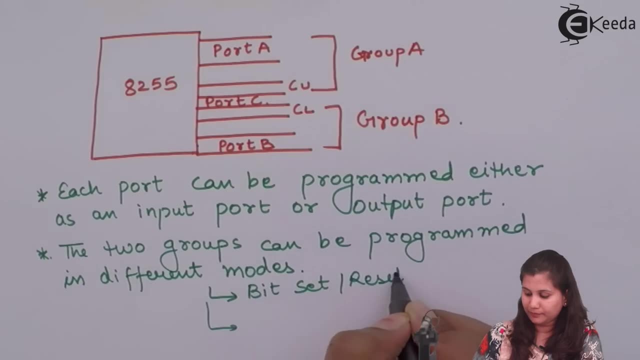 and in 8255 we have two modes: bit reset mode, the other is input output mode. so there are two modes: bit set reset mode and input output mode. this mode- bit set reset mode- it decides that which bits are to be set and which are to be reset, whereas the input output mode it will. 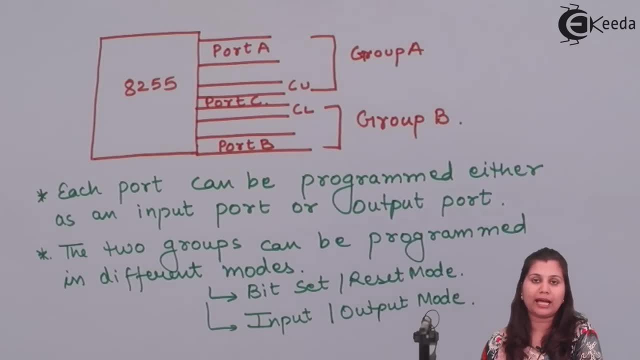 decide that which port is going to be used as an input port and which port is going to be used as an output port and the input output mode. it is further divided into three modes: mode 0, 1 & 2. so input output mode. we have mode 0, 1 & 2. we 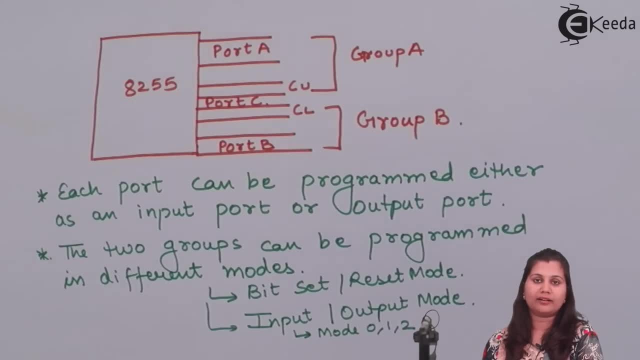 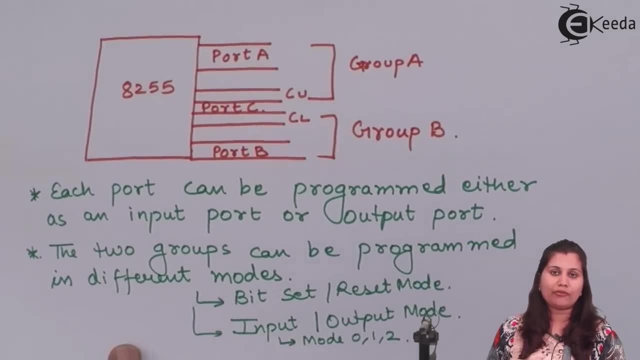 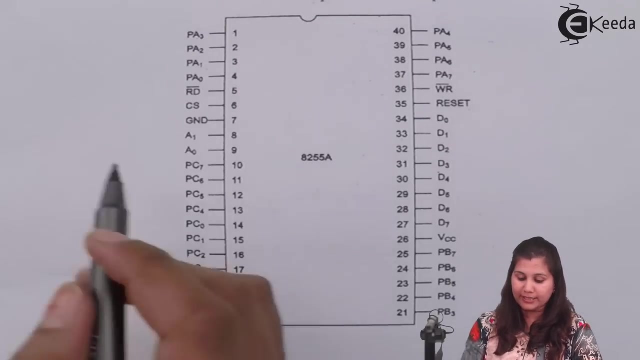 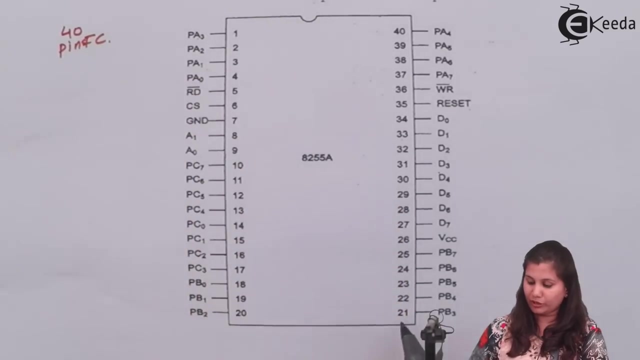 are going to study these modes of 8255 in our other video. okay, so now let's come to the pin diagram of 8255. we have the diagram for the pin description because it's a 40 pin IC, so these are the 40 pins denoting all the pin names are written over here. now, if 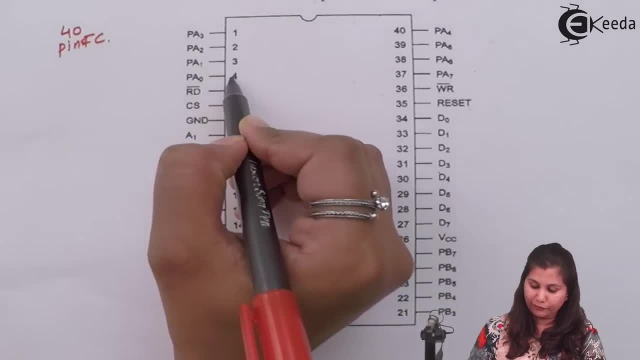 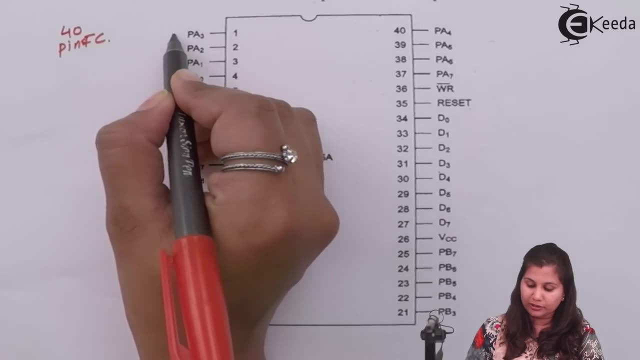 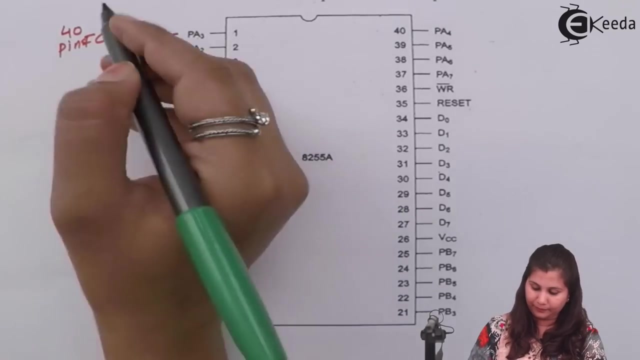 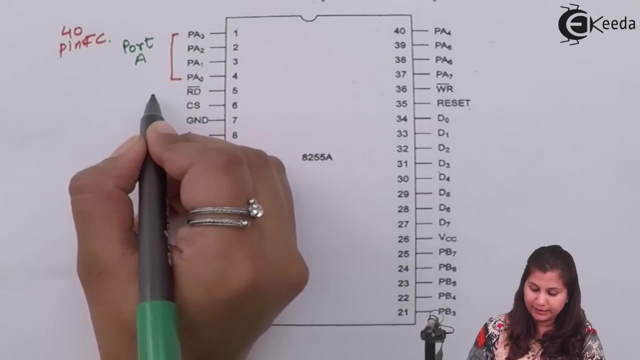 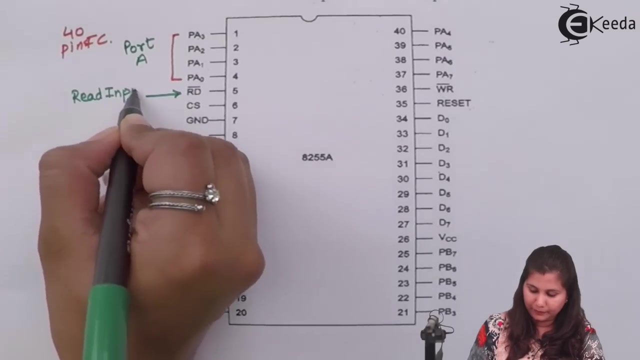 you can see that this pin number 1, 2, 3, 4. they are denoted as PA 3, PA 2, PA 1 and PA not. so these are the four lines of the port a. then we have our D bar. this is the read input. then CS, it is chip select. 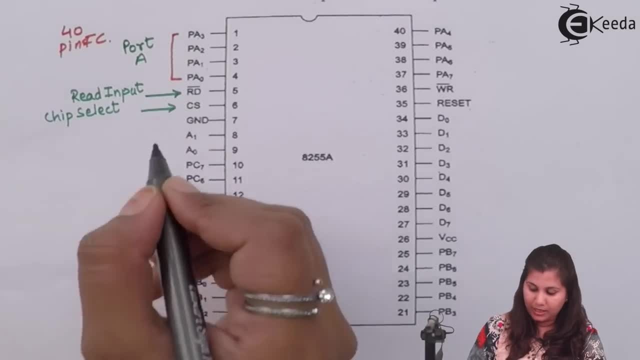 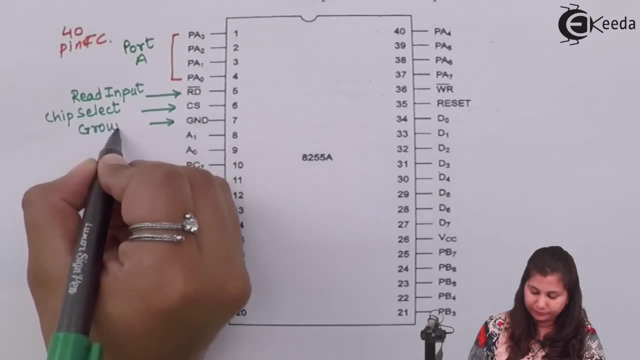 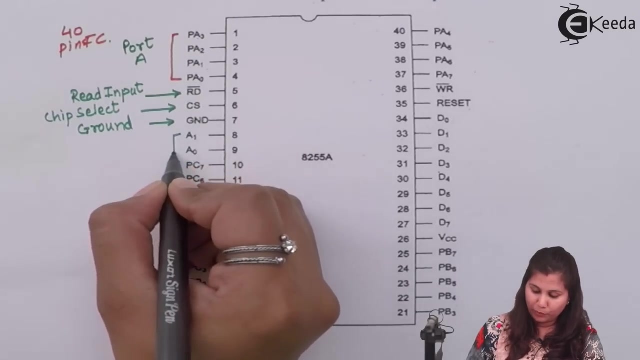 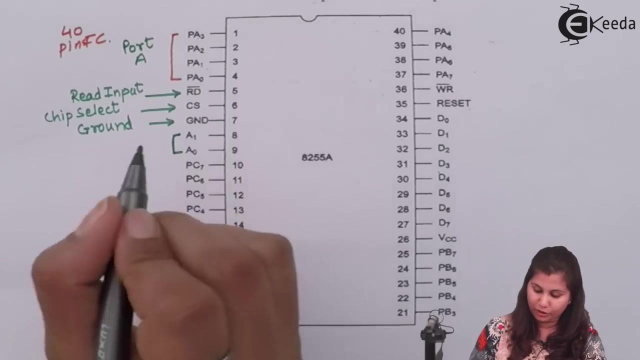 G and D. this is for the ground connection, even- and a, not these are the pot addresses. okay, which port is to be selected and in which mode it is selected? then these are decided by the a naught, and even so, we can say that these are the port addresses. they decide the. 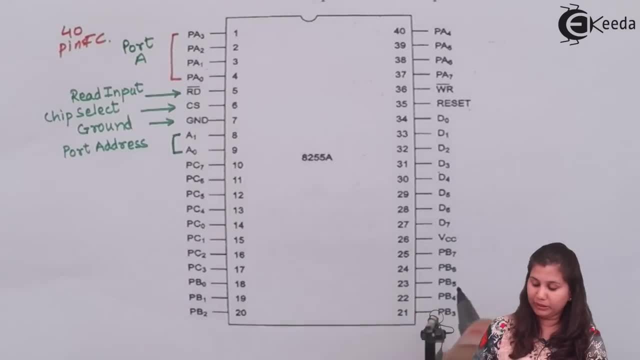 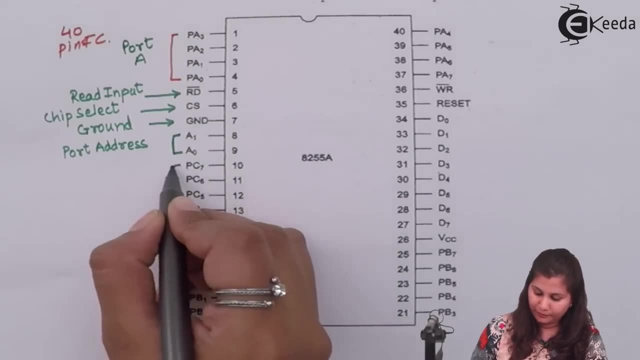 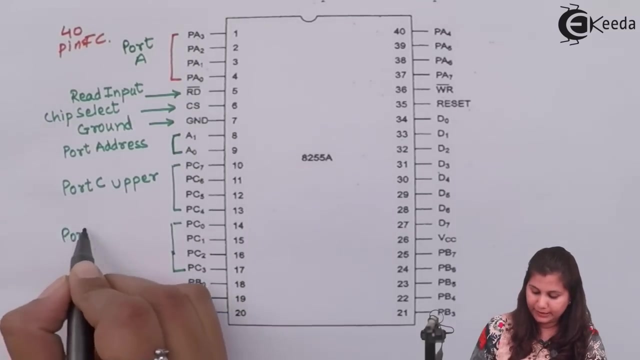 addresses for the ground connection. so here G and D. this is for the ground of the port, that which port out of port A, B and C has to be selected. Then PC7 to PC4, it is port C upper. Then PC0 to PC3, it is port C lower. Then PB0, PB1, PB2, PB3 till. 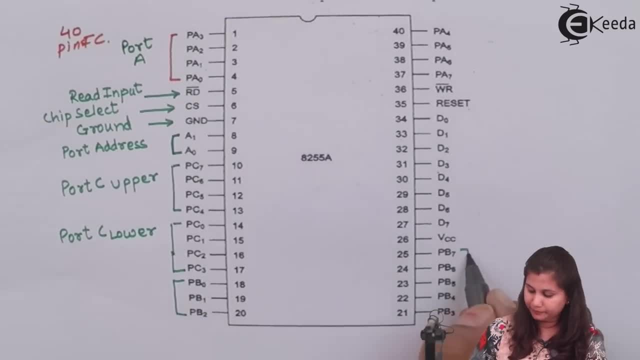 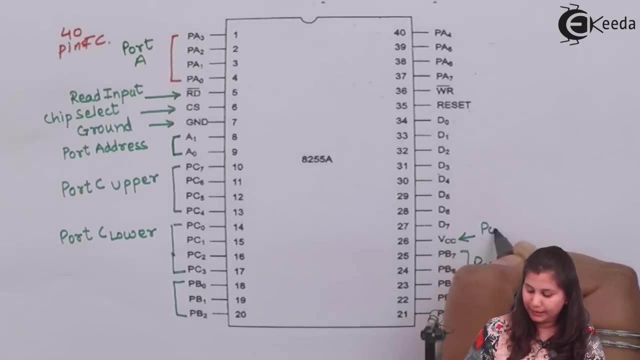 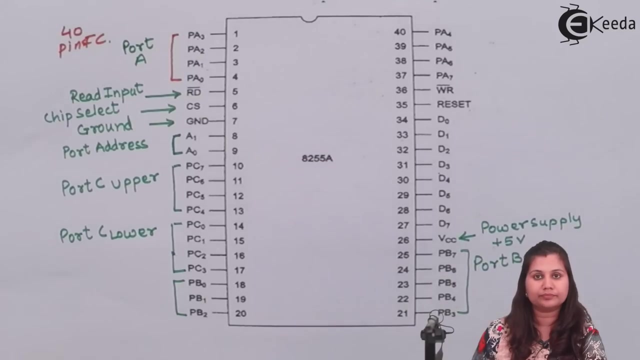 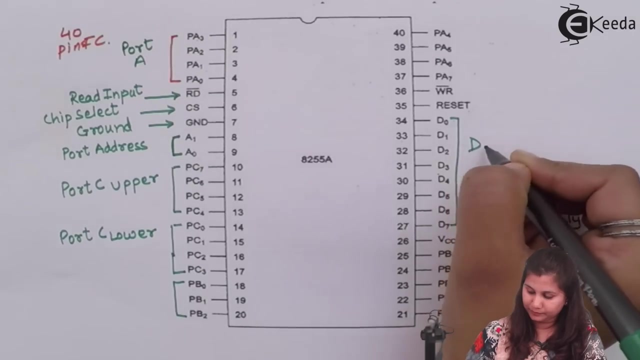 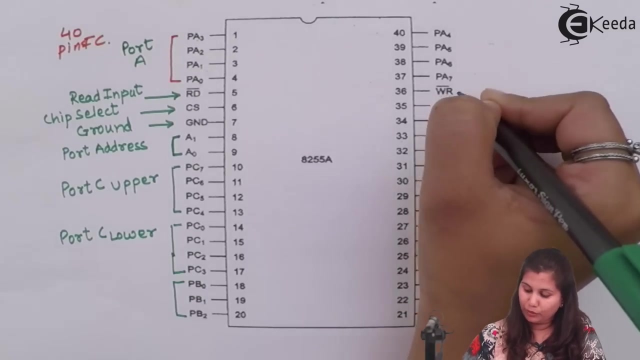 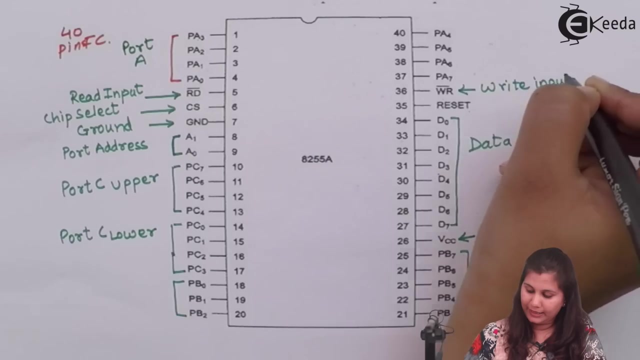 PB7, these are the port B, Then BCC, it is the power supply which is plus 5 volt. Then we have D0 till D7, the data bus, Then reset signal WR bar. it is the right input, And P4 to P7, it is port A. 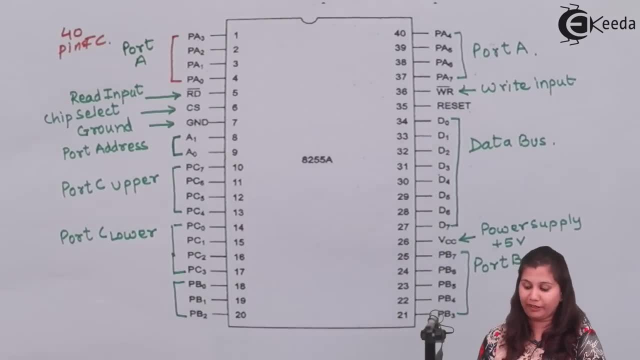 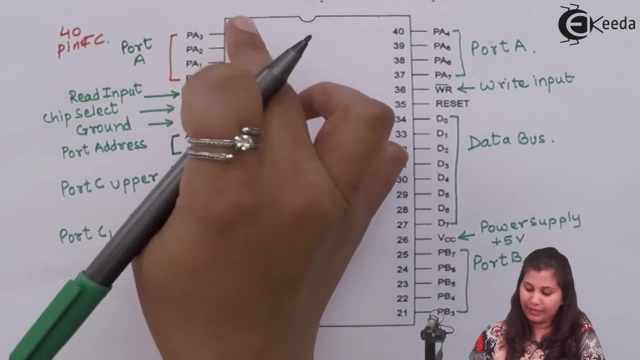 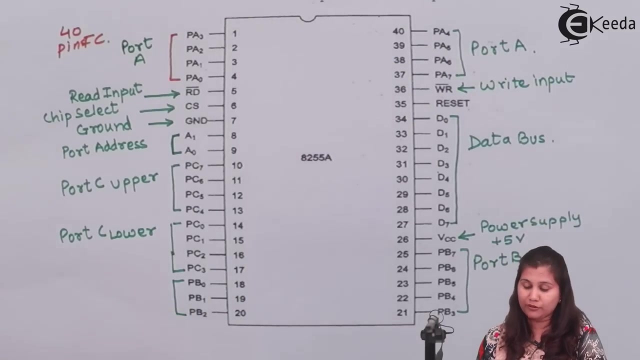 So this is how the 40 pins of the 8255 programmable peripheral interface They are described. Okay, So let's start again. We have the 40 pins from 1 to 20, then 21 to 40.. We have three ports in 8255. 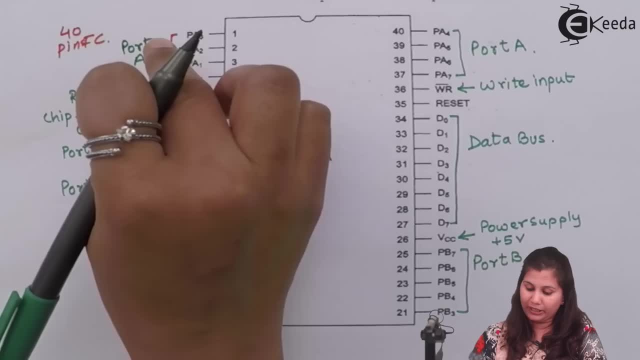 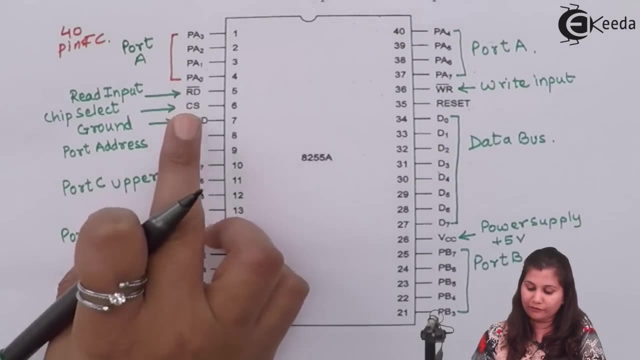 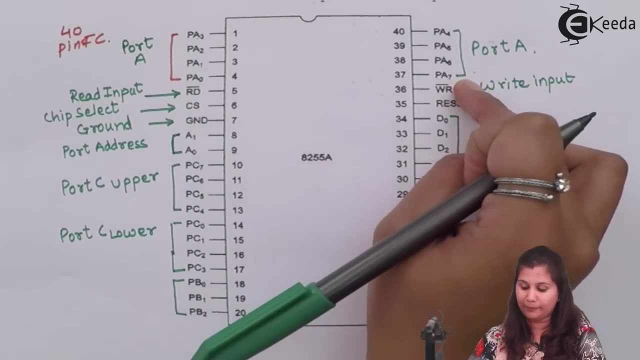 So each port have 8 pins. So we have four pins for port a, then four pins for port a here from 37 to 40. then we have the read chip, select ground, a, naught, a1 and vcc reset and wr rd is for the read input, wr bar it is for the right input. 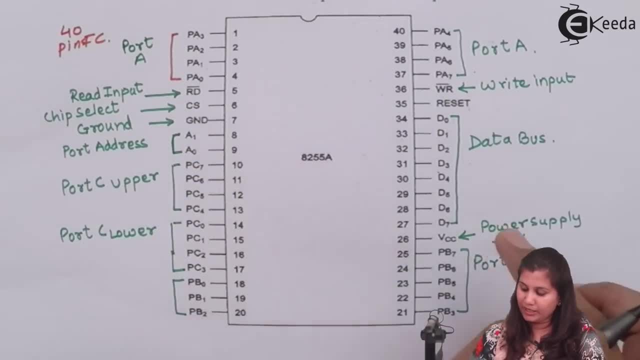 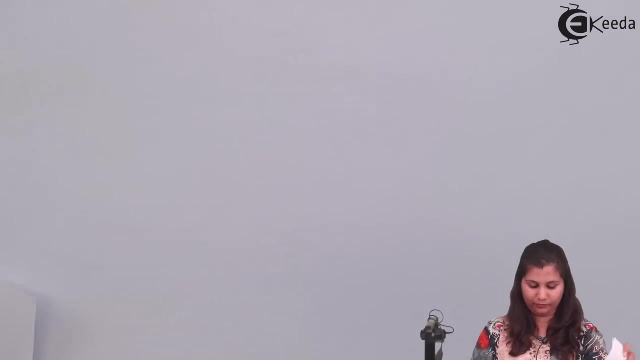 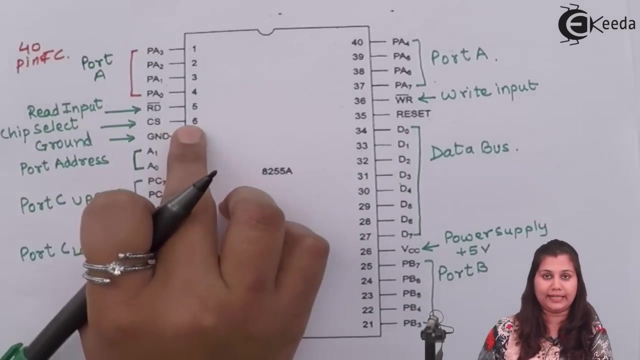 then chip select, then ground, sig is there, ground and vcc are the power supply pins and reset is there. ok, so let us study one by one the description of all the pins of 8 to 5: 5. so first we will start with the chip select, that is c? s. 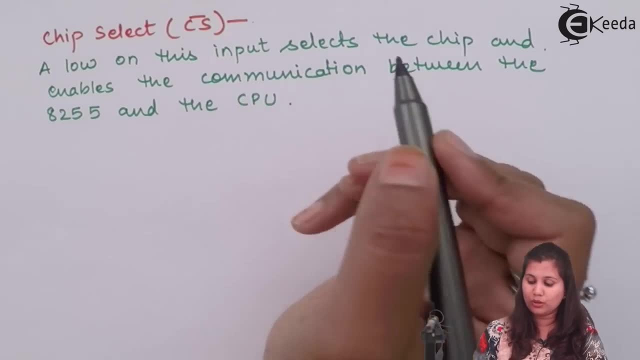 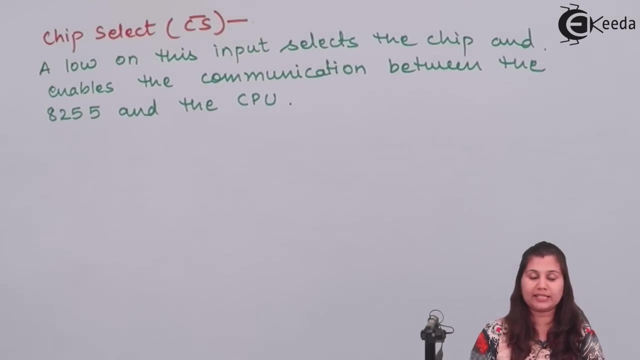 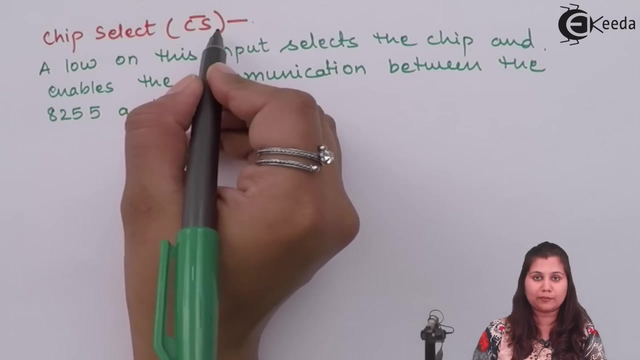 so, Obviously, this pin- it is used to select the chip- means if we want to use the 8 to 5: 5 programmable peripheral interface, then we have to select this chip, this ic, and this chip will be selected when this chips select pin. it is low because we are having cs bar over it, so it's an active low signal. 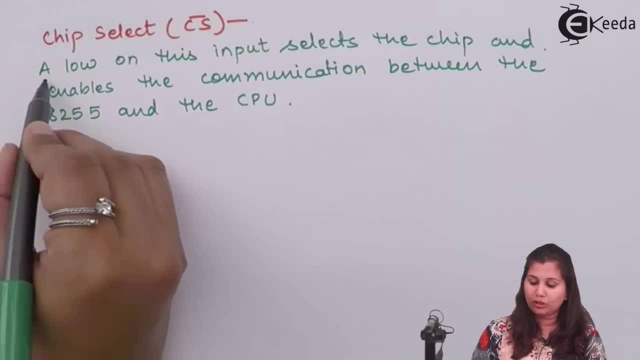 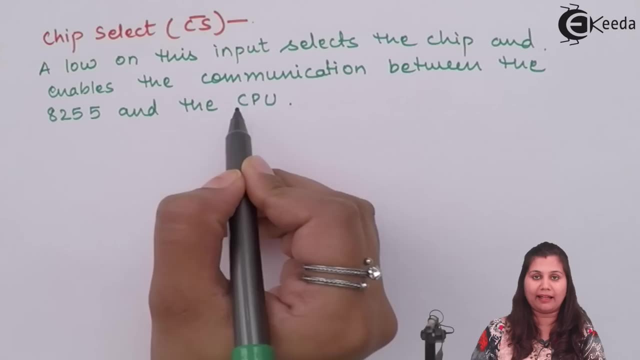 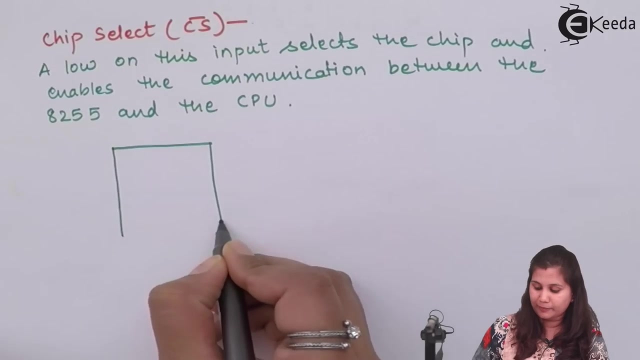 means it is active when its value is zero. so a low on this eight. we can see v is s. so order is 0 and input. it will select the chip and enables the communication between the 8255 and the central processing unit of the microprocessor. so here, if we see, this is our microprocessor mu p. here we 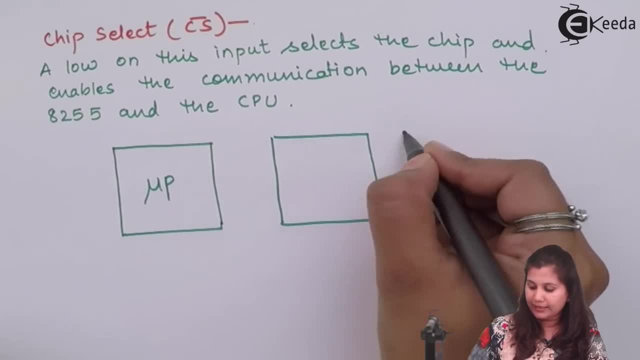 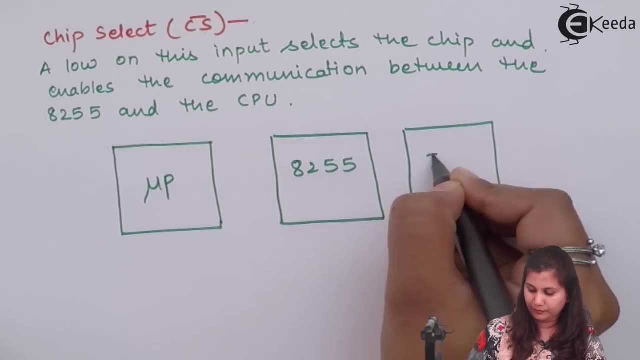 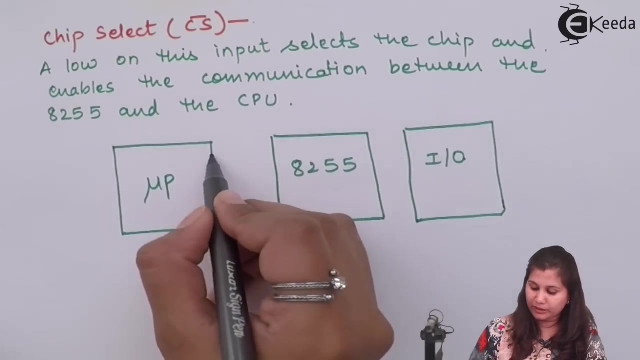 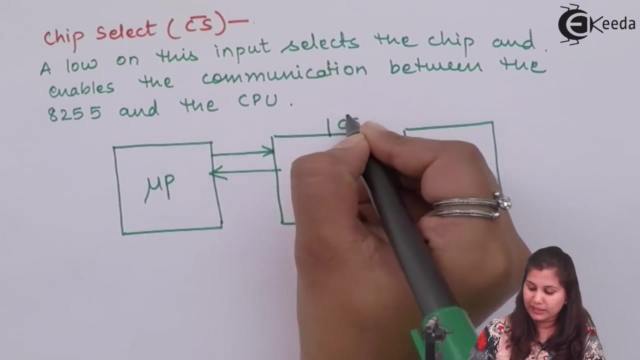 have the 8255 and here we have the input output devices. so this: if we have selected the chip, then it will enable the communication between the microprocessor and the 8255. when on this chip select signal it is low is provided, then the communication between microprocessor and 8255. 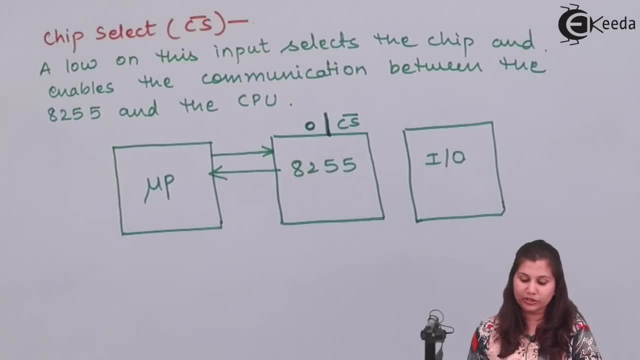 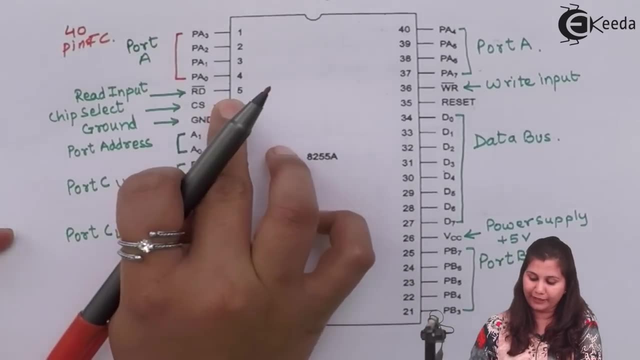 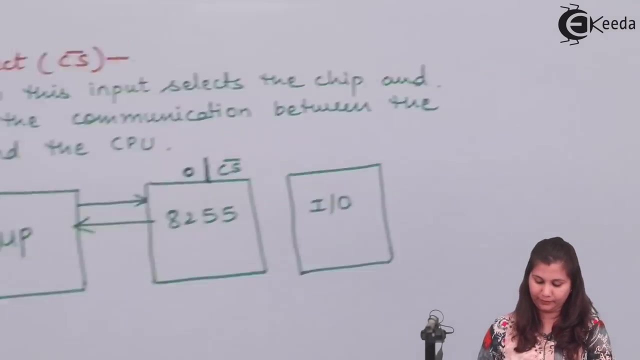 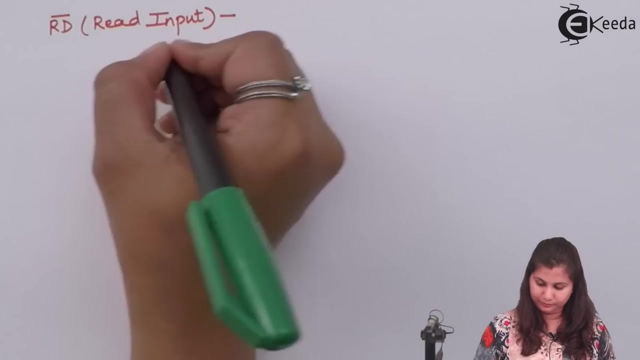 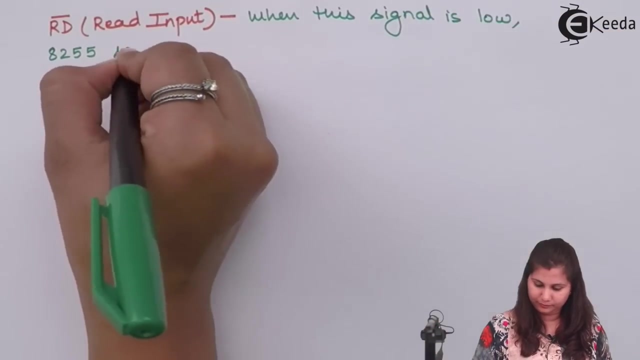 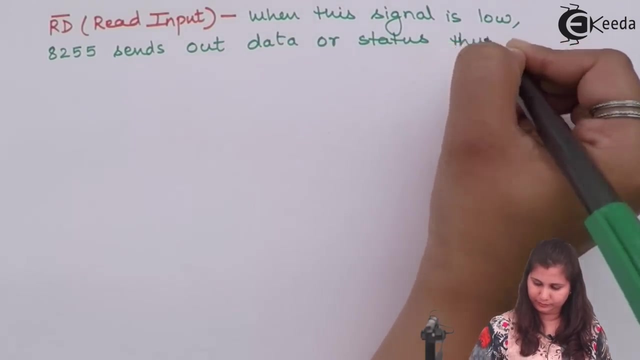 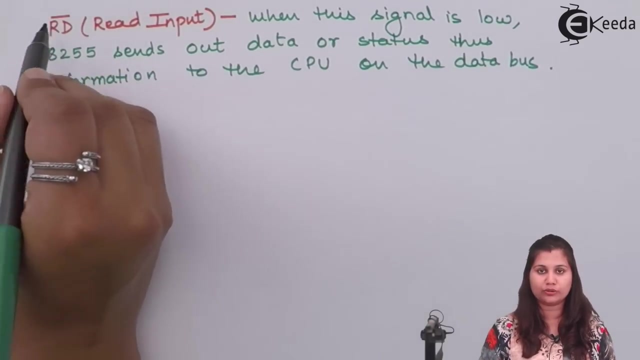 is achieved, the communication will be performed. so this is the use of chip select signal. next, we have Rd bar, which is on pin number 5, which is the read input. so this is read input, and when this signal is low, because we are having bar over it. so 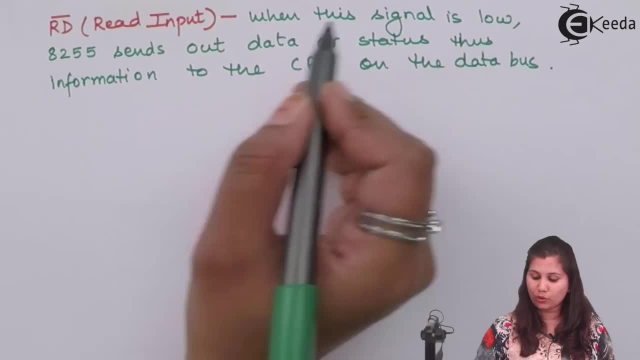 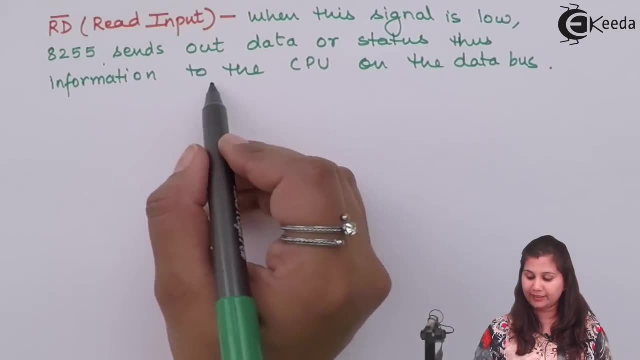 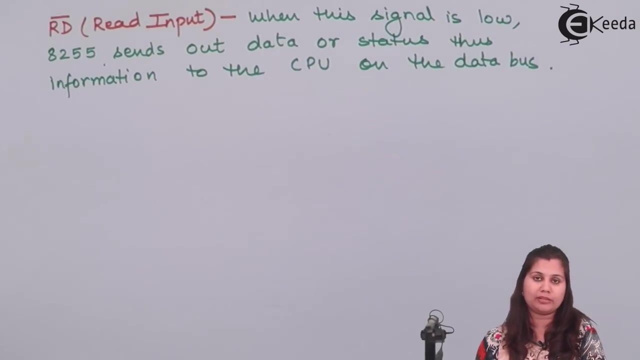 it's again an active low signal. so when this signal is low, 8255 will send out data or status and or it is, or we can say that is sending the information to the cpu on the data bus. it is providing the information to the central processing unit and it is. 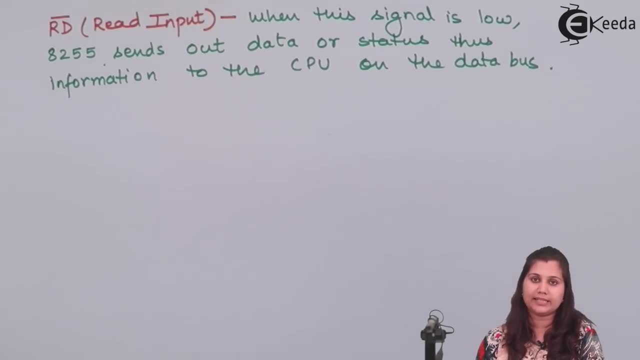 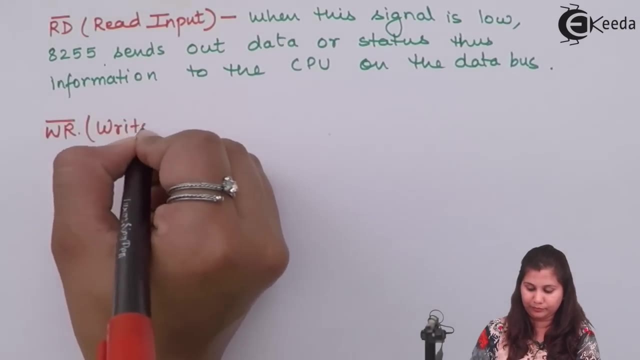 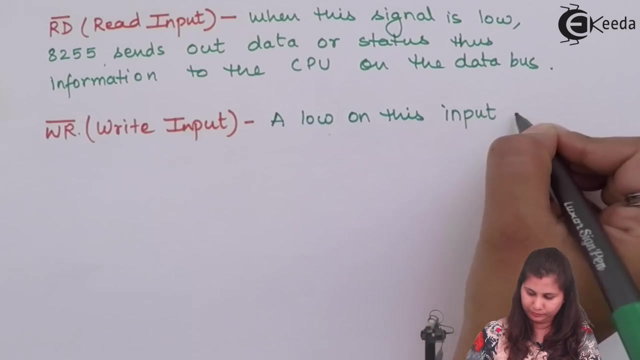 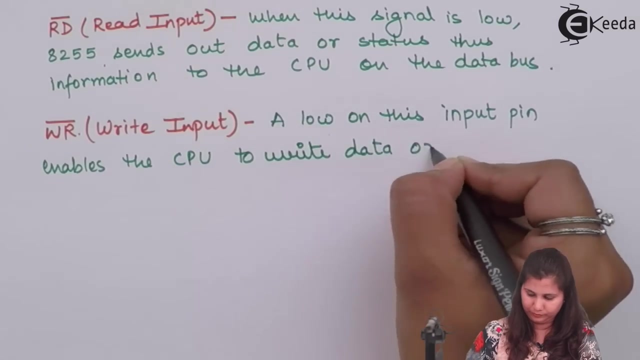 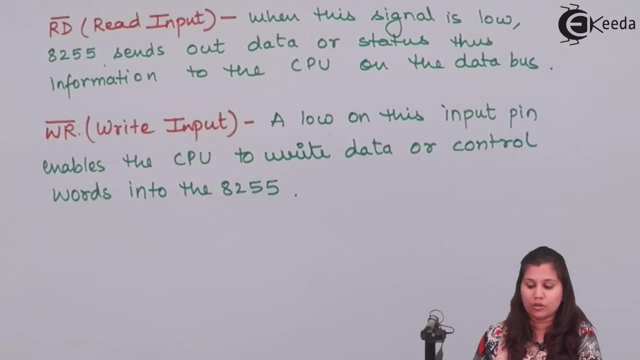 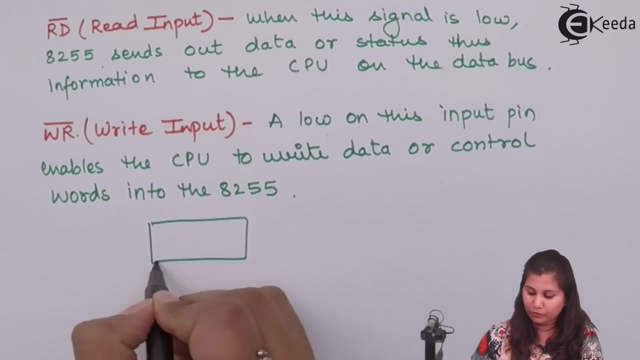 putting the data on the or sending out the data on the data bus. okay, then we have read. so when this right input- we are having a low on this input pin, then it will enable the central processing unit to write the data or control word into the 8255. so if we have here the cpu, 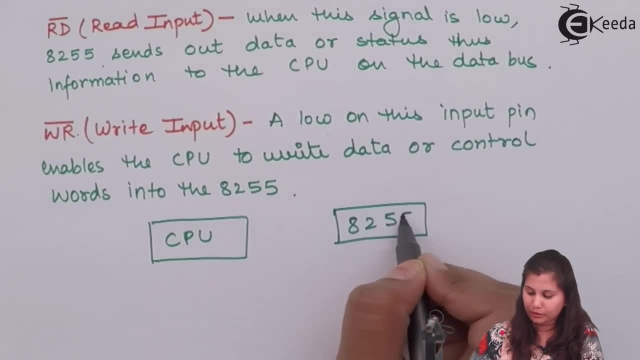 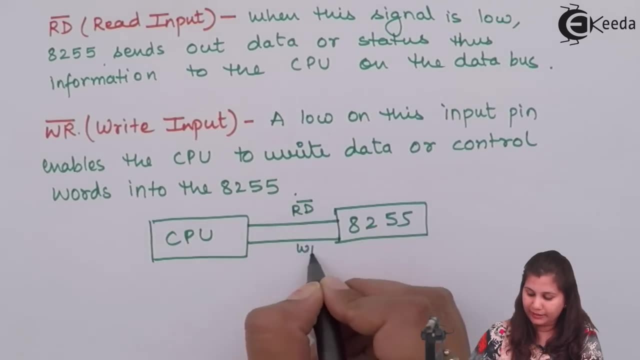 and it is the 8255 and we have the two signals are the bar and right. so when read is there, then the 8255 will send the data to the on the data bus of the CPU. and when rewrite is there, then CPU, it is going to write the data or the control word into the. 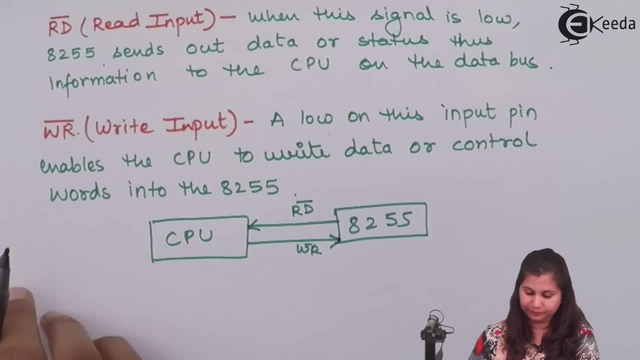 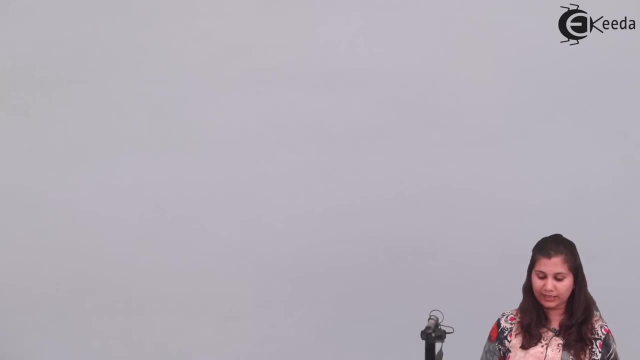 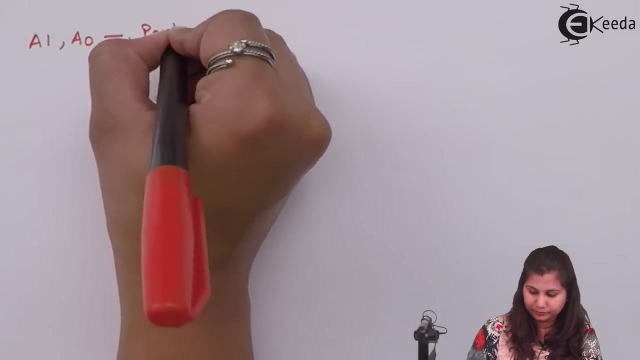 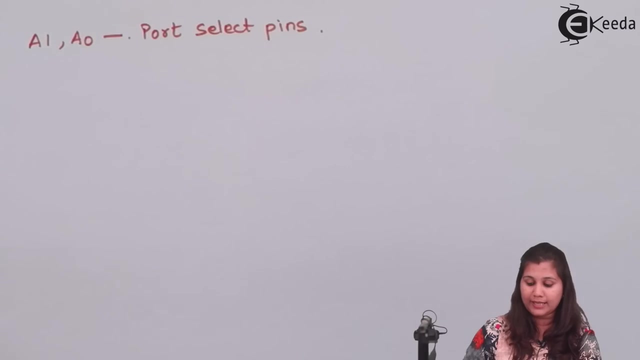 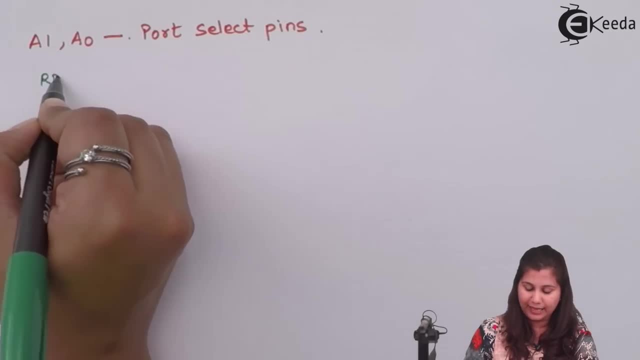 these pins, a, 1 and a not, they are known as the port select pins. so These pins, in conjunction with the read signal and the write signal, means A1,, A0,, read and write. they decide that which of the port is selected by the control board. 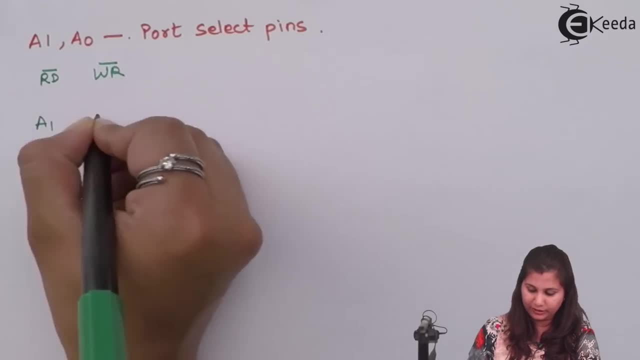 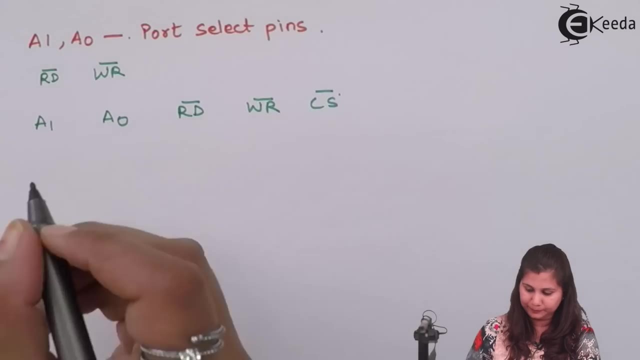 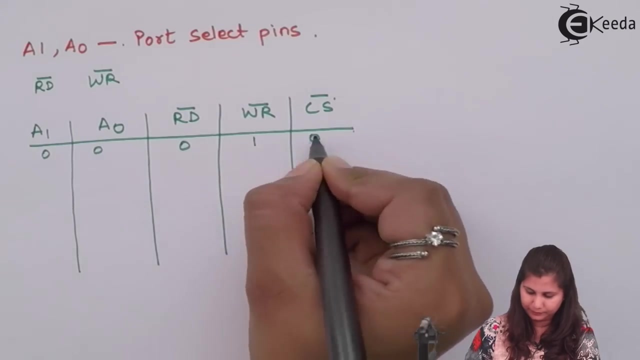 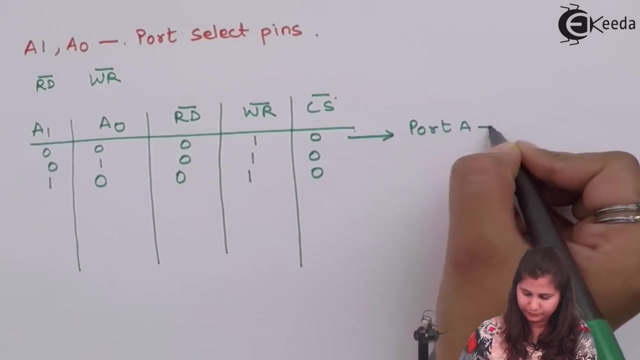 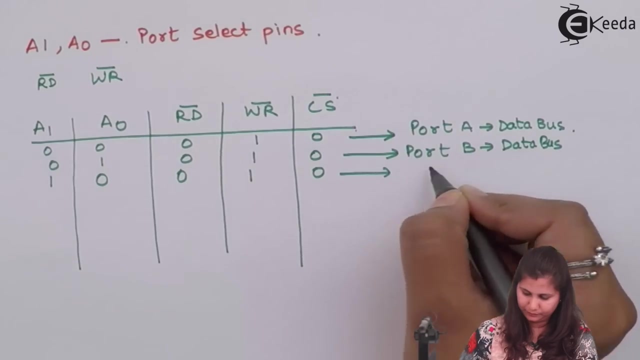 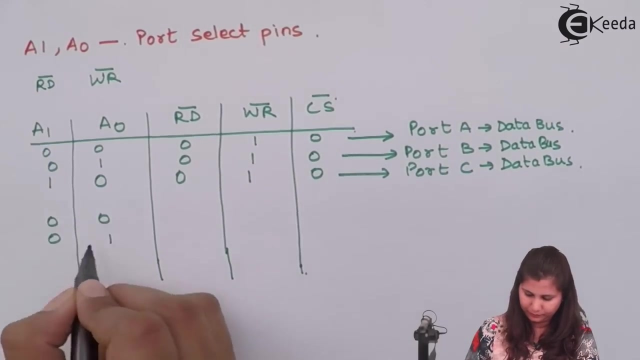 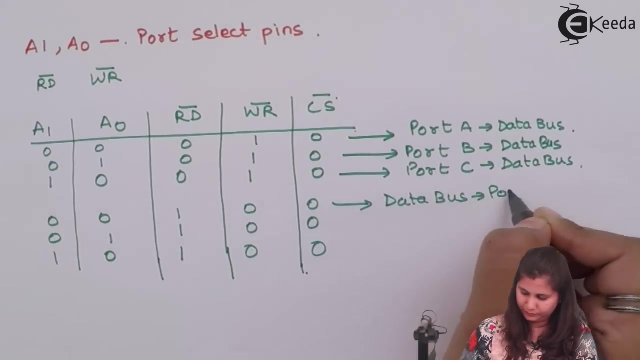 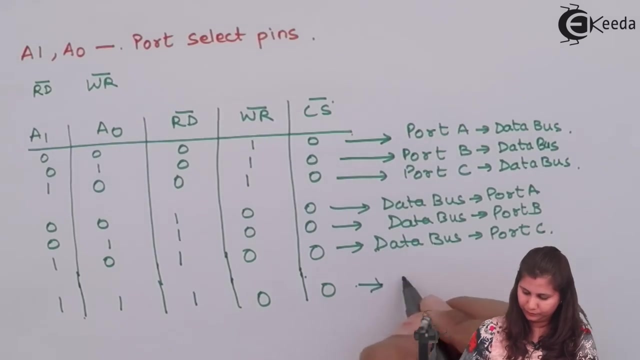 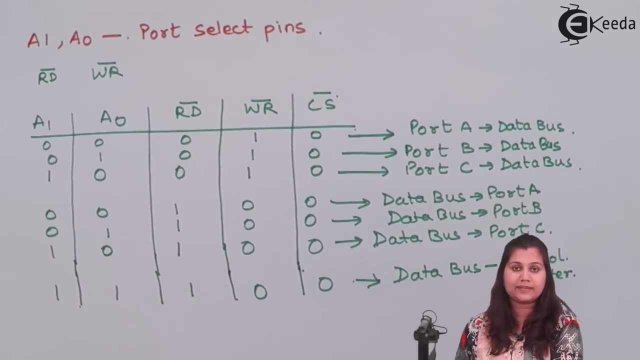 Okay, let's see the table for it. We have A1, A0, RD bar, WR bar and chip select signal. Okay, let's see the table for it. so, as i have said that a1, a0 and read and write these four pins, they are going to decide that. 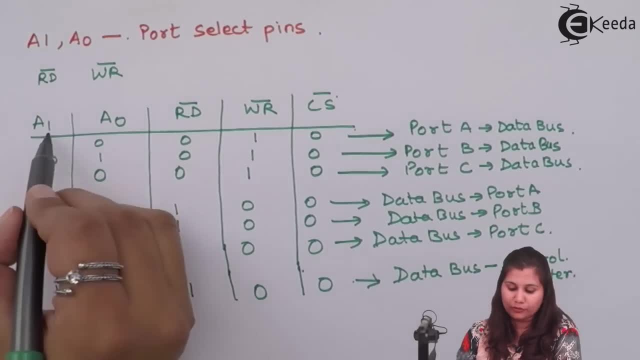 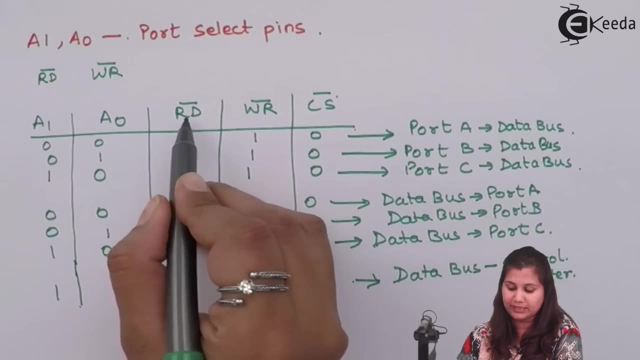 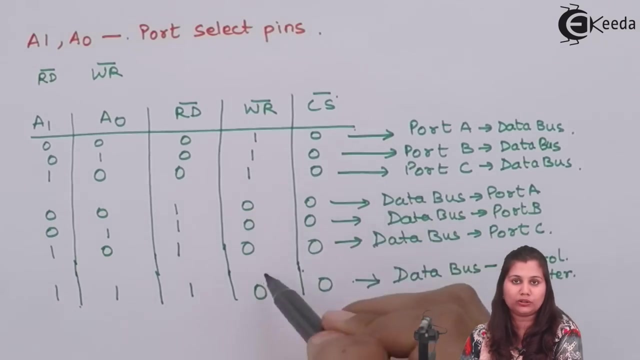 which port is going to be selected. so when the value of a1 and a naught both is zero and the read signal, the read pin, it is zero means it is activated, right is one means it's not activated, and chip select signal, it has to be zero for all the operations, then only the chip 8255 will be. 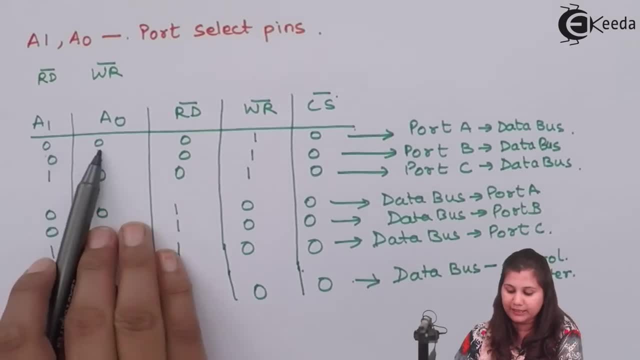 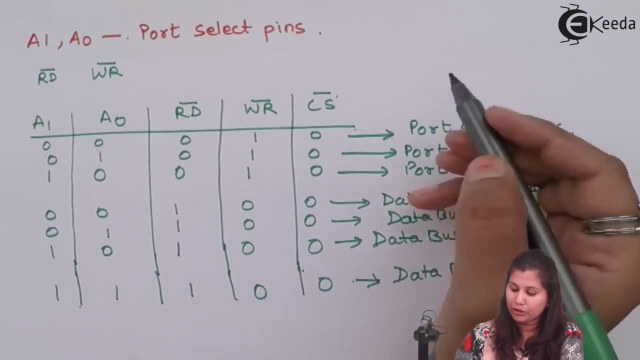 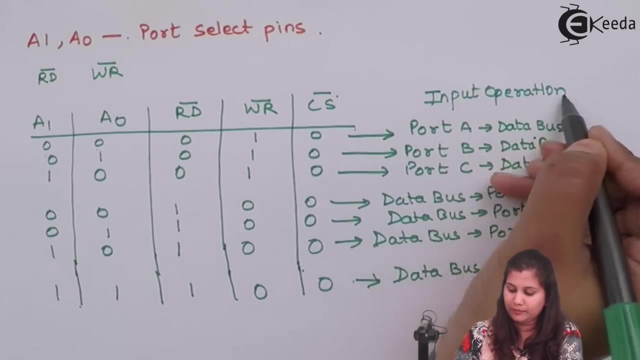 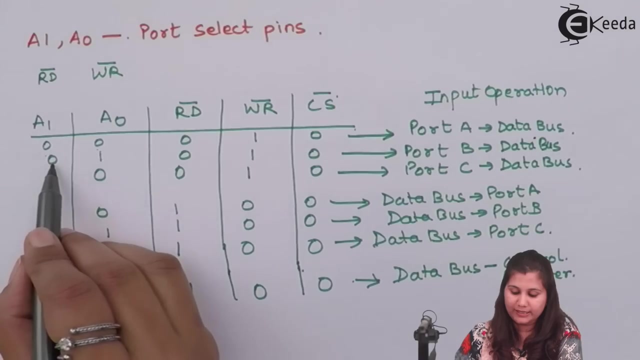 selected. so when a1 and a naught both are zero, then port a is selected and the data on the port a it is given on the data bus. so this is an input operation, means the port a, it is giving an input to the data bus. then a1 is 0, a knot. 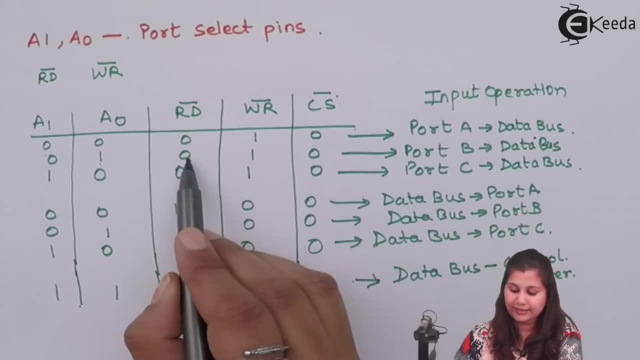 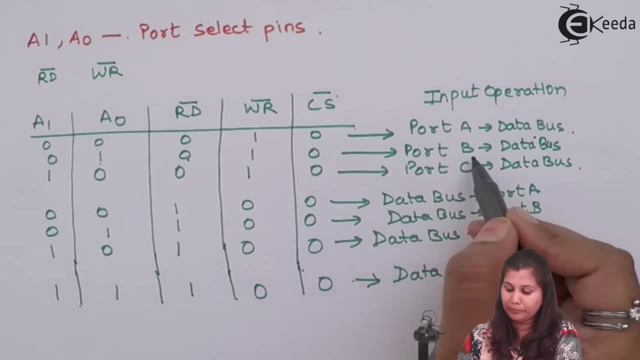 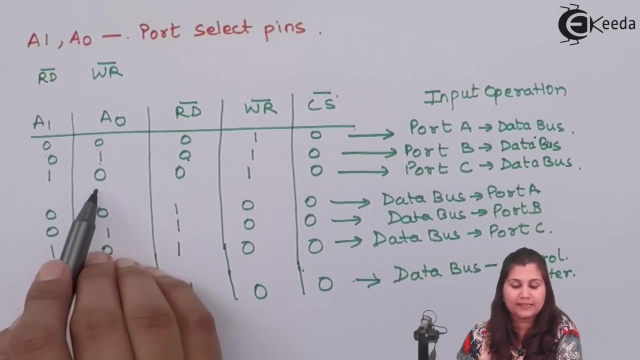 is 1, then port b will be selected and it's a read operation, so port b- it is going to read the data that port b will be read by the data bus. okay, then a 1 is 1 and a naught is 0, support C will be selected. 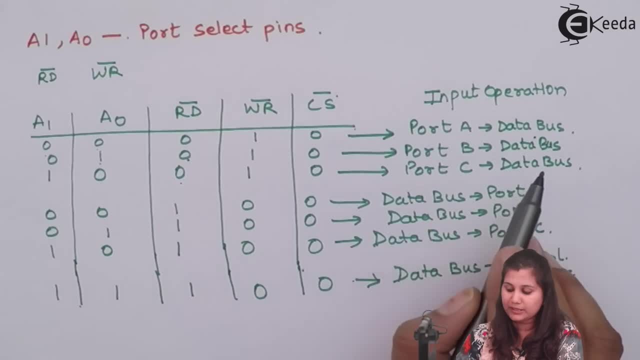 and it's a read operation, so data was it is going to read the data from the port C, so data was it is getting the input from the three ports. okay, so this is describing the input operation. now again, 0, 0, support, a will be selected and the 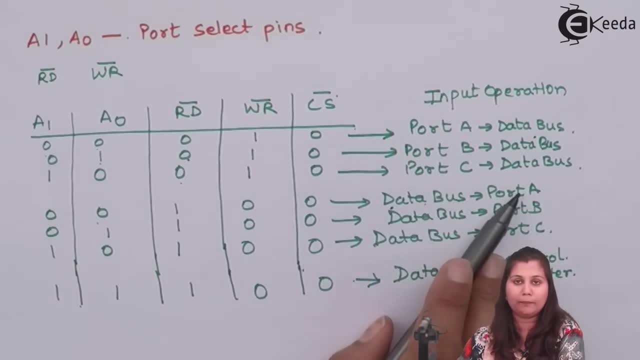 data which is available on the data bus. it is given on port a, so this will be an output operation. okay, so these three are the output operation. then a? 1 is 0 and a naught as 1, then port B selected. when a 1 and a naught, it's 1 and 0, then port C is. 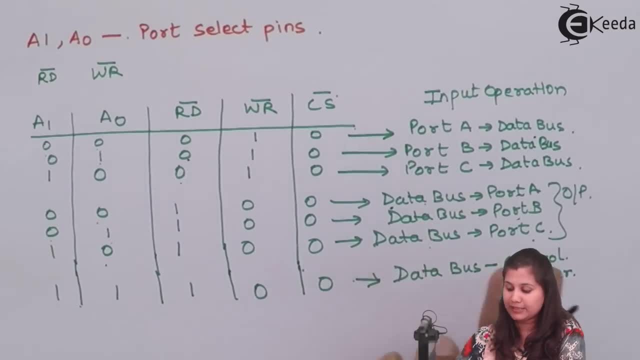 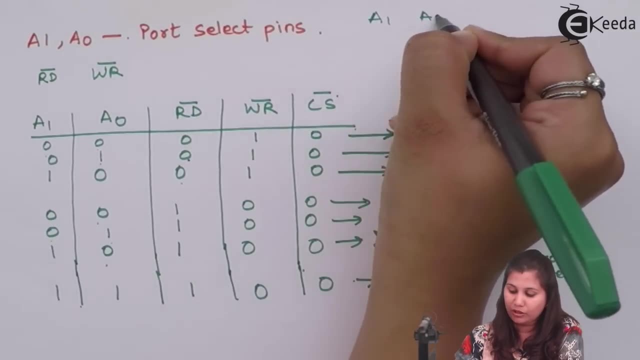 selected. so the data which is available on the data bus it is given on the three ports. so it's an output operation. so we can say that when a, 1 and a, A naught they are 0- 0, then port a is selected, when they are 0- 1, then port B. 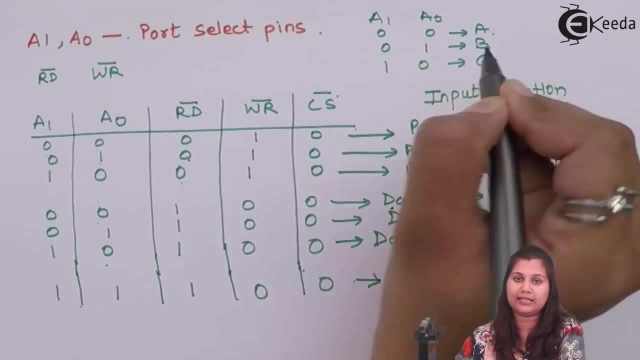 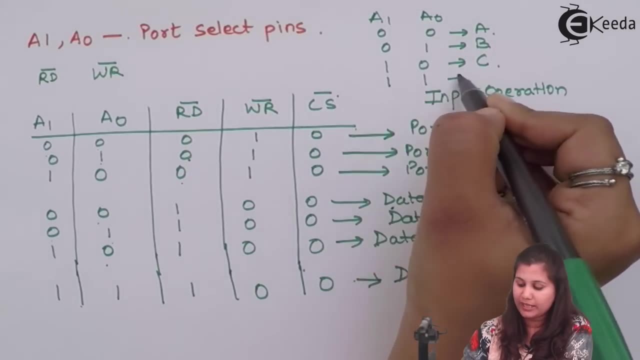 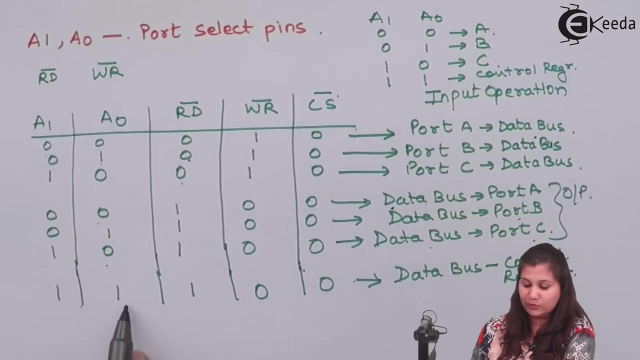 is selected, and when they are 1- 0, then port C is selected. okay, now when the value of this a 1 and a naught it is 1- 1, then control register is going to be selected. okay, so when its value is 1- 1, it's a read operation, then data bus it. 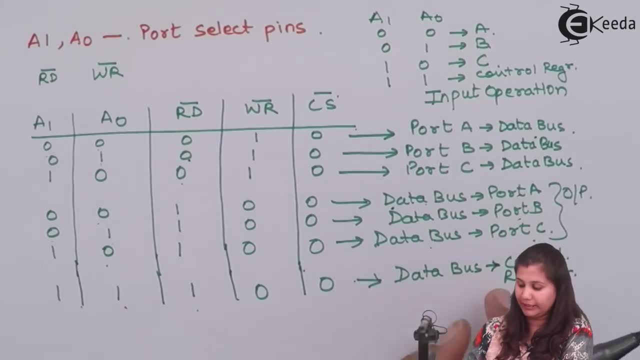 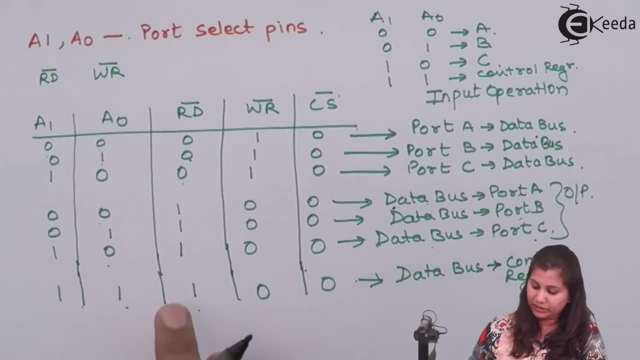 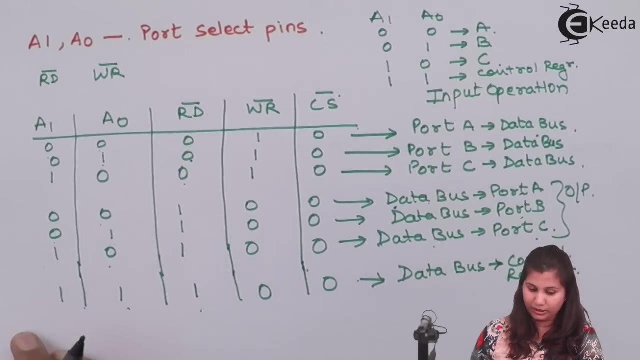 is going to give the the data which is available on the data bus. it will be loaded into the control register. okay, so because it's read is 1 and write is 0, so that data will be written on the control register. okay, so we can say that these 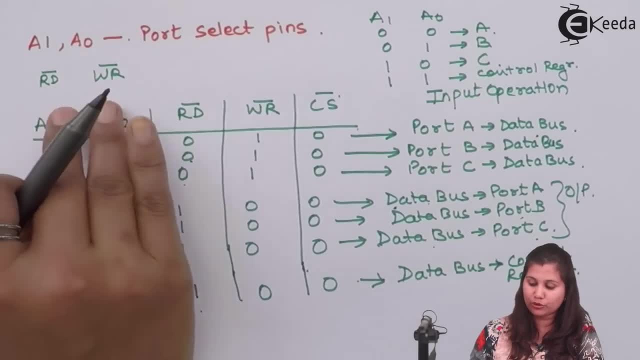 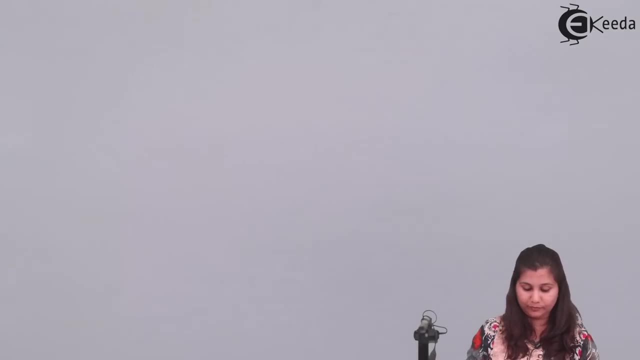 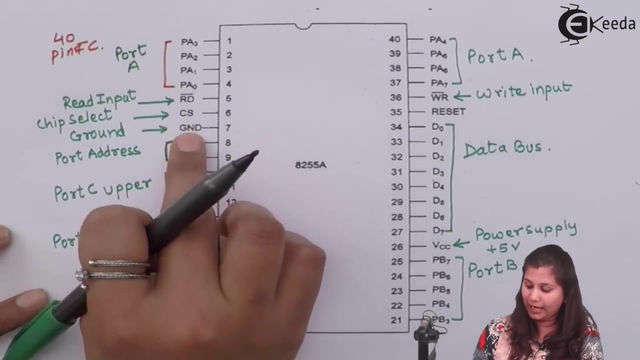 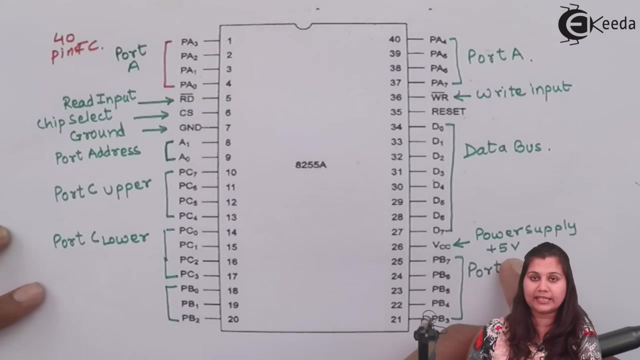 two pins: port select pins. they are used to select the three ports a, B and C. okay, next, in the pin diagram we have- we have studied, read- we have chip select signal, ground and power supply. they are the power supply pins. ground is connected to the earth and VCC it is connected to the plus 5 volts power supply. we are left. 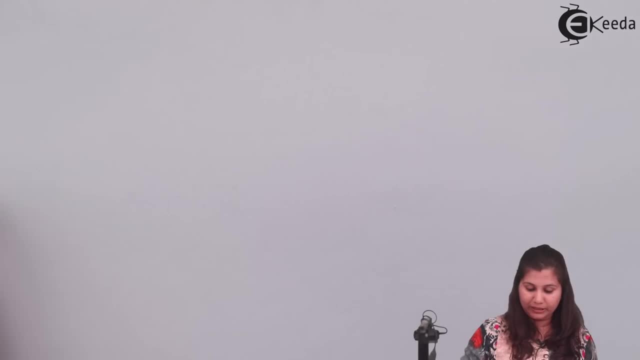 with this reset pin. okay, so reset pin. it is used to clear the control register, though, as I have said that there are various modes in which the 8255 works and these modes. which mode is going to be work? it is decided by the control word which is written in the control register. now, if 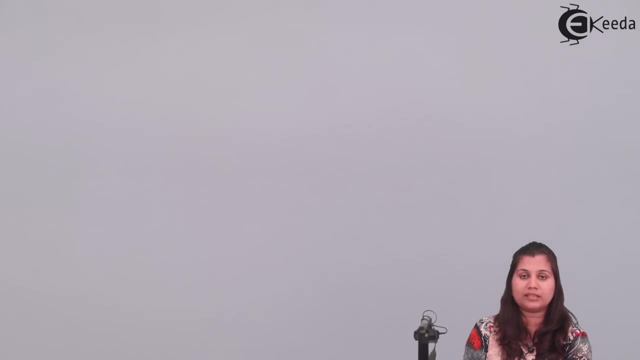 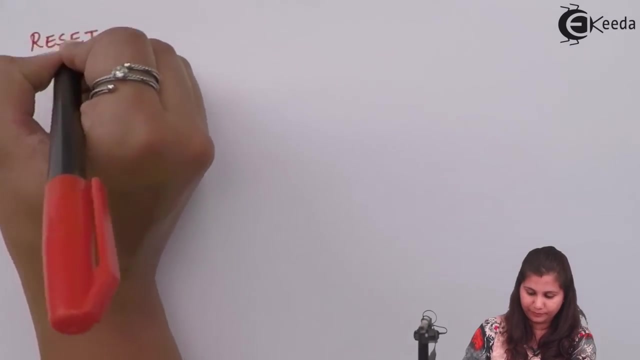 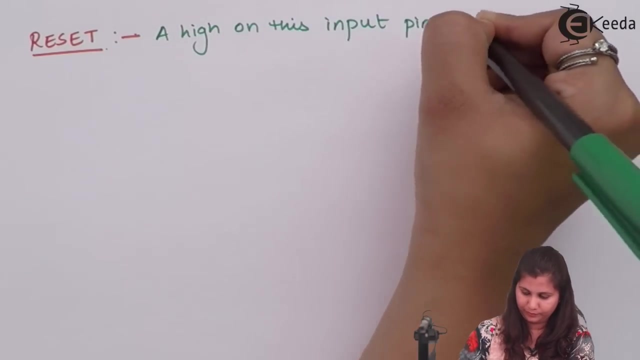 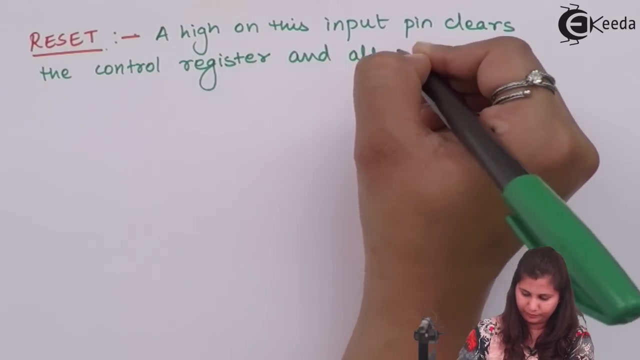 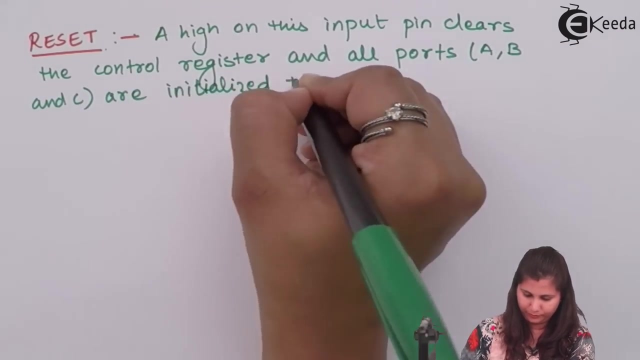 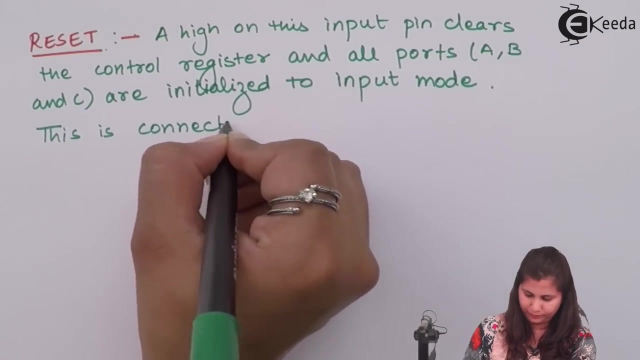 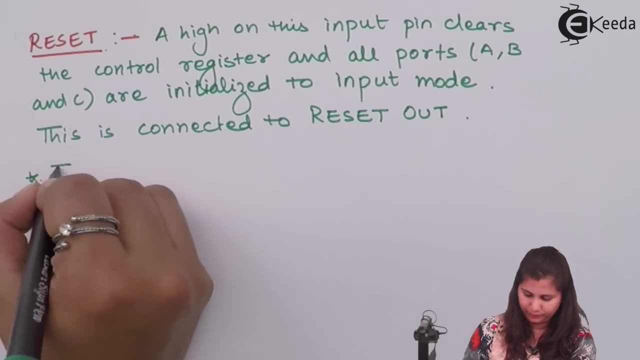 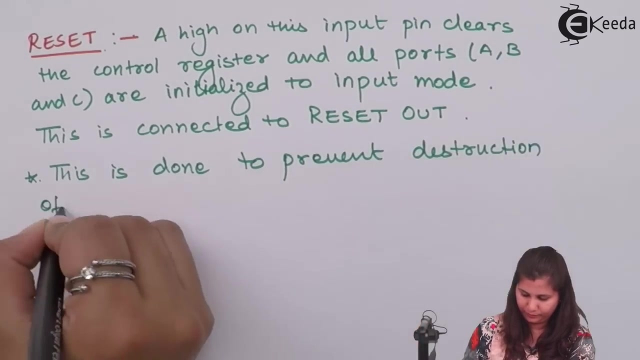 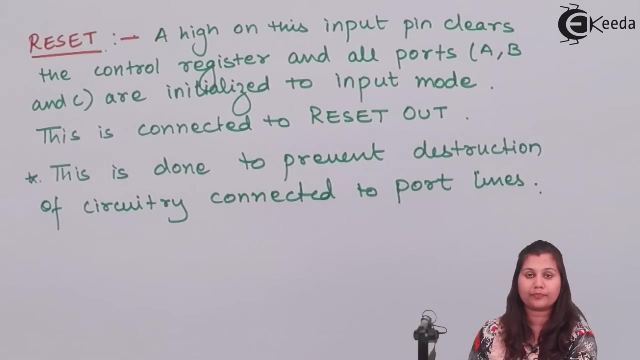 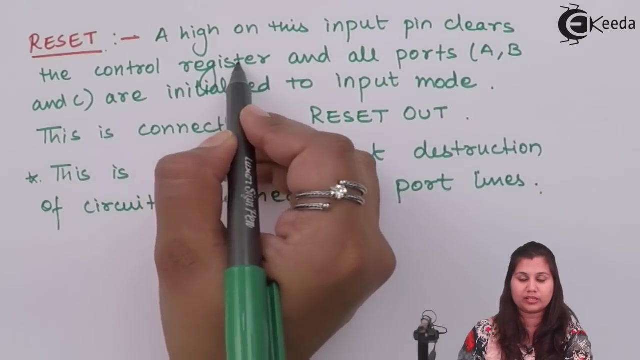 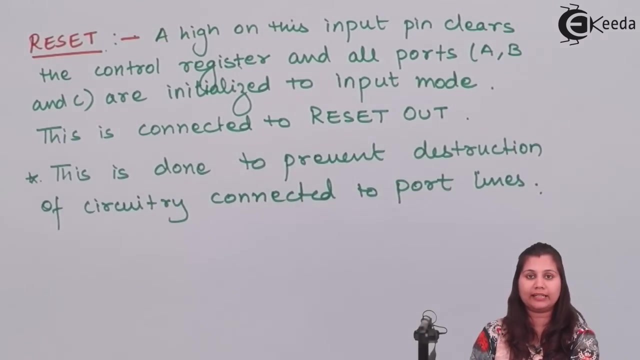 you want to clear the contents of the control register, then this reset pin is used. you here soj, you, you, you, you, you. so this reset pin, when it is high on this input pin, it will clear the control registers and all the ports a, b and c. they are initialized to the input mode. that means they will act as an input. 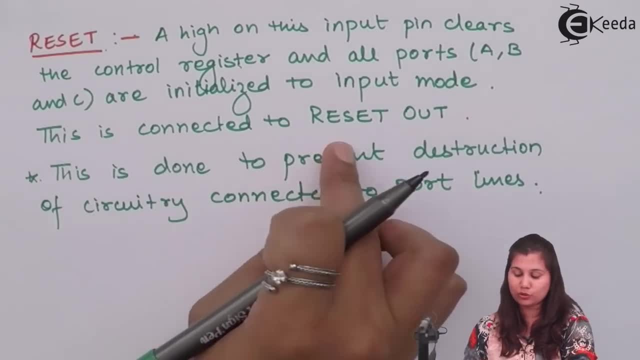 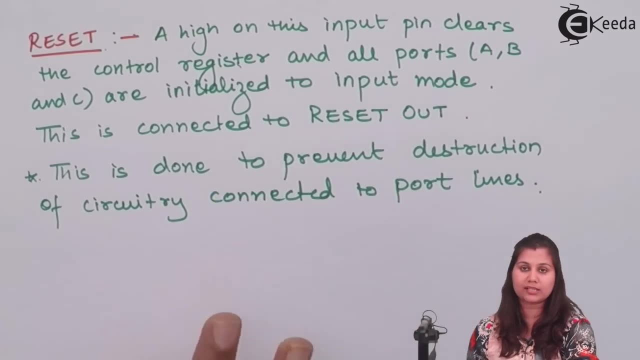 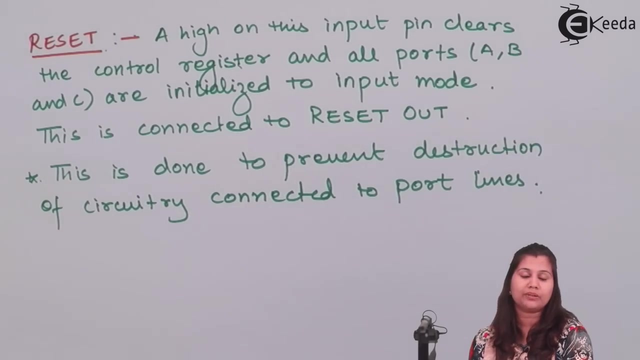 ports and this pin? it is connected to the reset out pin of the air microprocessor and this is done to prevent the destruction of the circuitry which is connected to the port lines. why we are clearing out to this? because we want to prevent the damage of the circuitry which is connected. 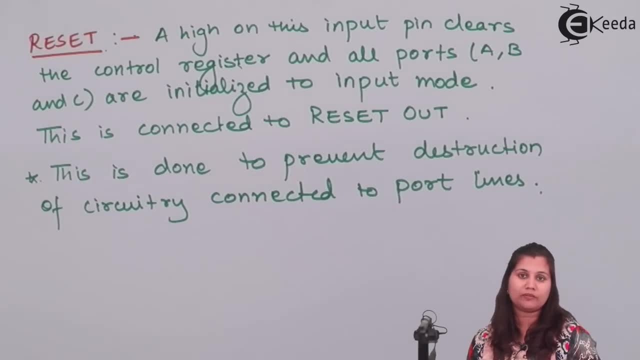 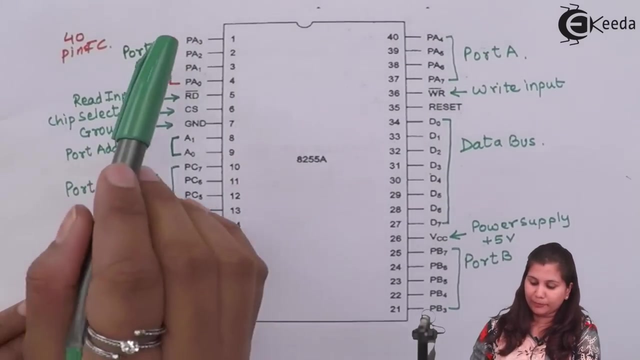 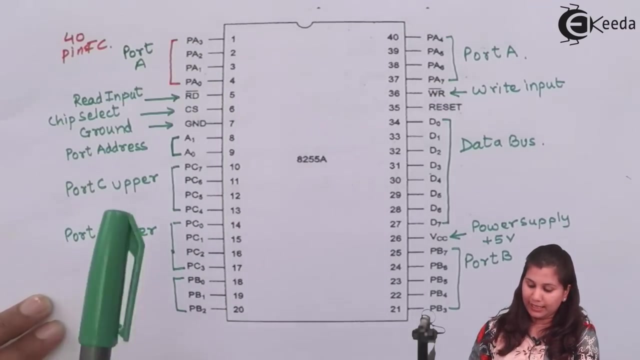 to the port lines. okay, so the main purpose of this reset pin? it is to clear the control register and to initialize all the ports in the input mode. so this was the reset pin. so in this pin diagram we have the port a, which is the 8-bit port, and port B and port C, which are also 8-bit ports, and port C. 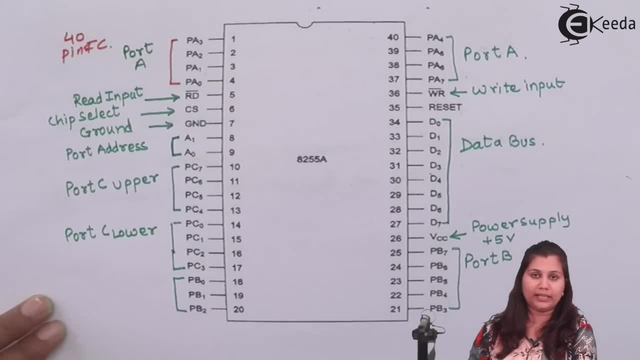 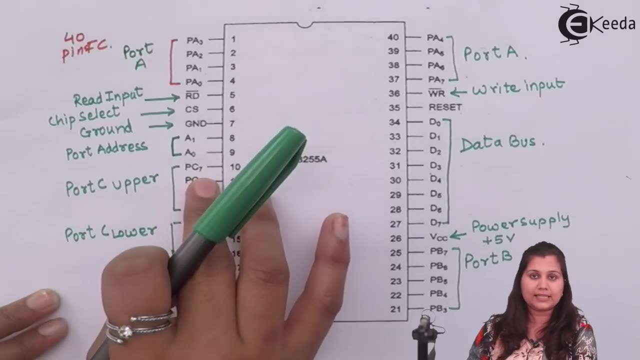 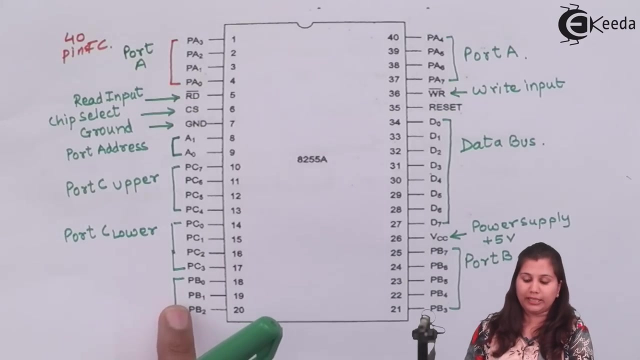 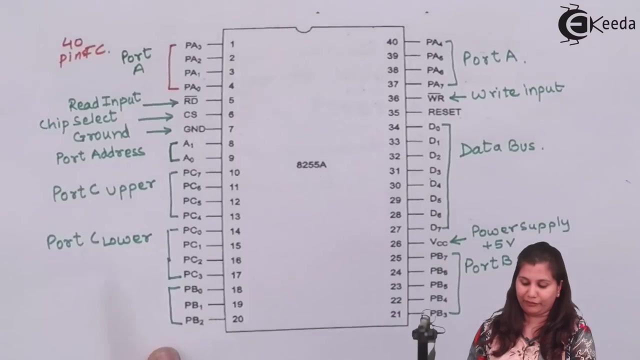 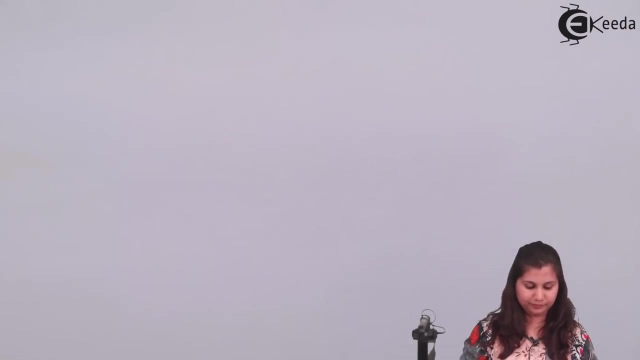 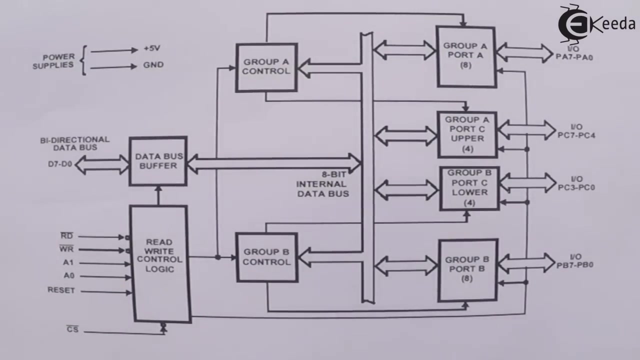 it is divided into four bit ports: port a, port C upper and port C lower, and the other pins which we have, which are present in this pin diagram. we have this course. so we have completed this pin description of the 8255, this pin diagram. now let's come to the block diagram of 8255. this is the block diagram of 8255: programmable peripheral. 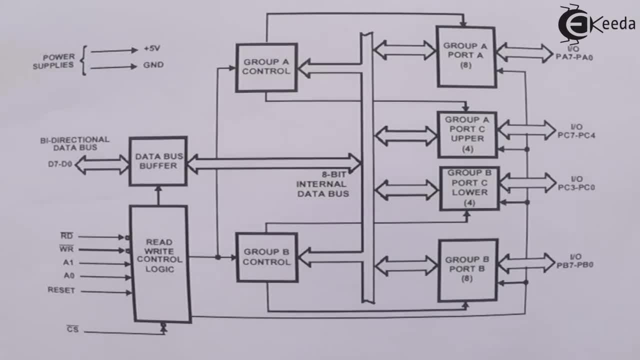 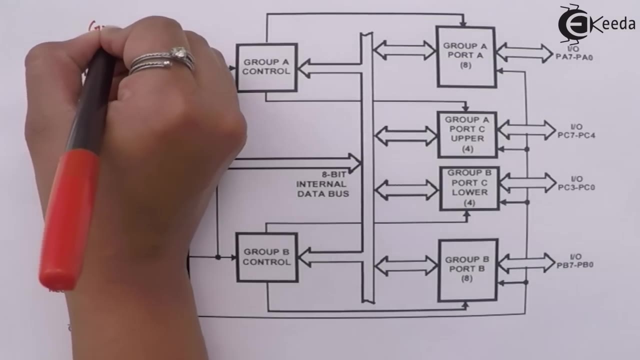 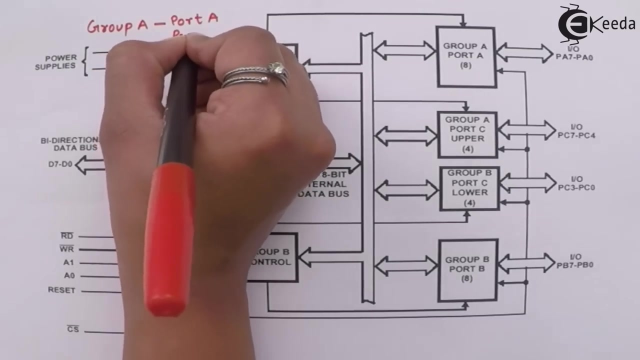 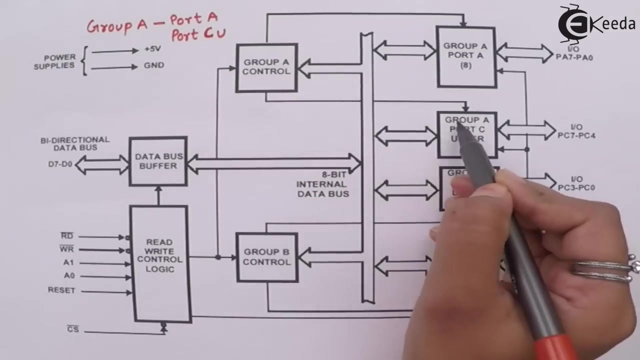 interface in this block diagram. you can see that you have two parts here: group a control and group B control. in group a we have the port a and the port C upper. you can see that the group a control is the control. it is controlling the group a, port C upper, the four lines which are from pc7 to pc4 and 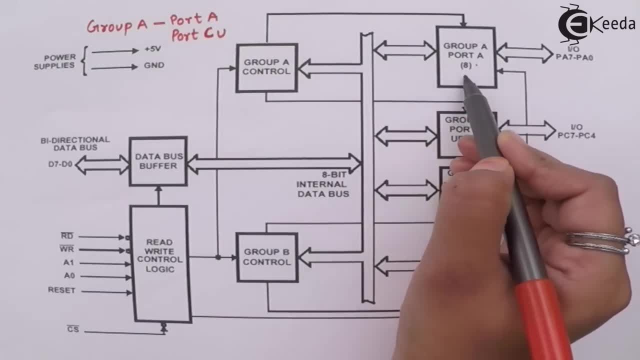 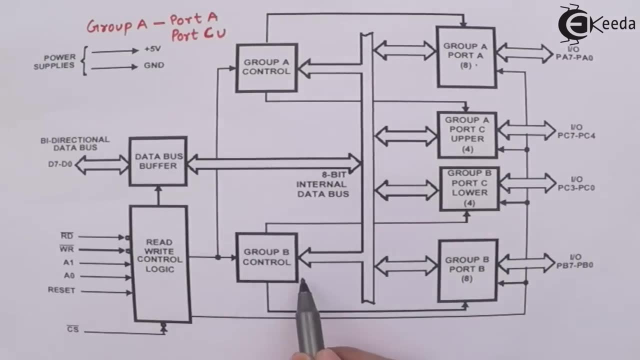 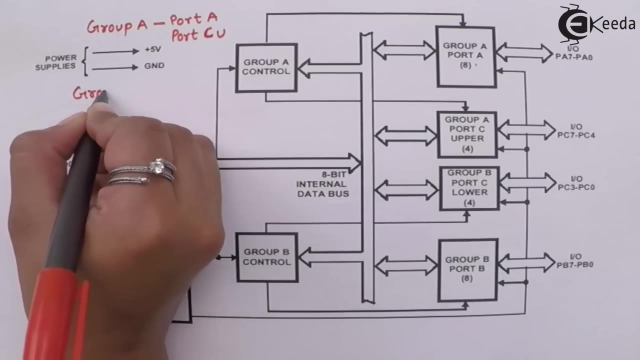 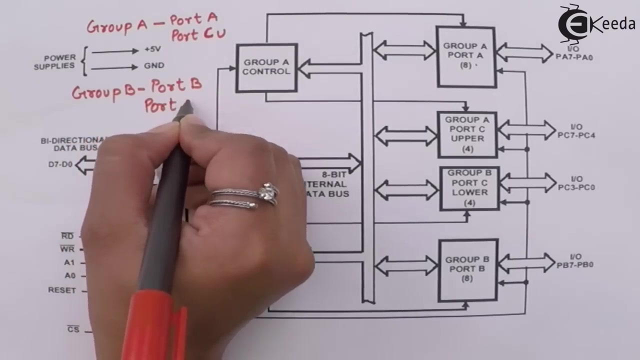 also the group a, port a, which is having eight lines, PA0 to PA7. okay, then we have the group B, control, which is having port B and port C. lower then the dependent to the lot mates. each group is having port P, it is having eight inside. 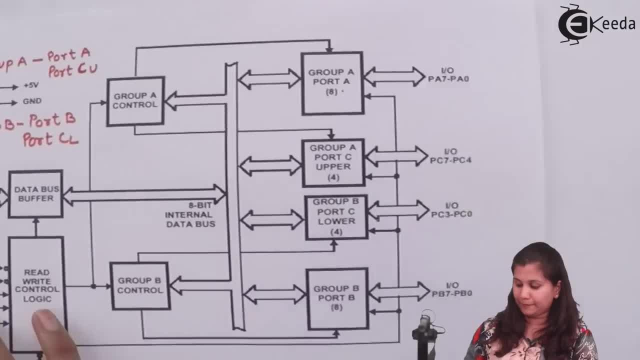 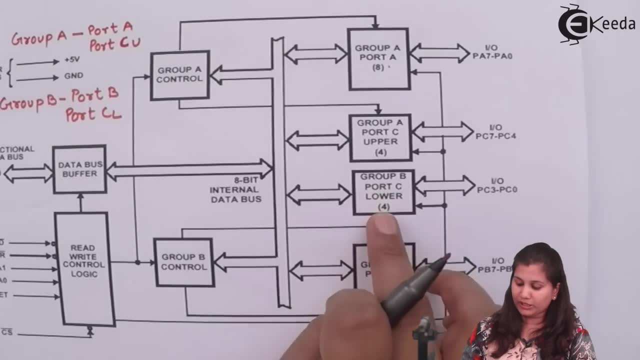 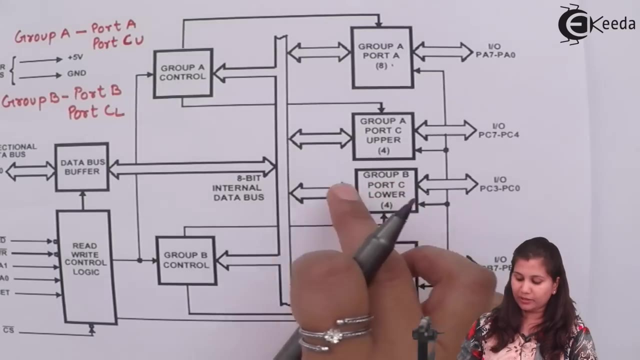 the lymphahn別阿 Med ㄱ lines here, and the eight lines of this are from PB not to PB 7. then port C lower, we have PC3 to PC, not okay. so these two port line ports, they are controlled by this group B control. and these two group a, this port a to Pb7 and this ㄱ'll remain a little one and you can see that stage pointsина they are starting to go to 3 different port, bena, and then in by ㄱ they're going to go to b at ㄱ. 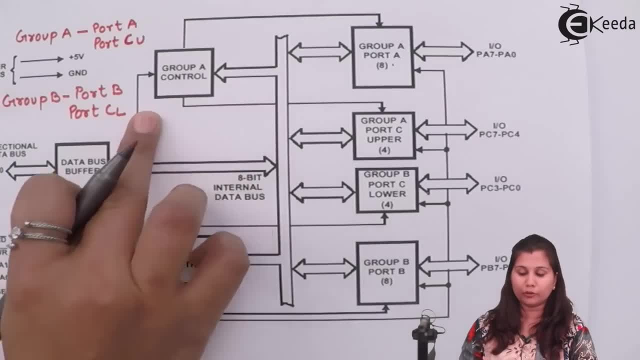 then they're going to stop. you can see this will be okay up to b and then we stay in before. ㄱ will stay up to b and then sister p or E will also Sheer. Thank you very. c a and port c upper. they are controlled by the group a control. the lines are going to each of the 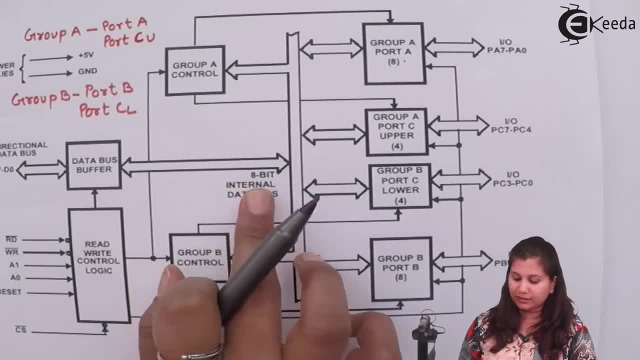 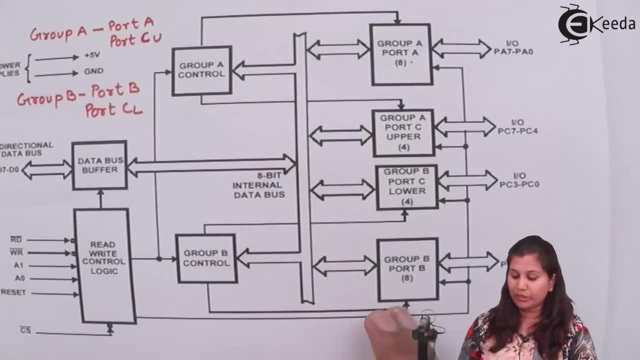 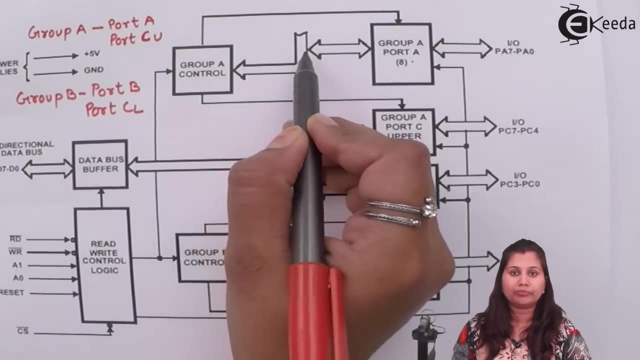 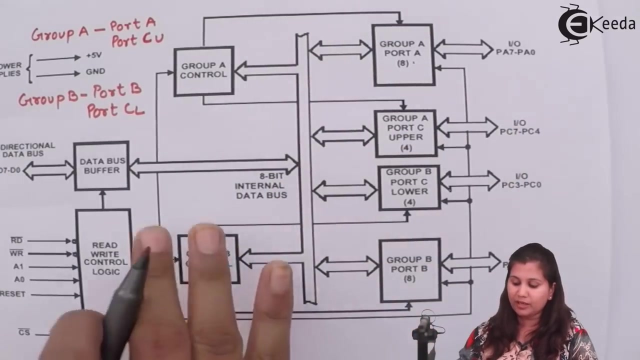 ports. okay, then we have an internal 8-bit data bus. okay, and this data bus. it is connected to all the ports, the data can be read from the data bus and also the data from the ports can be written on the data bus. okay, so we have this 8-bit internal data bus which is connected with 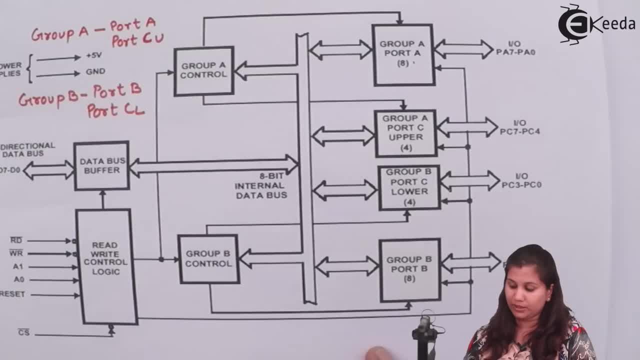 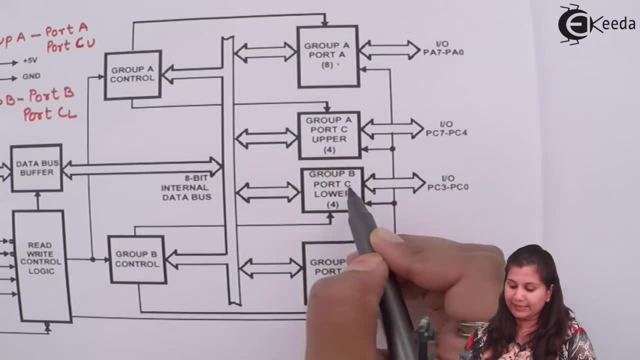 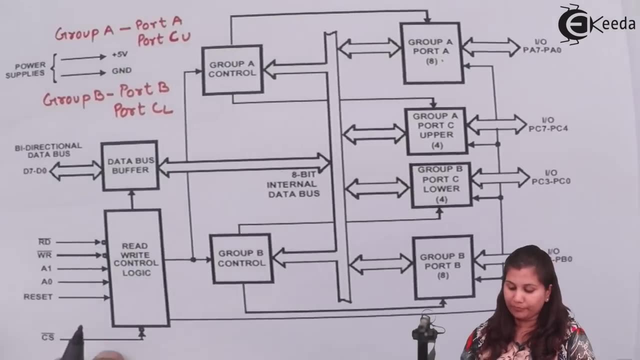 the controls also and to all the ports. now these in ports, they can act as an input output ports. so we have these bi-directional lines here, which is showing that they can be used as an input output ports, depending upon the modes. now, here we have this data bus. it has a data bus. 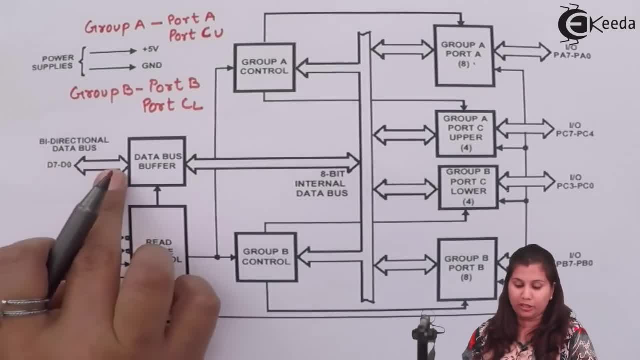 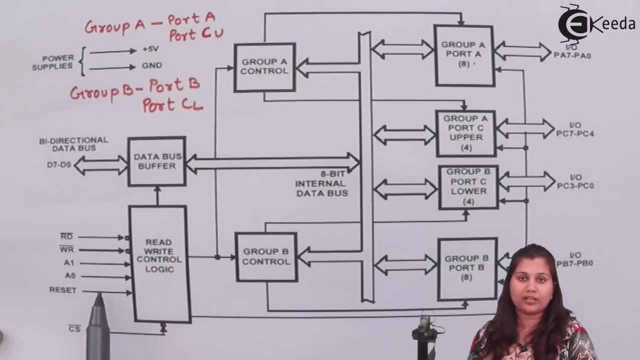 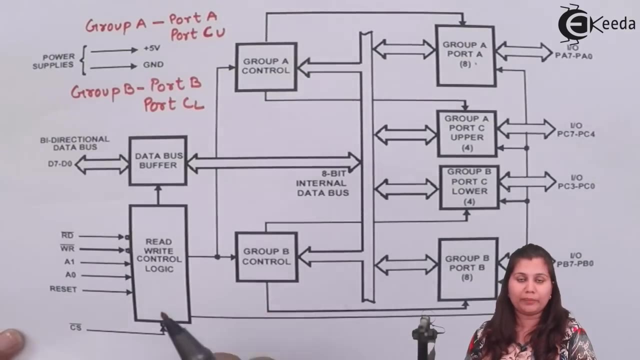 buffer and this data bus is bi-directional, from d- naught to d7. then we have read write control logic. and to this, read write control logic, we have the various signals which decide that, whether the operation, it is a read operation or it's a write operation, we have the signals: read write a1, a naught. 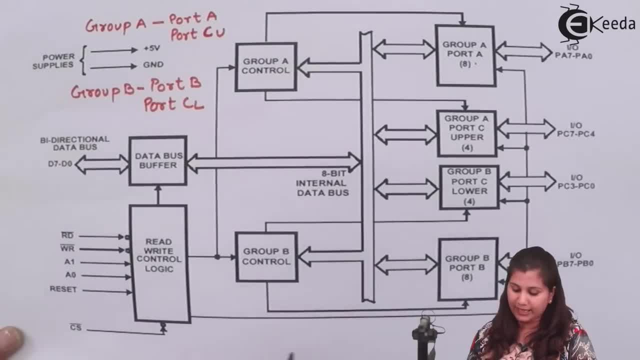 which will decide that which port is going to be selected. then we have the reset uh signal here, reset pin, which is going to clear the control register. then we have the chip select signal here, which is uh, will decide that when, if it is low, then this 8255 chip will be selected. 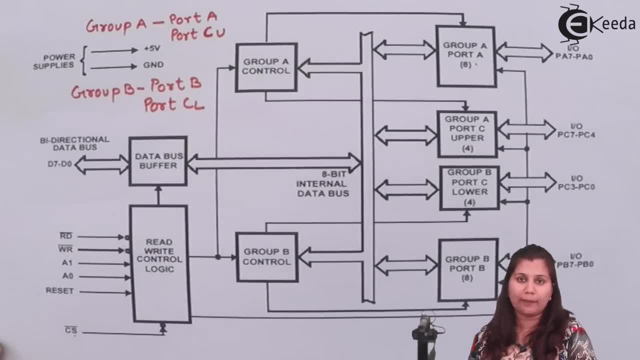 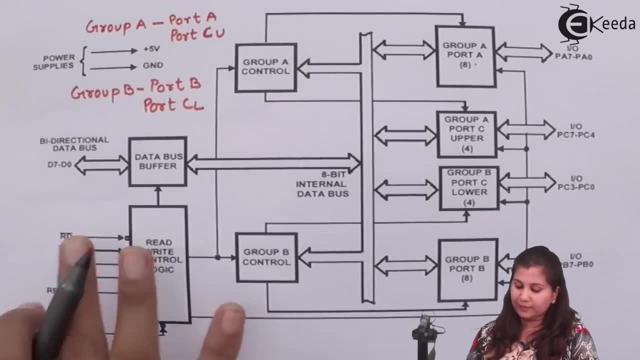 otherwise it will not be selected. it will not allow the communication between the central processing unit and between the data bus. okay, so this is the block diagram representing all the blocks, or all the controls components of 8255. now let us study each of these blocks, each of these components, one by one. 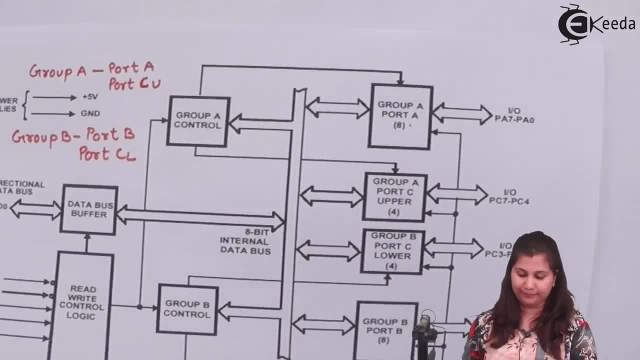 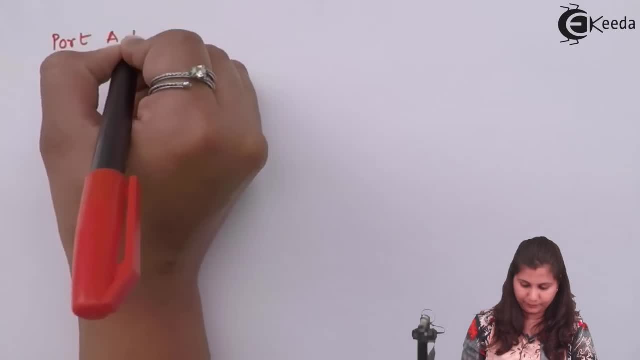 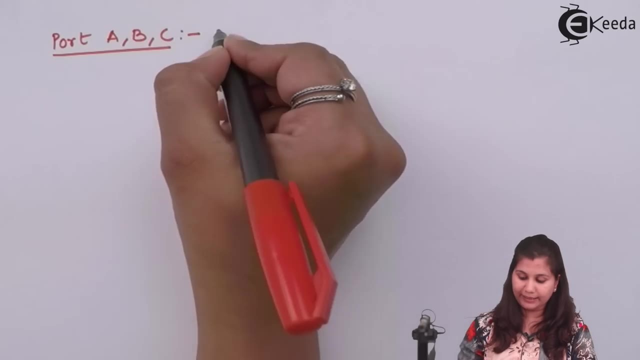 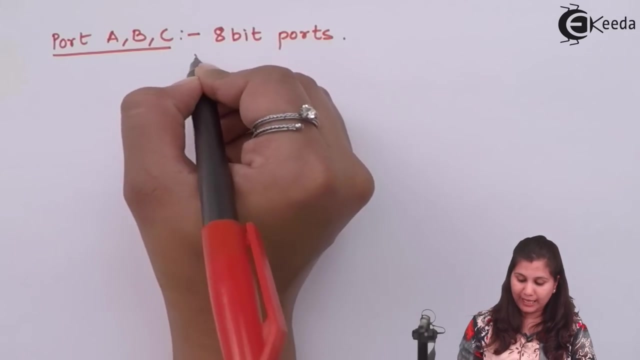 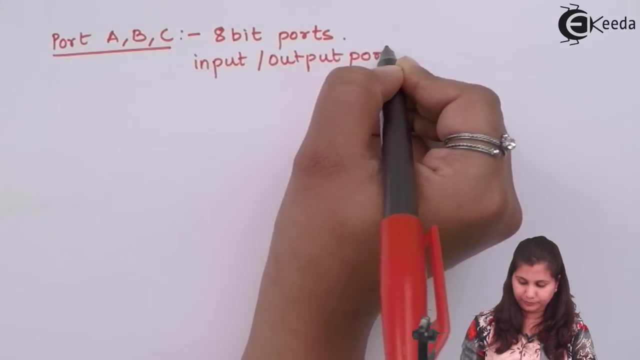 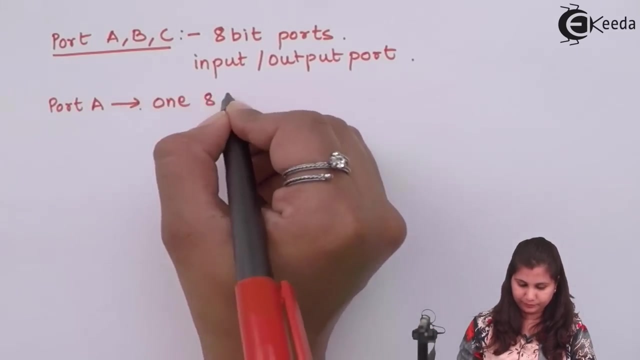 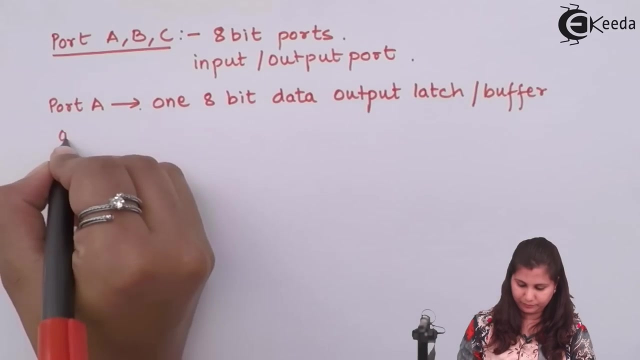 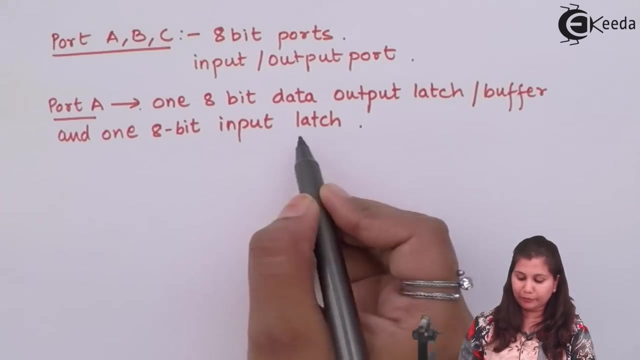 we will start with the ports a, b and c, as we have studied earlier that these ports are eight bit in ports and they can be used as either input port or output port. first we will have port a. this port a is having one 8 bit data output latch or buffer, and one 8 bit input latch. okay so, input. 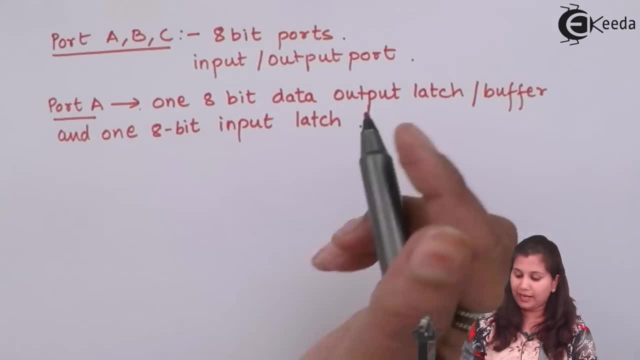 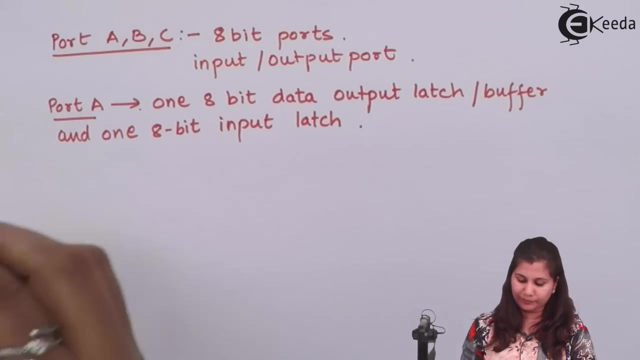 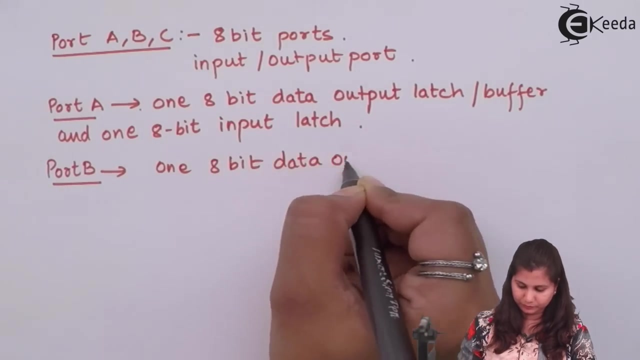 latch: it is providing the input data and output latch: it is providing the output data. so when the port it is acting as an output port, this latch will work, and when this port is acting as an input port, then this input latch. is this going to work? then we have port b. 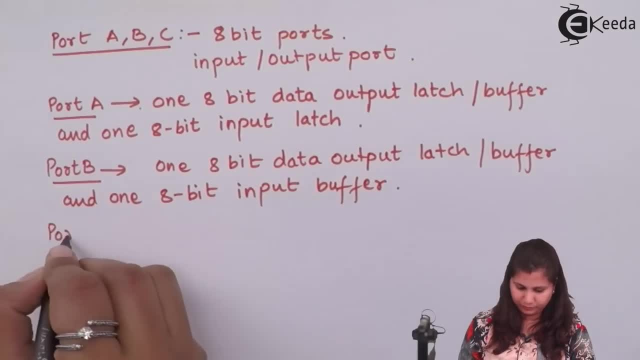 port b also have one 8-bit data output latch which will be used when the circuit blackheadS express is operating. so come surely use this port. if you want to use the port b also, you need to be careful about another one like this. port b is acting as an input port, then this input latch is. we are going to work. then we have port b. 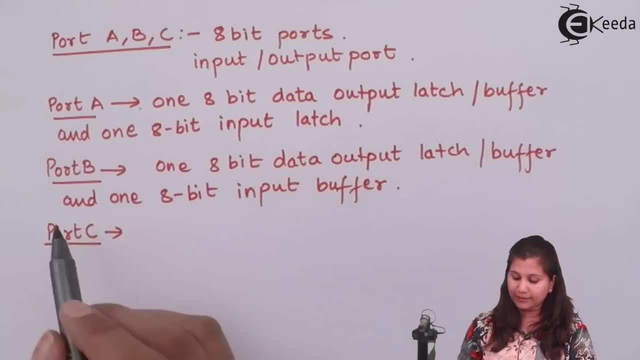 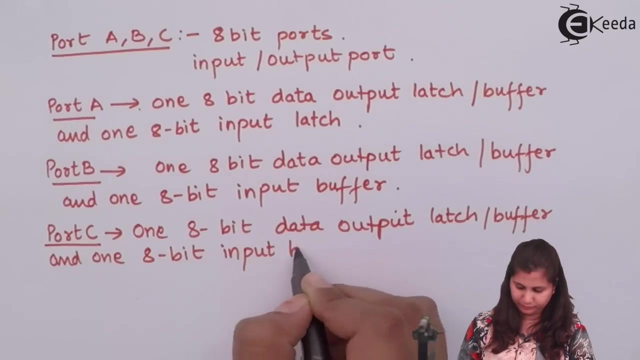 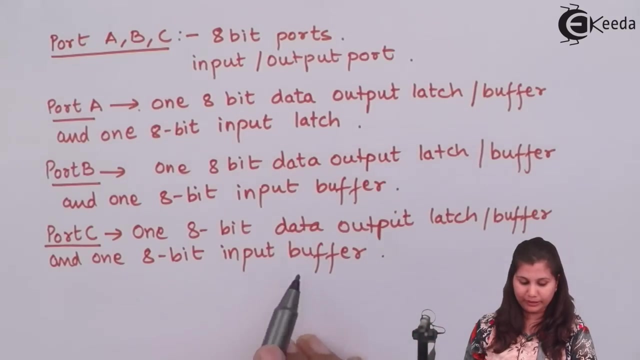 used when the port will act as an output port, and one 8-bit input buffer, which will be active when the port will act as an input port. Similarly, we have port C. Port C also have one 8-bit data output latch and buffer and one 8-bit input buffer. 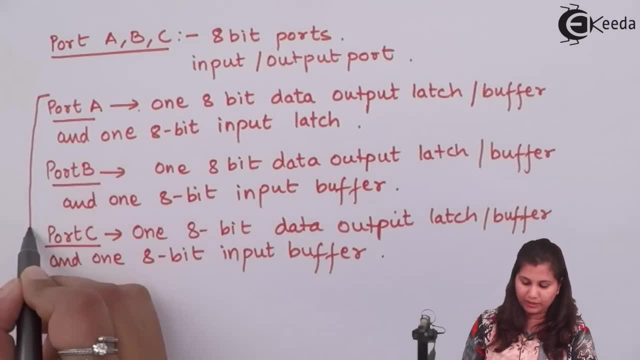 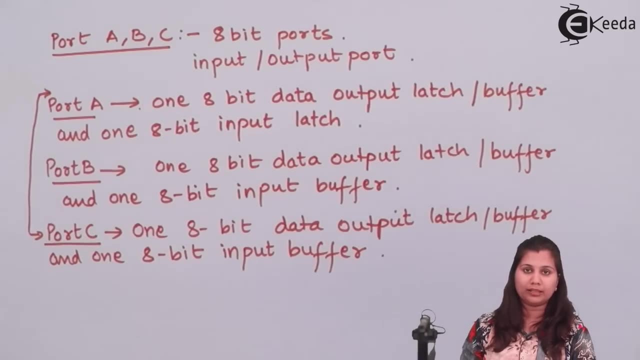 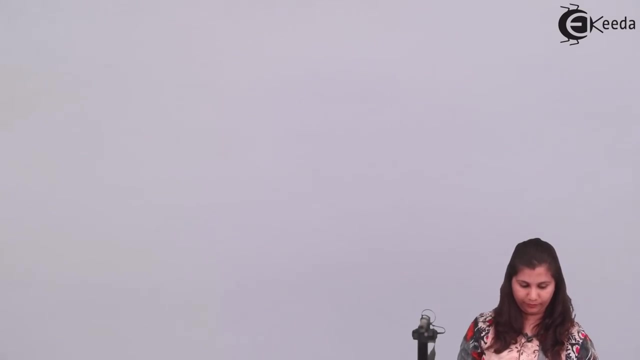 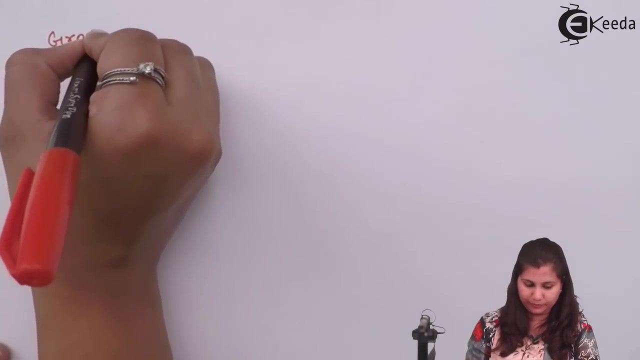 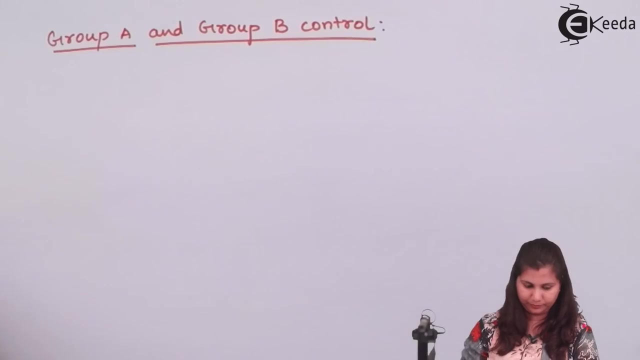 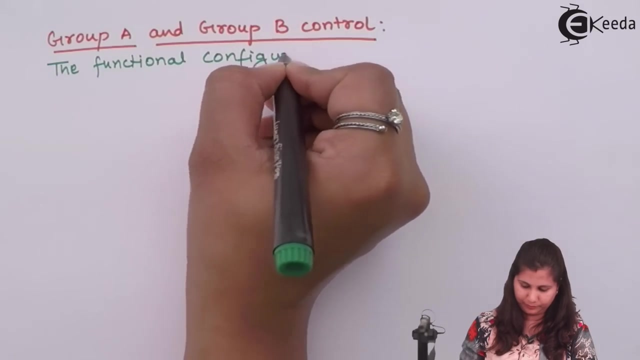 Okay, so these three ports are available in the 8255 and for each port we have an output latch and an input latch. Okay now. next, we have the group A and group B control. So let's see what we had in the group A and group B control. 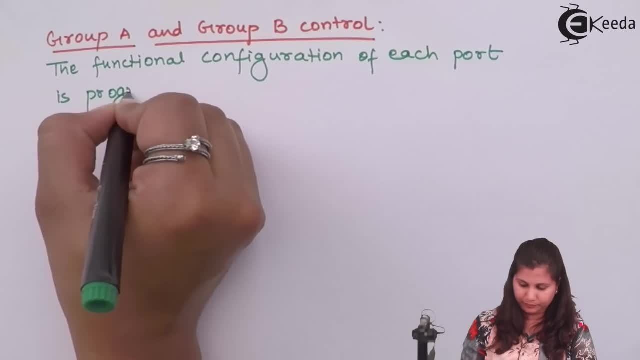 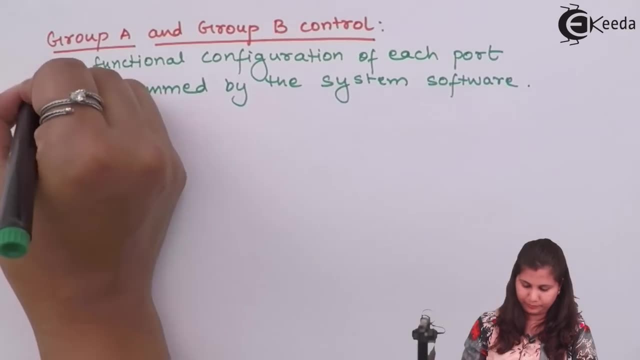 So we had the group B control and we have the group A control for each port And, as you can see, we have a similar setup for the group C control and for this group C control. So we have a shared operating system in the group B control. 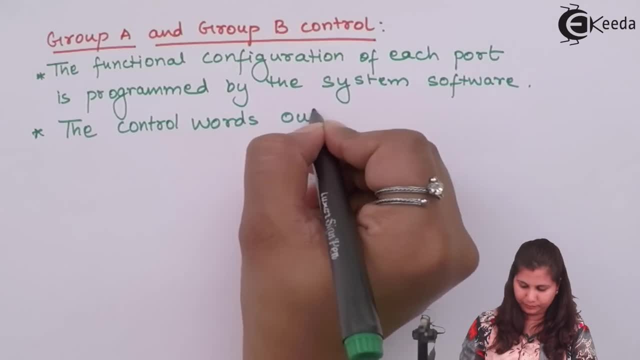 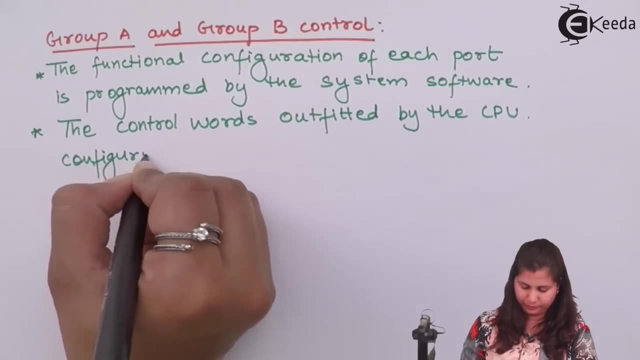 We have two different control systems and we would be 해тер, So this would be our control system. Here is the control system where we would be having to create an operating system, And this would be a control system that our device would be operating on. 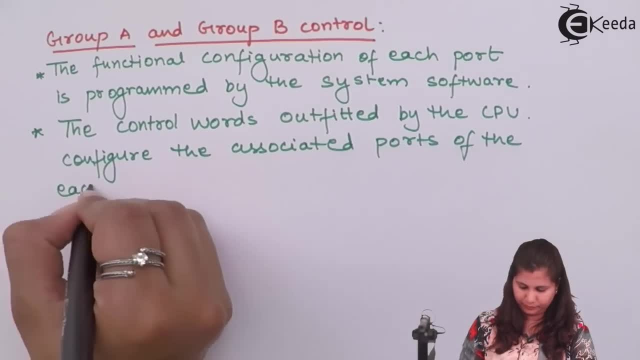 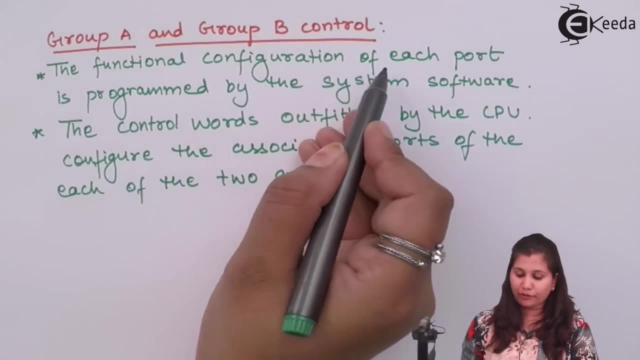 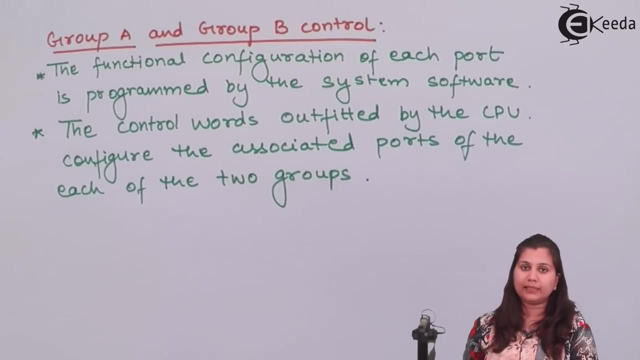 Okay, so the functional configuration of each port. it is programmed by the system software. we have three ports and each of the port can act as an input port and output port. so this function, that whether the port will act as an input or output, it is defined, it is decided by the control word, which. 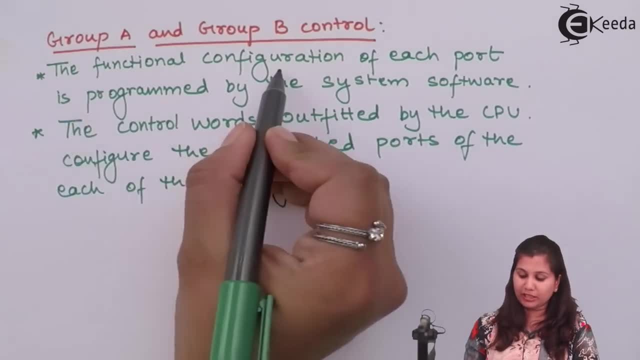 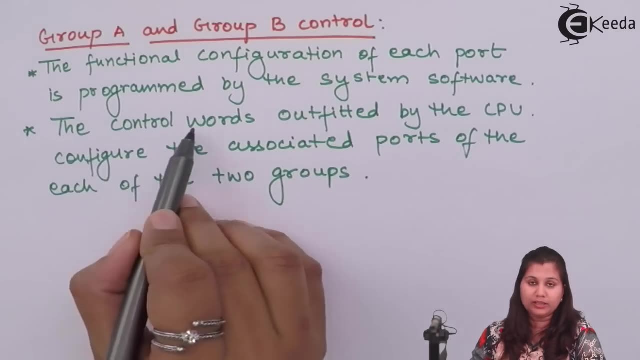 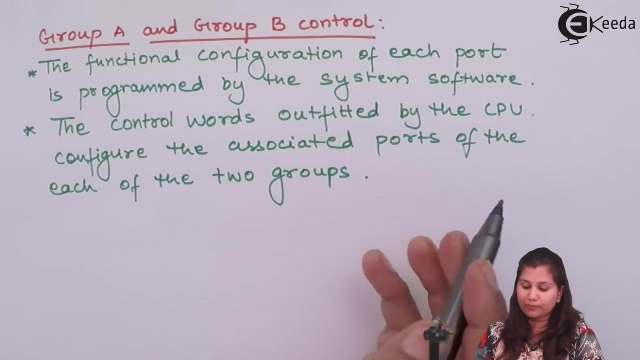 is written in the control register, so the functional configuration of each port. it is programmed by the system software. so the control word which is written in the control register, it is given by the CPU. it configures the associated ports of each of the two groups, because we have 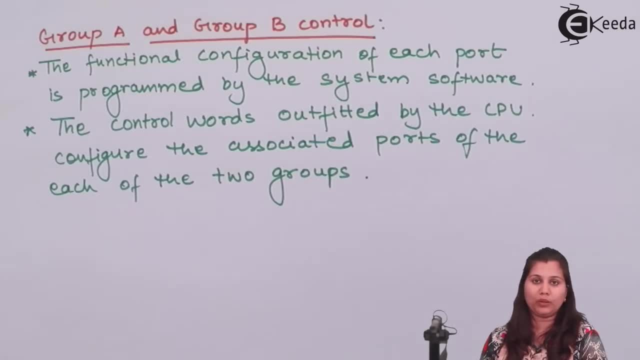 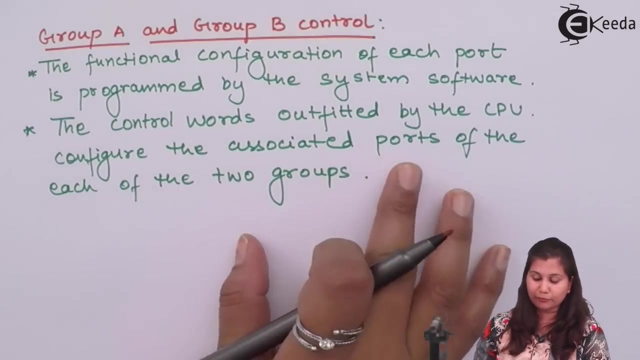 group a and group B. group B is having the port a and the port C upper. so the control word which is written in the control register that will decide that which group is going to be active. okay, so the control word it is which is outputted by the CPU, it will configure the associated ports. okay, and which information? 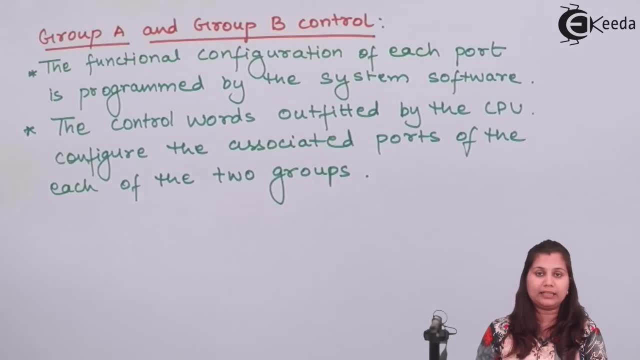 the information which is carried by the control word. it contains the mode, set, reset bits and which mode is going to be selected and which data bit is, which port will act as an input, which is going to be acted output and which group is going to be active. all the information it is contained in the control. 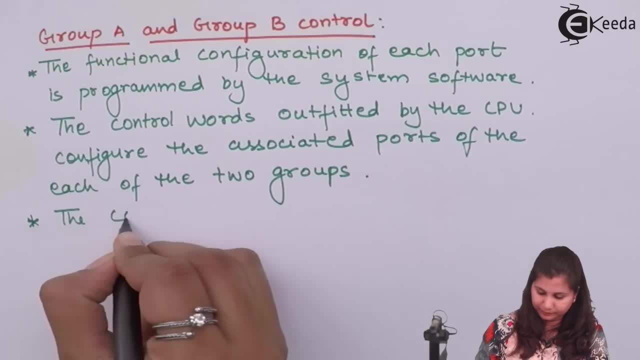 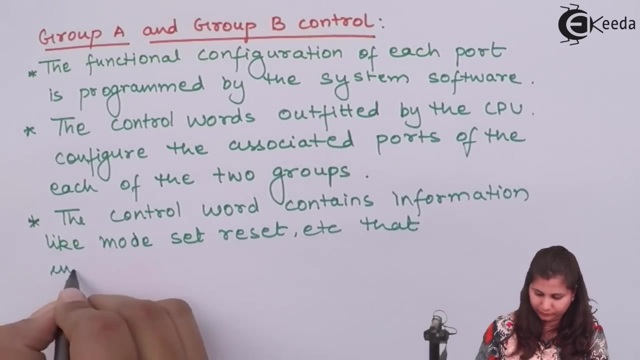 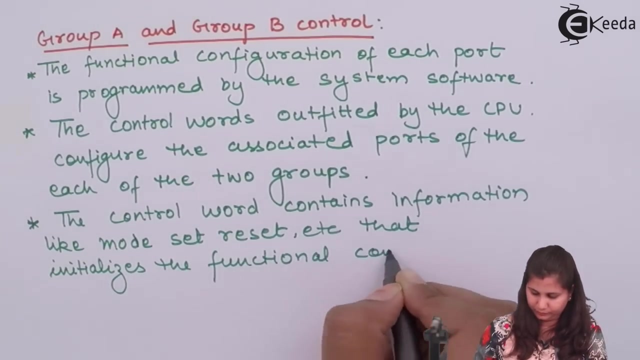 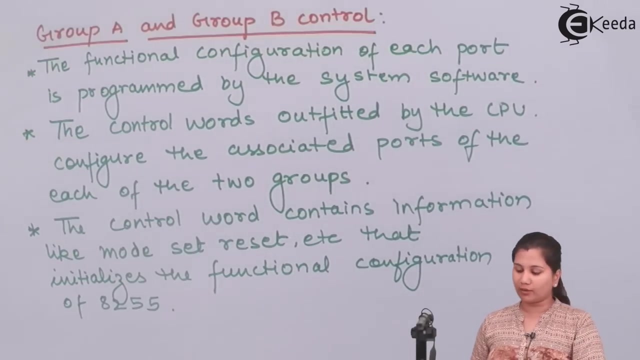 world. so the control word, it contains all the important information like the mode set, reset, then this information, it initializes the functional configuration. or we can say that this control word decides that the ports of the 8255, they will work in which of the modes. now, this control word, 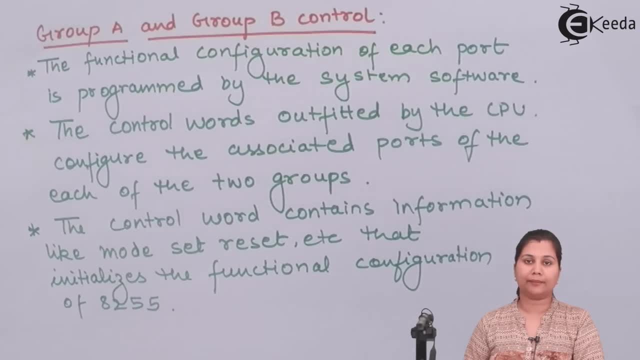 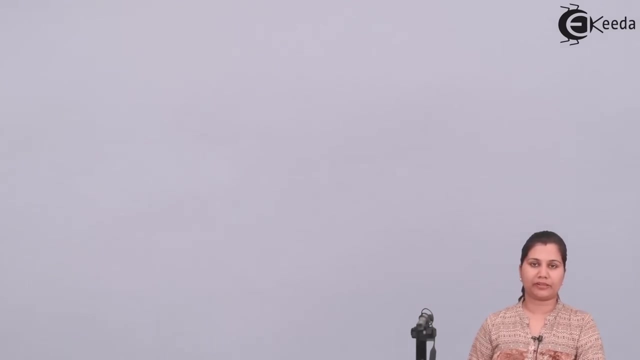 it is provided by the CPU of the microprocessor and the CPU is going to write this control word into the control register. so for the control register we have the right signal and the control register. it cannot be read by the microprocessor, so it has only the right signal associated with it. 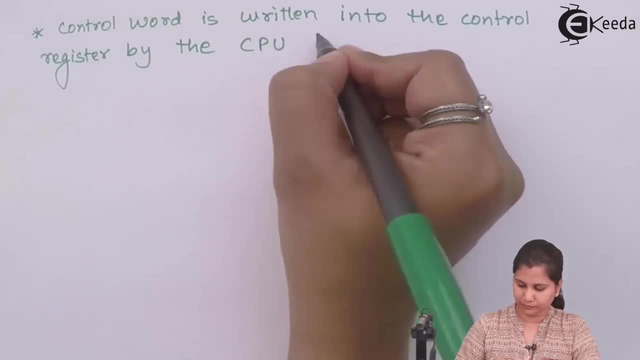 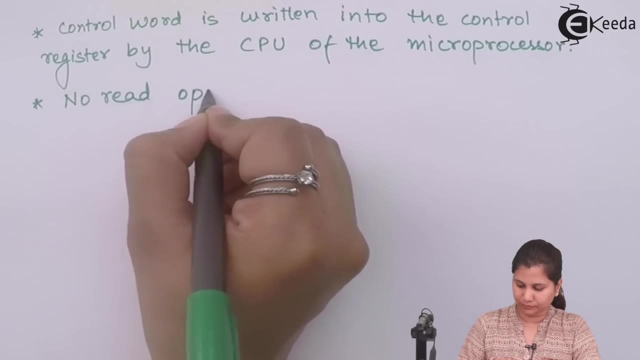 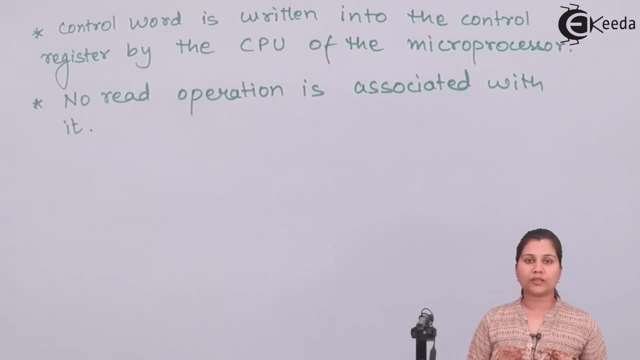 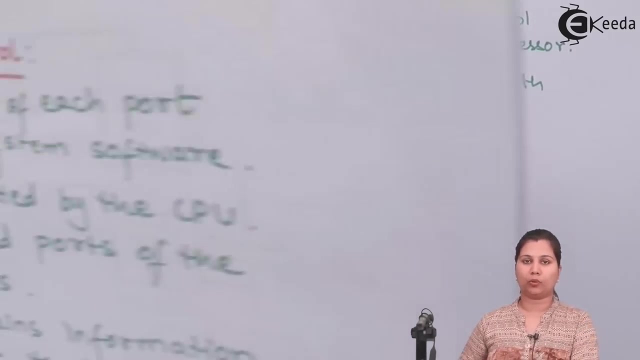 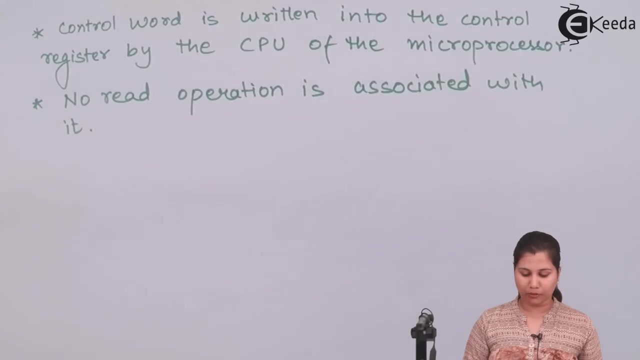 she needed a pulled back. so this was about the эта and group be controlled to. a was having the port and port c output, and group be contains the part b and port cm now comes in the block diagram. we have the next block, that is, the data bus buffer and the 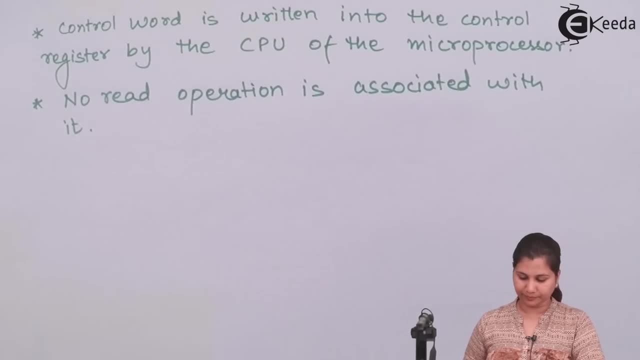 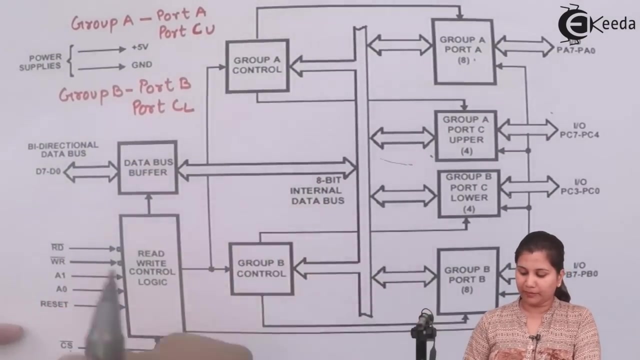 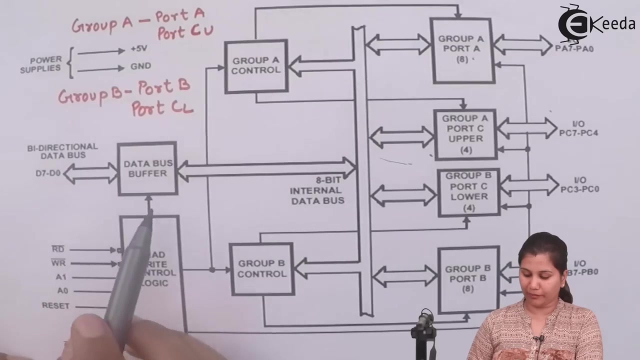 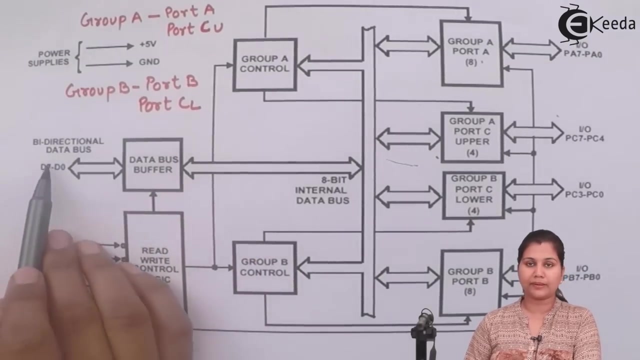 bi-directional data bus, the 8255. it is having the internal 8-bit data buses also there and with this internal data bus it has the data bus buffer. now, this data bus buffer, it is an 8-bit bi-directional buffer and it is a tri-state 8-bit buffer which is used to communicate with the data bus. 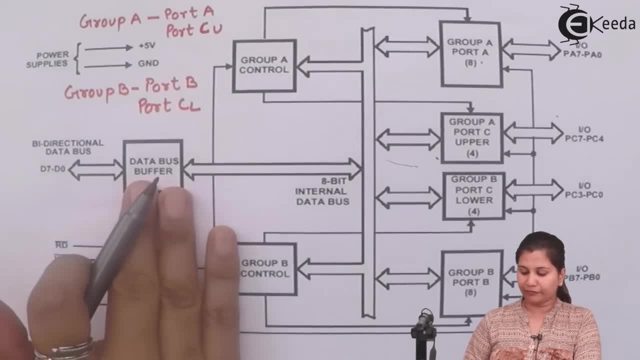 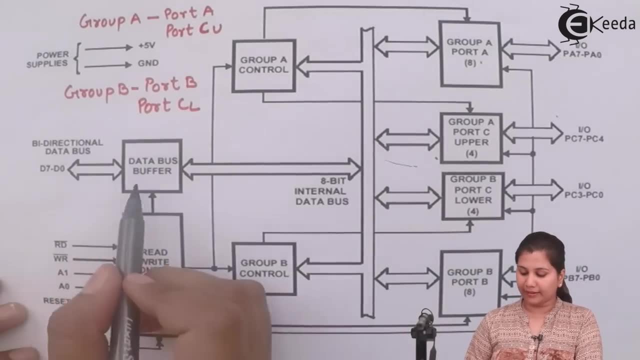 of the microprocessor. so whatever data, if the data is to be written into the ports a, b and c or in the control register, then that data is provided by the cpu of the microprocessor into the data bus bus buffer. and when the data is read from the ports A, B, C, then that data is also. 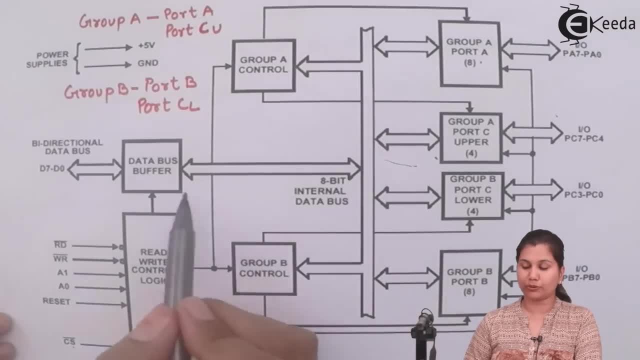 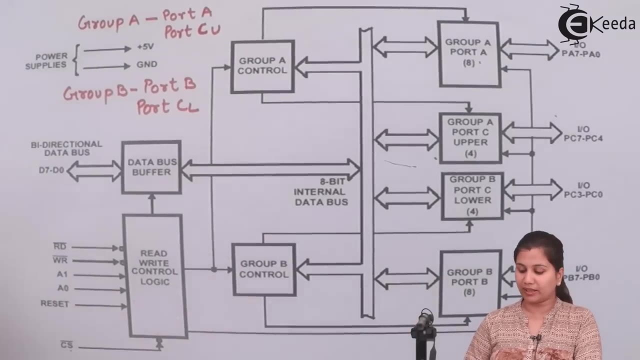 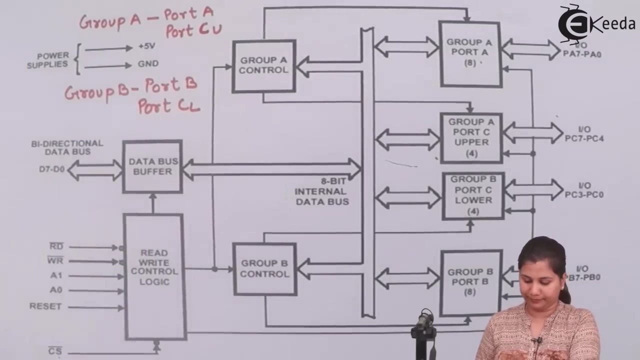 transferred through the internal data bus on to the data bus buffer. so the work of this data bus buffer is to communicate with the central processing unit of the microprocessor and also with the 8255. so it's a communication link which is transferring the data between the 8255 and the microprocessor. so we 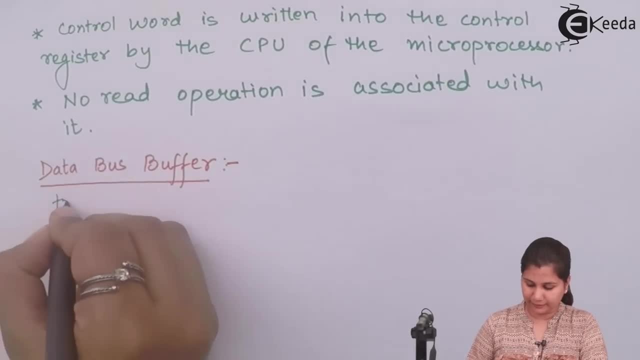 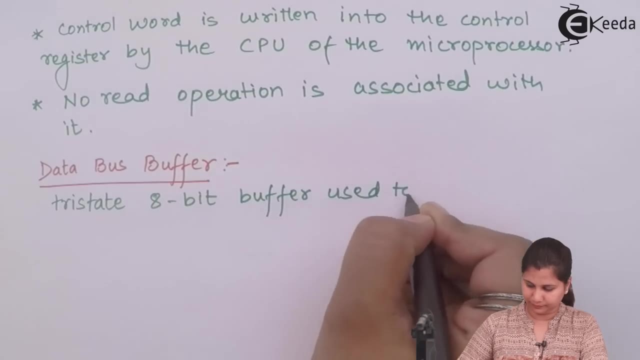 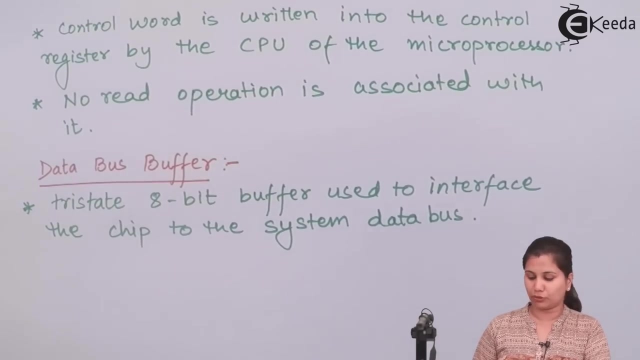 can say that the data bus buffer it is a tri-state. it is a tri-state 8255 buffer because data buses of 8 bits, so the buffer has to be of 8 bits. so it's a tri-state 8 bit buffer which is used to interface the chip to the system data. 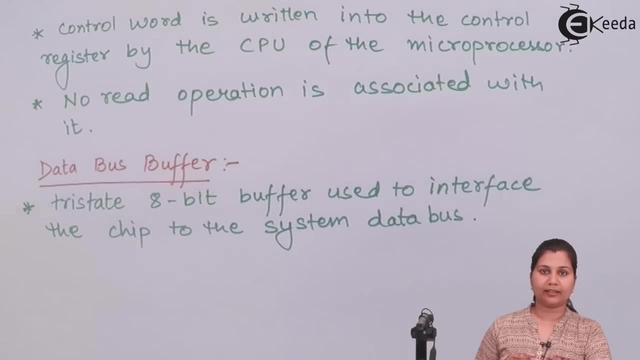 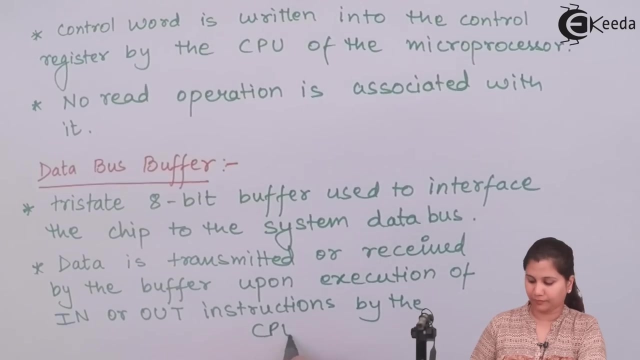 bus interface. it is a communication link between two components. so we can say that the data bus buffer, it is acting as an interface between the chip, that is the 8255, and the system data bus, that is the data bus of the microprocessor. now, as this data bus buffer it is, 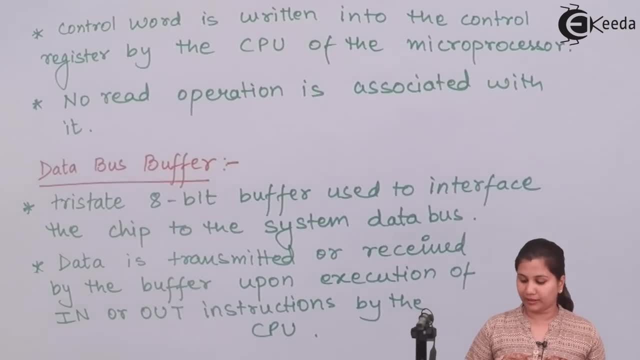 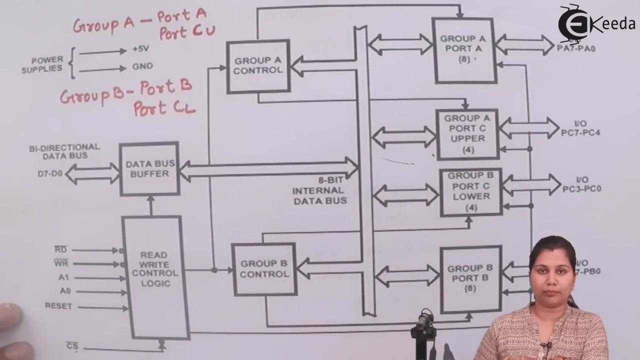 transmitting or receiving the data. so this data is transmitted or receive the When the instruction- in and out- are executed by the CPU of the microprocessor. Now this data bus buffer, it will read the data from which is on the ports. If this read signal, it is low and the instruction in is 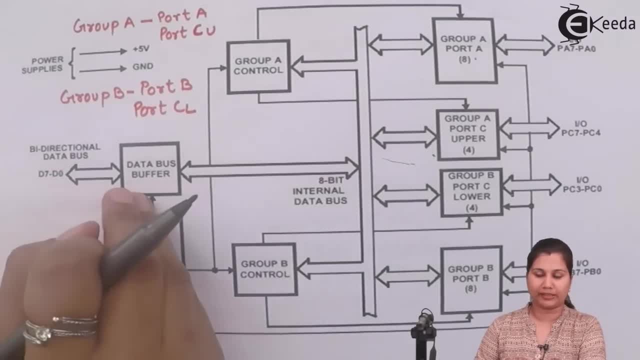 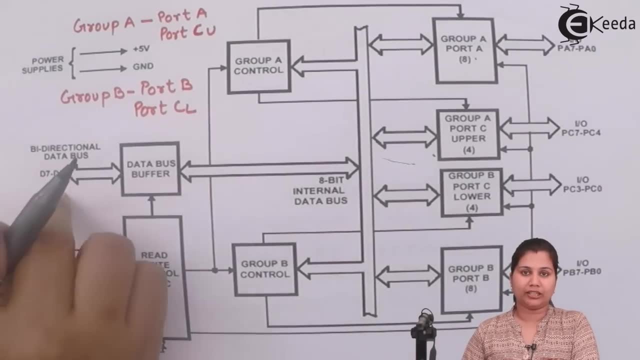 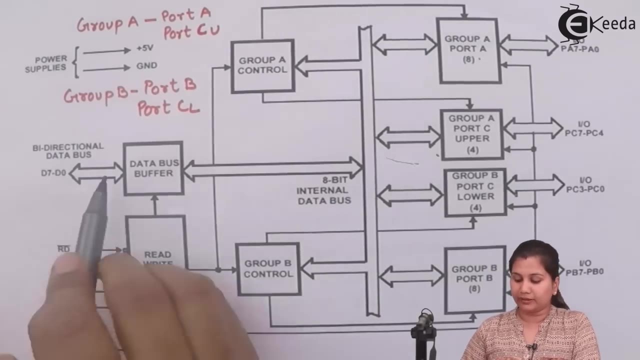 given by the central processing unit of the microprocessor. So in instruction it is going to read the data from the ports and if the CPU has given the instructor or it has executed the instruction out and this write signal, it is low then the data which is available on the data bus. 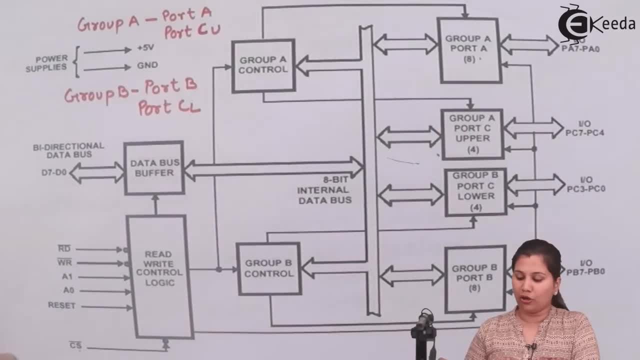 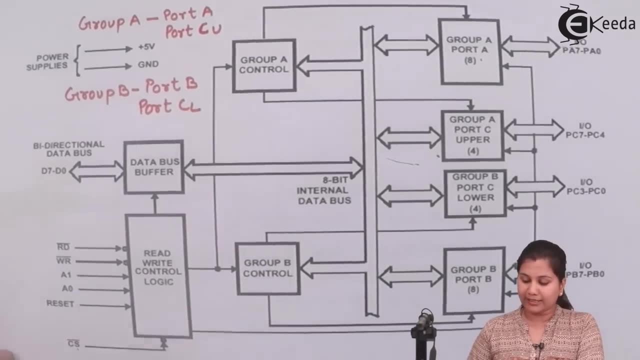 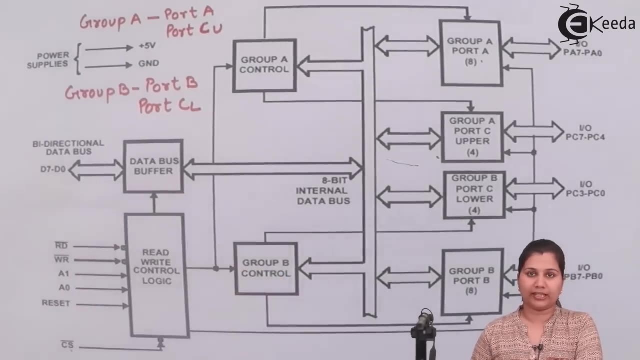 buffer, it will be written on the ports A, B and C, or if it is the control word, then the control word will be written in the control register. So that is the function of the data bus: that the data is transmitted or received when the instructions in and out are executed and when the signals read. 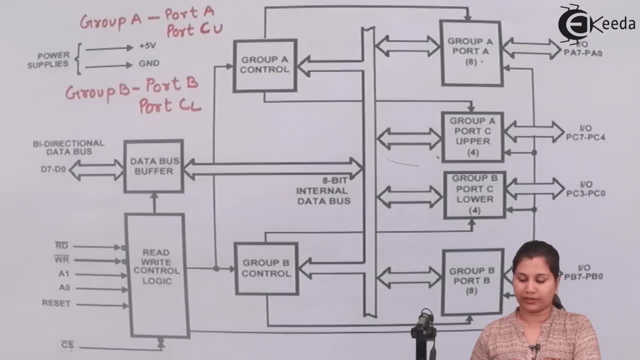 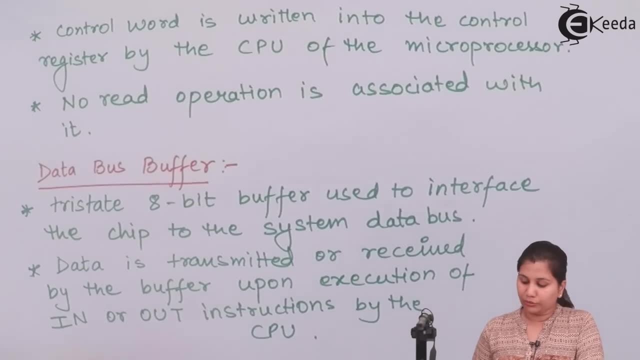 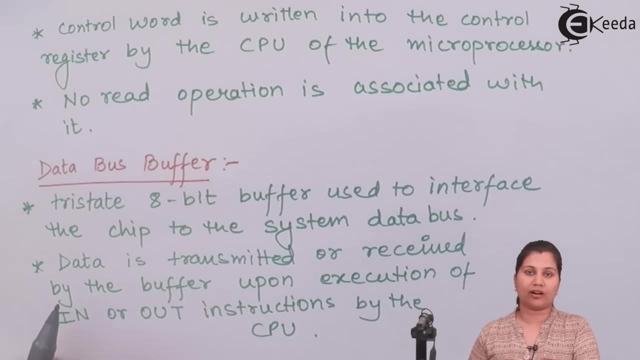 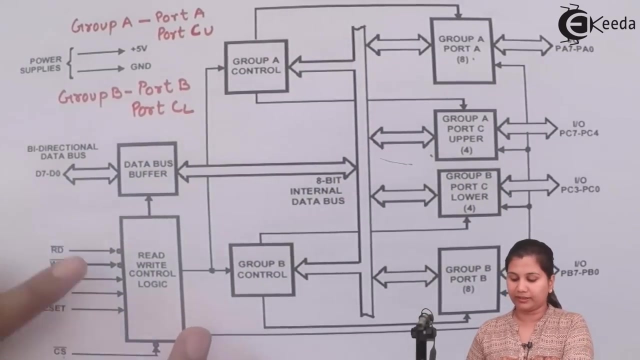 and write are at their uppercase, Not only the data which is transmitted or received by the buffer, the control word is also and the status words. they are also sent out by the data bus buffer. If the control register is selected, then the data bus buffer, the data which is provided by the CPU of the microprocessor. 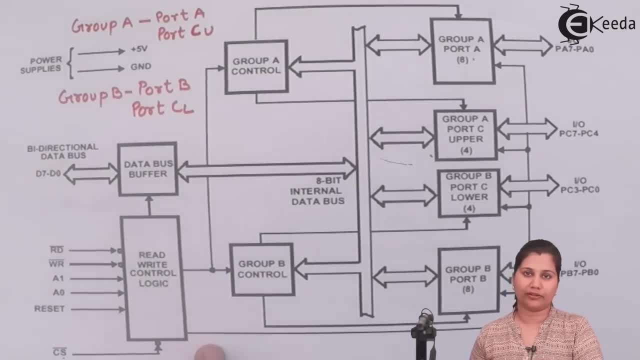 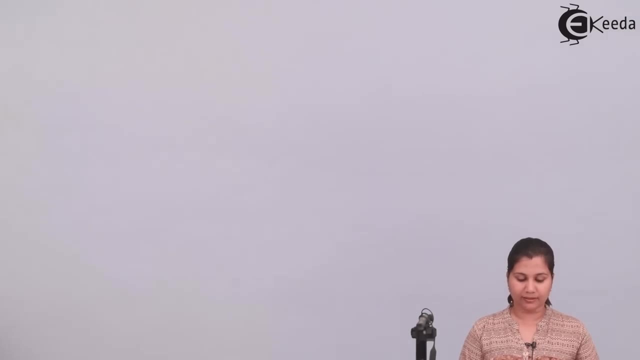 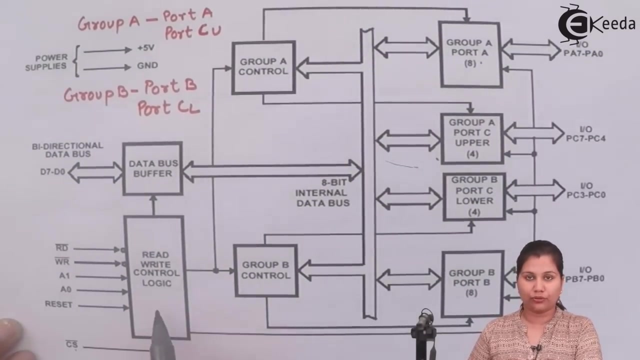 that control word will be written in the control register. So the data and the control and the status information, all such type of information. they are transmitted or received by the data bus buffer. Now, next in the block diagram comes the read and write control logic. Now this read and write control. 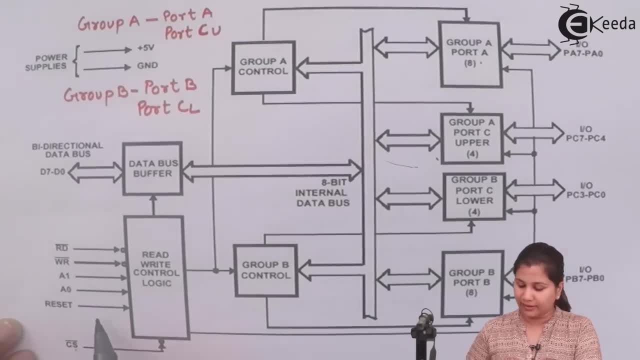 logic it is having these five signals: read, write- A1, A0, reset and chip select. We have already studied these signals. that what is the function of these signals? Read signal: it is used to read the data from the ports. Write is used to write the control word or write the data onto the ports. 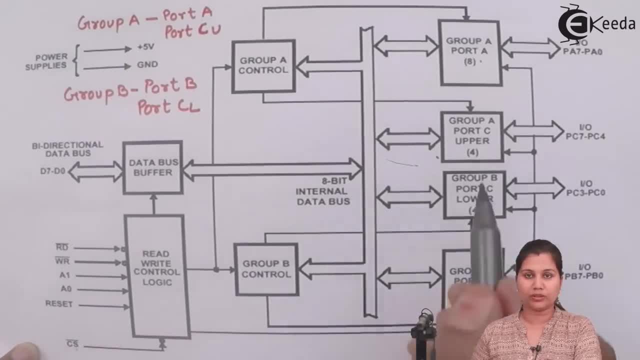 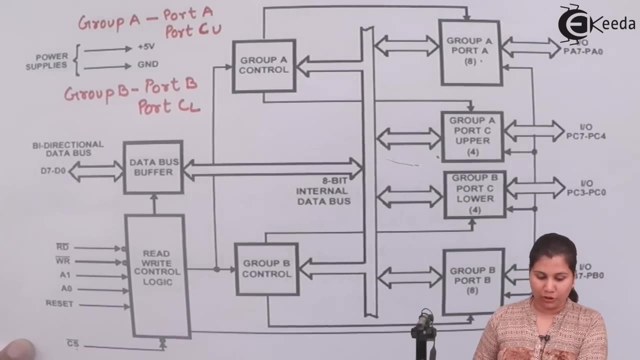 Then A1 and A0. they are used to select the port, that is, the port addresses. they are decided by A1 and A0 and reset is used to clear all the ports and chip the select this signal. it is used to select A2, A5.. So this read and write control logic. its function is to control all the functions which are: 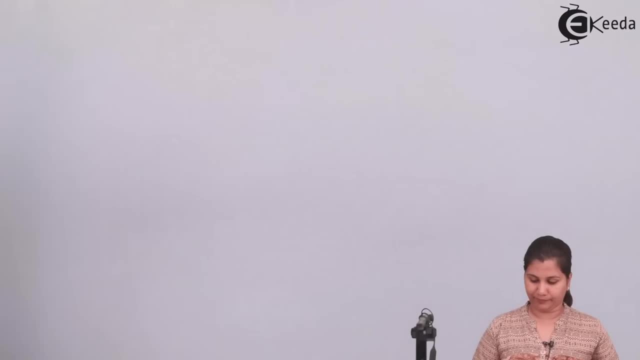 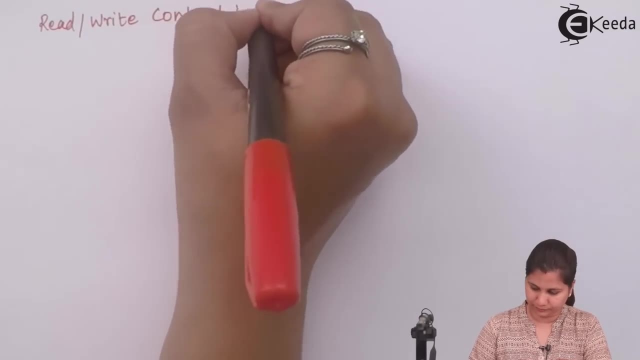 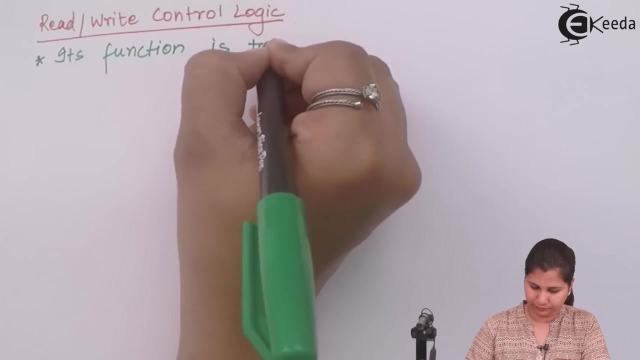 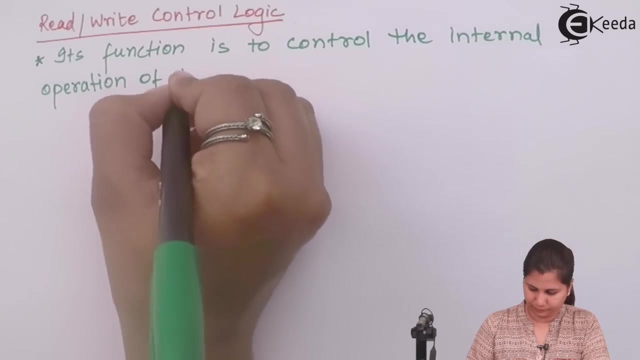 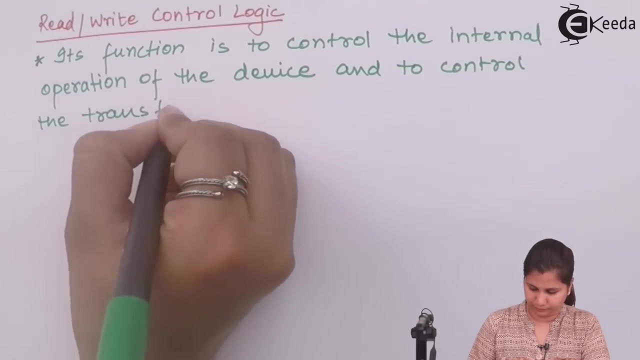 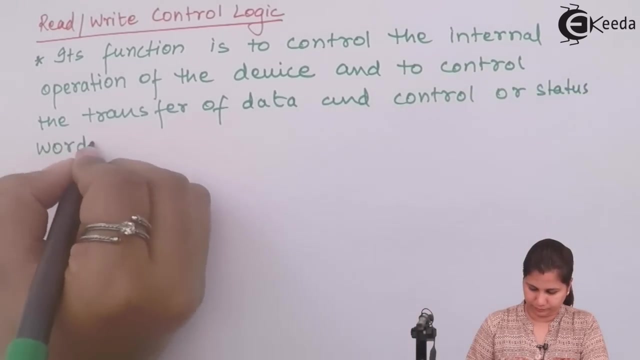 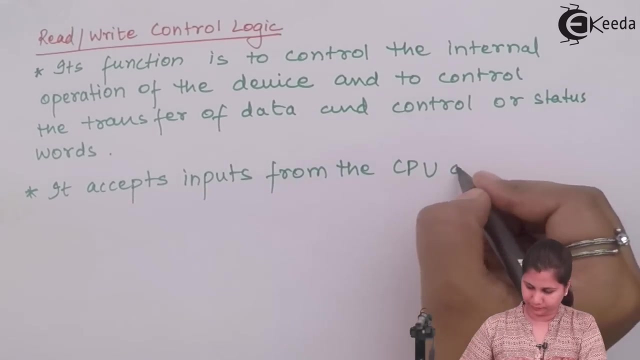 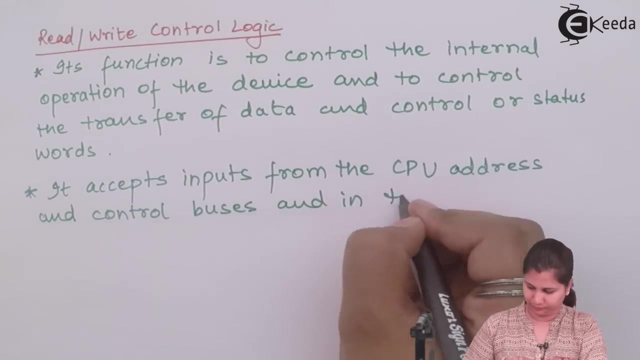 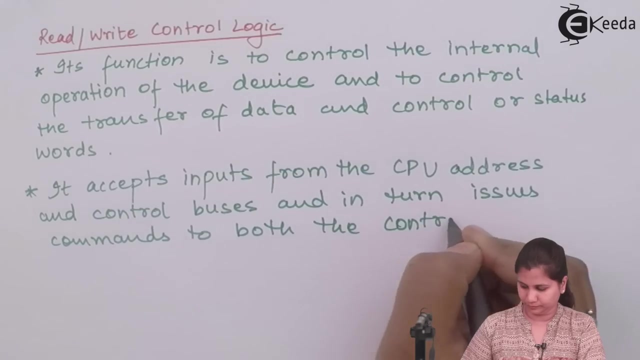 performed by the chip A2, A5.. When you look at this sequence, the Tout上面, both of these signals are using the same function- A1, A2- you can find out that both of it E2, e2, e3. so the function of this read and write control logic it is to control the internal operation. 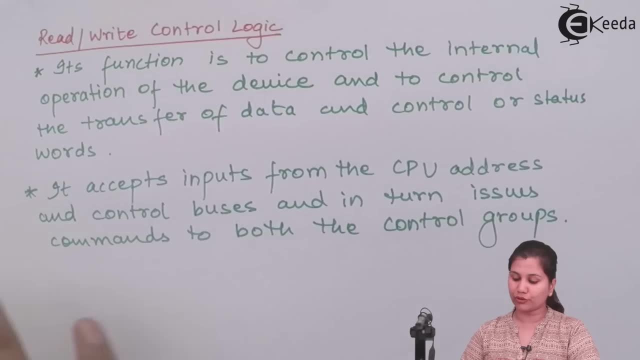 of the device that is the 8255, and to control the transfer of data and control or status word. so whatever data it is read or written that is read from the ports and written into the ports and the control register, all those information it is controlled by the read and. 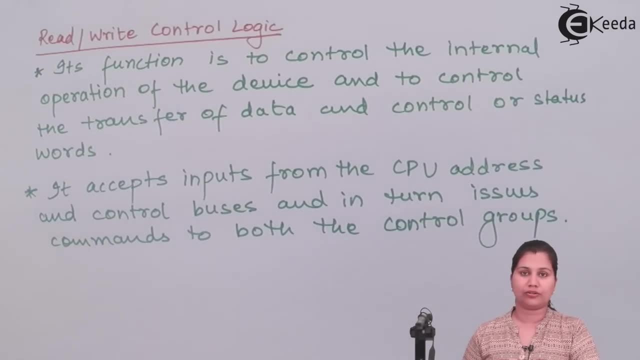 write control logic. now this read and write control logic. it accepts the inputs from the cpu address and the control buses. the address of the ports it is getting from the address bus of the cpu of microprocessor and control buses. from the control buses it is getting the control. 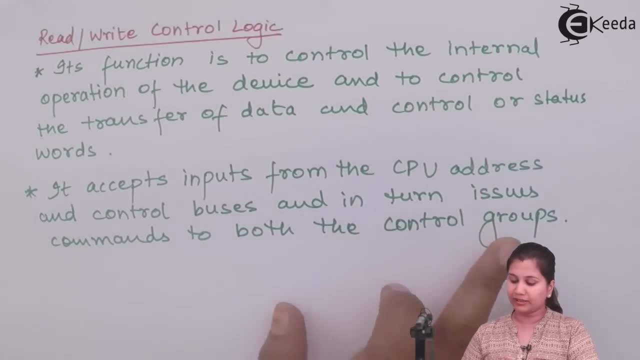 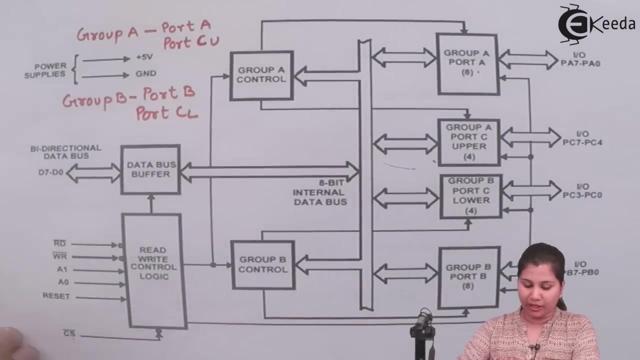 signals, read and write, and in turn it is issuing the command to both the control groups: group a, control and group b, control. okay, so that is the function of all the blocks of this block diagram of 8255. we know that this power supply, it is provided by the 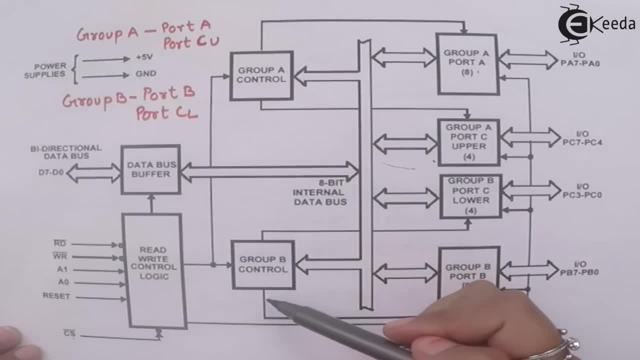 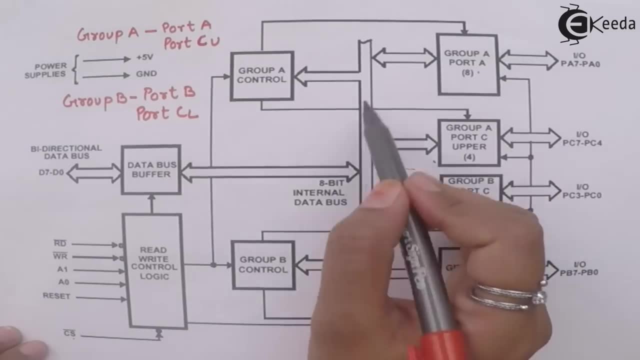 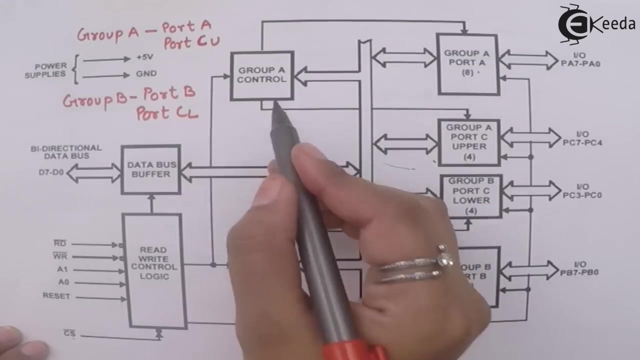 plus five volts and ground. then we have the group a control, group b control. group a control is having port a and the port c upper. these are the internal data buses which are transferring the data to the all the blocks and the single lines. they are showing the control signals which are 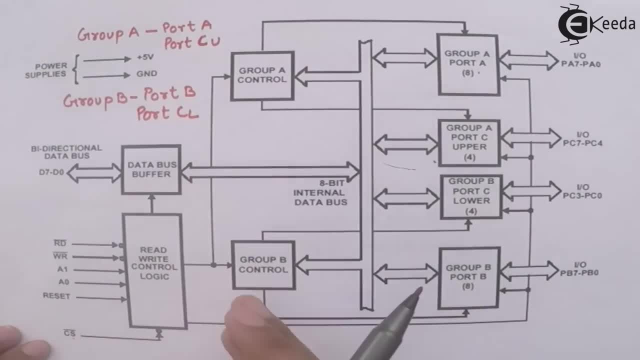 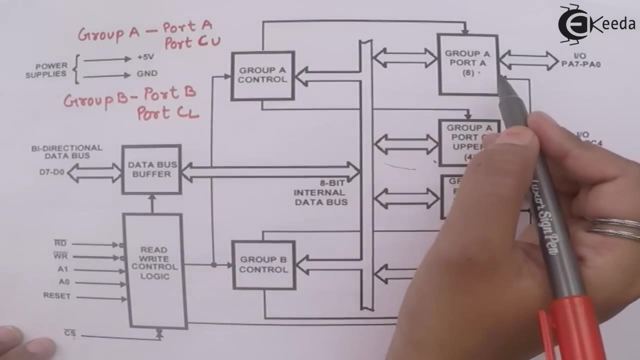 given to all the ports and the group a control and group b control the bi-directional buses they are showing. these are the internal data buses and the single lines. these are the internal control bus. okay, control signals are transmitted through these. now, these groups, the ports, they can act as an. 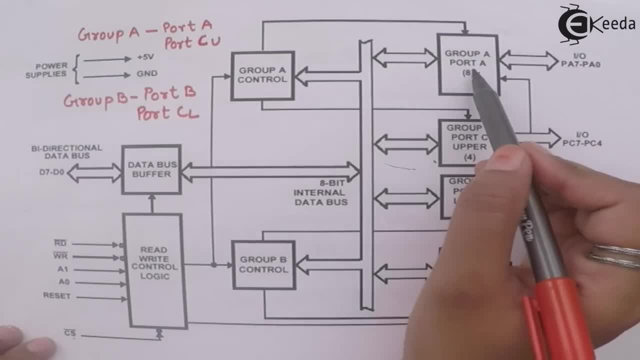 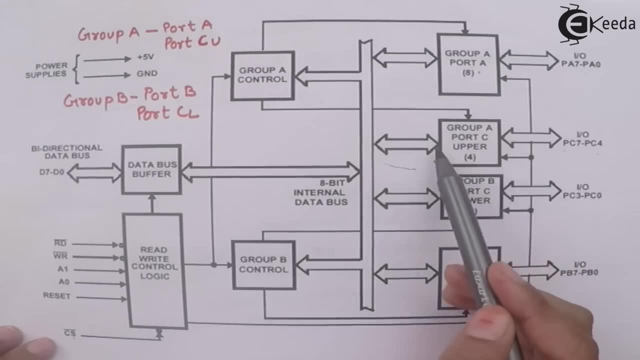 input output ports. so they have the pins because they are eight bit ports. so they have the pins: pa7 to pa0, like pa, pc7, pc4, because it is port c upper, then port c lower, pc0, pc3 and port b, pb7 to pb0 and all these 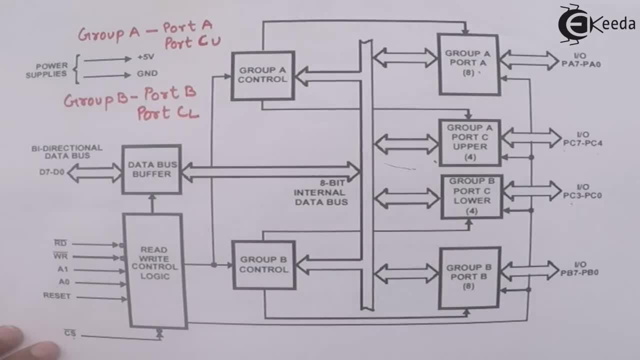 four ports. they can act as an input output ports. then we have the data bus buffer, which is connected to the bi-directional data bus of the microprocessor and read and write control logic. it is providing the control signals to the group a control and group b control. so this is the block. 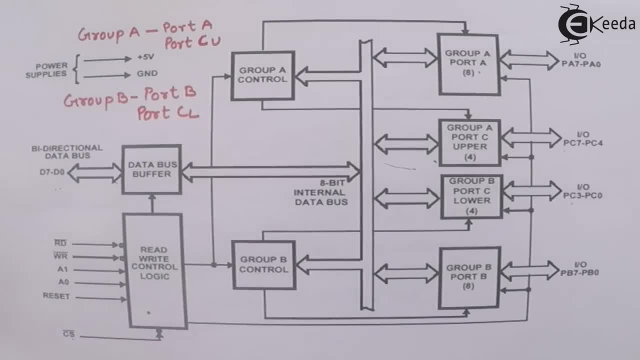 diagram of 8255. so in this video we studied about the programmable peripheral interface 8255. this 8255, it is acting as a peripheral device which is connected, which is acting as an interface between the microprocessor and some of the input output devices. 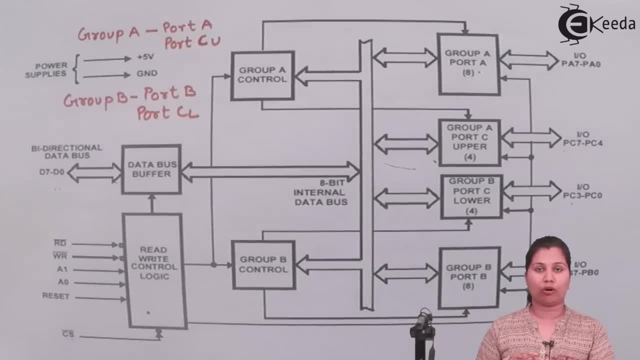 so whenever microprocessor it is connected with an uh it wants to communicate with an input output device, then this 8255 it is connected in between it, so it is acting as a programmable peripheral interface. okay, so we studied the features of 8255 that it's a 40 pin ic then 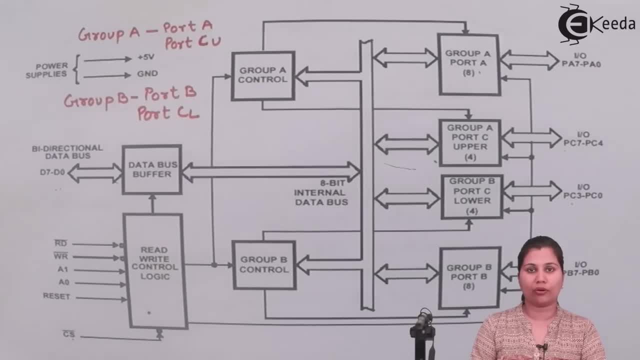 we studied the pin diagram, the description of all the pins of 8255, and in the last we the block diagram of 8255 describing the functions of all the blocks of the programmable peripheral interface. So I hope that this topic is clear to you. Thank you.